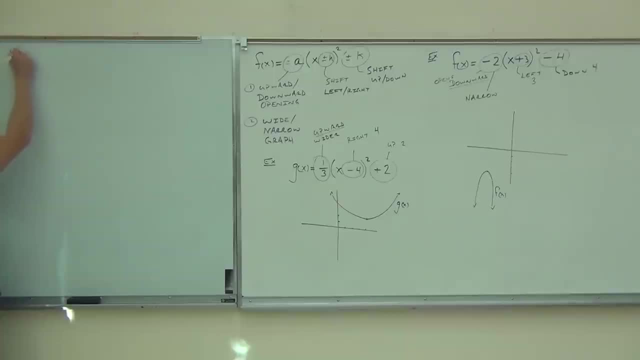 So in 11.6, you're going to get a little bit more on graphing, More on graphing. Don't worry, we're not graphing morons. That's the 13th time I've used that joke, actually Isn't. 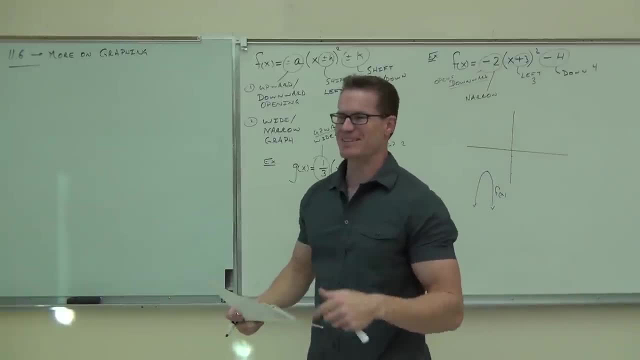 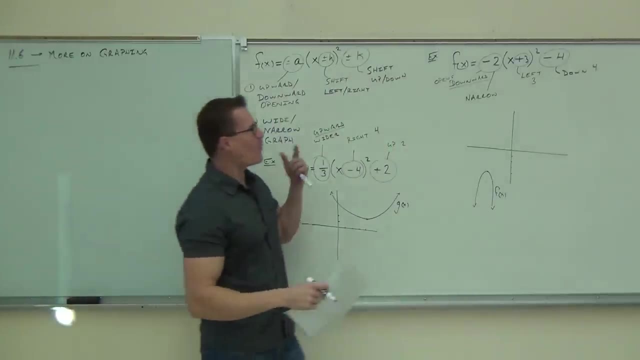 that pretty bad, Starting to even sound. no, it's still funny. I still like it. You see, the problem is is that we don't always get things that look like that, We don't get things that look like this. This form isn't always what we have, and we'd have to do a lot of. 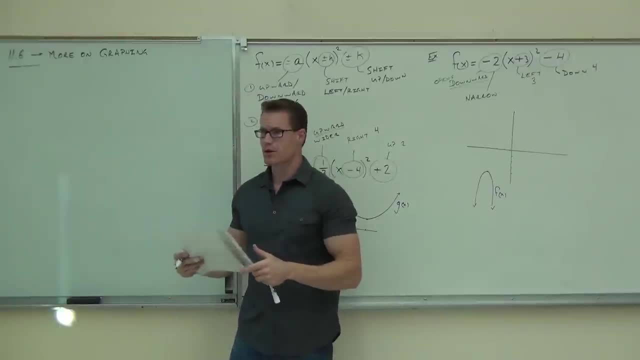 work to make it that way. We'd actually have to complete the square in order to get this thing and be able to factor in order to get that thing, And that's not exactly what we have all the time. We don't want to waste our time. 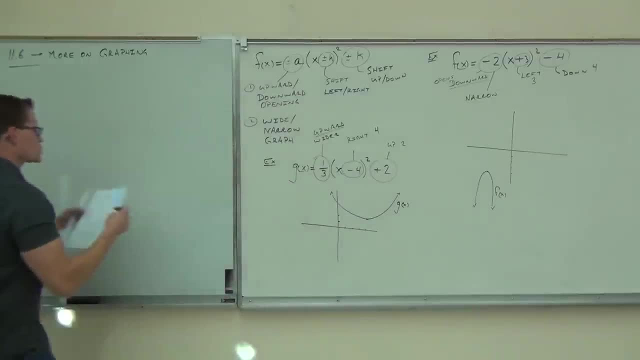 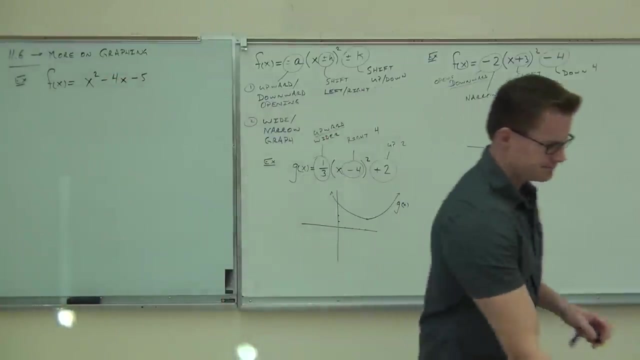 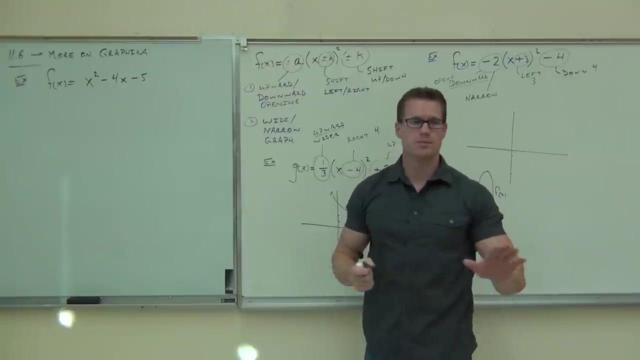 We don't want to waste our time doing that, So there are some other things that we can do with just our general quadratics, For instance, like this one: Hmm, Is that of this form? We could turn it into it. We're not going to. That'd be a lot. 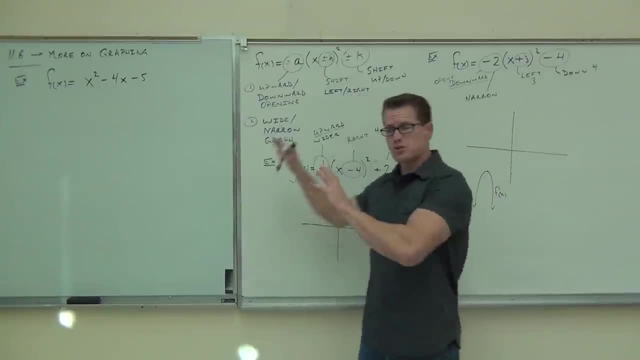 of work. We've got some better ways to do it, In fact, more precise ways to do it. This was curve sketching. This was great. This gives us an approximation of what our graph is going to look like, and a pretty 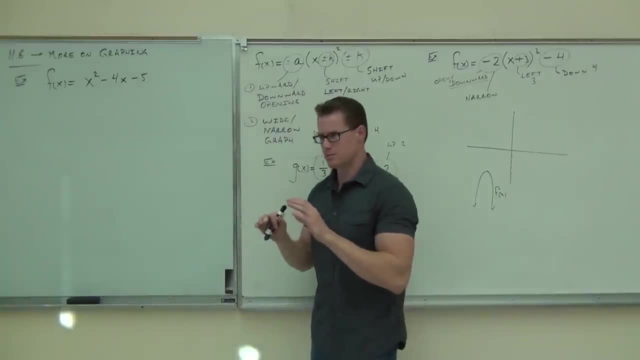 accurate approximation. What we're going to learn now is how to make it pretty precise without doing a table and without making points. Now, is it still a function? Is it still a quadratic function? What tells you it's a quadratic function? Good, What's your? 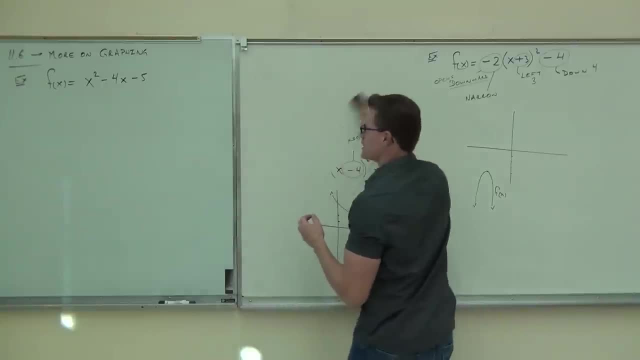 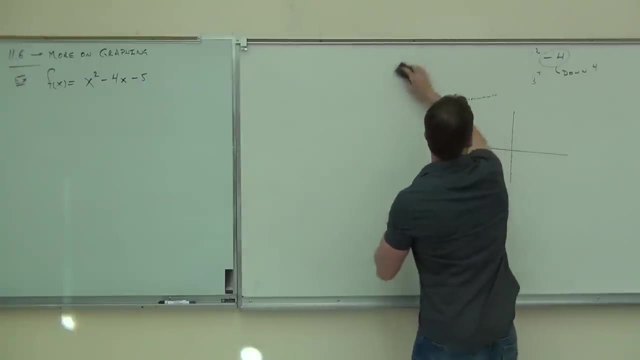 a here- Wait, wait, I'm sorry- Positive or negative one. So would you say it opens upward or downward? Upward, Upward's right, Exactly right. The problem is, you can't tell me whether this shifts up, down, left or right right. 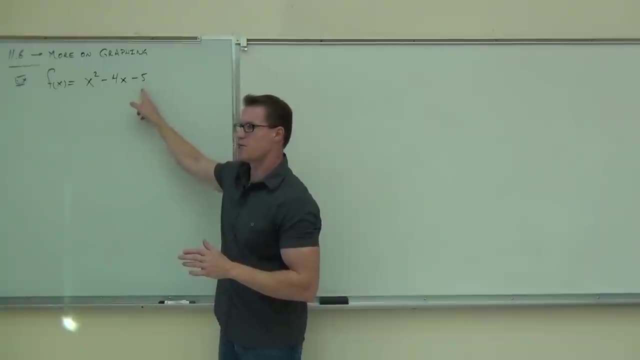 now because it's not in the proper form. This number would change if you had it in the proper form, but this number and this number do still tell us things. This right here tells us whether we're upward facing or downward facing, depending on whether you're. 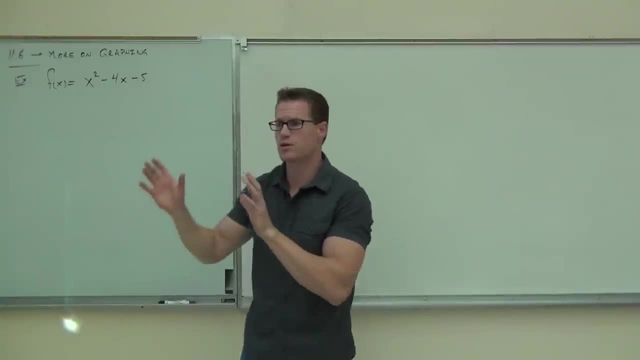 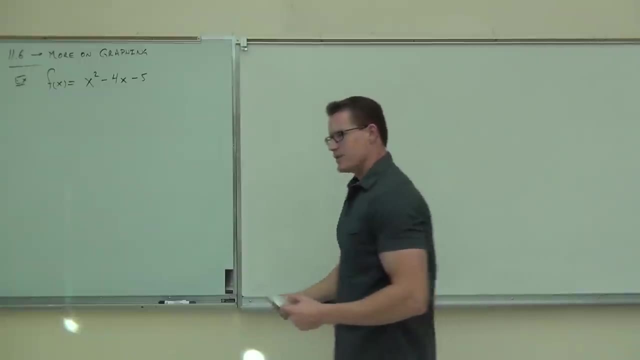 positive or negative. It tells you whether you're a wide graph or narrow graph, depending on whether you're above one or less than one. This also tells us something. We're going to come to that in just a moment. So I'm going to give you some steps. I'm going to give 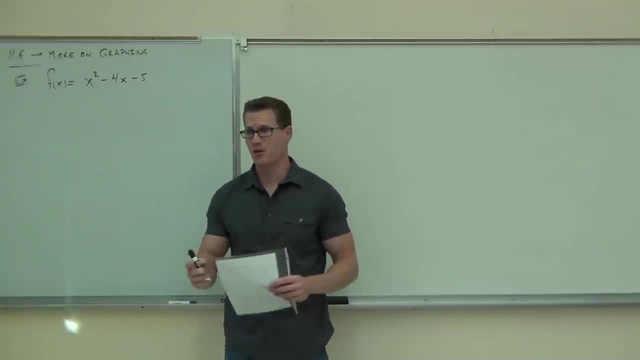 you some steps on how to graph, But trust me on this, These steps have to be followed in order. Can you do that for me? Don't just jump around on these steps. You've got to do them in order, Because on one of these steps we might be changing signs a little. 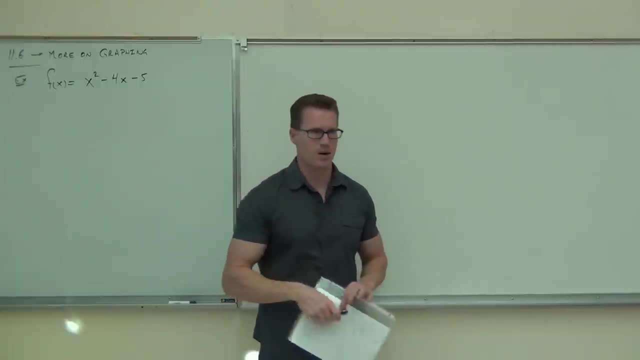 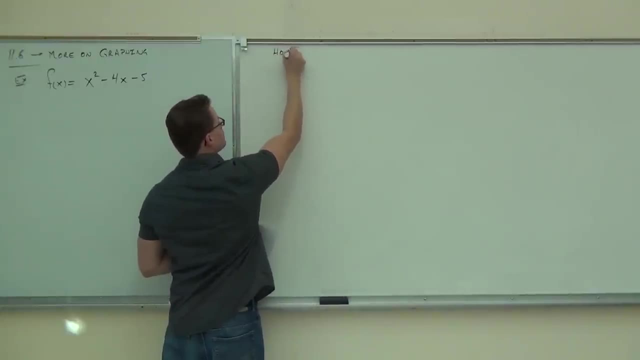 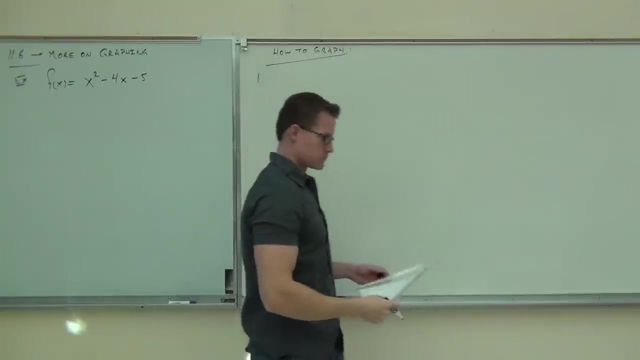 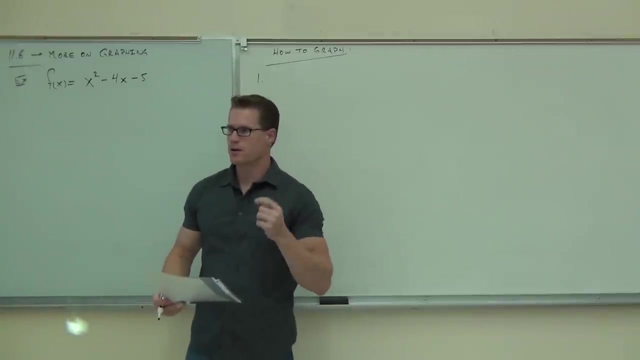 bit, And if you do that before you graph these other parts, it's not going to come out. You're going to get the opposite facing graph. So here's some steps on how to graph Number one. The first thing you're going to do, you're going to find the vertex, The 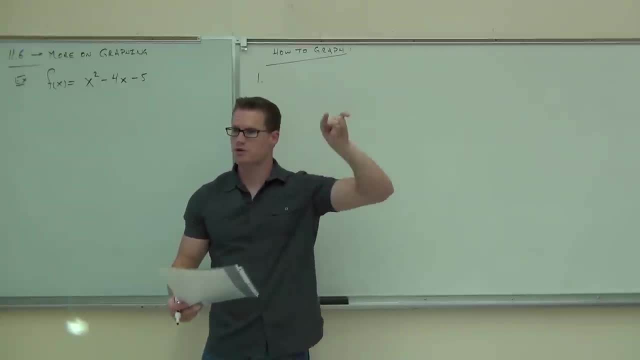 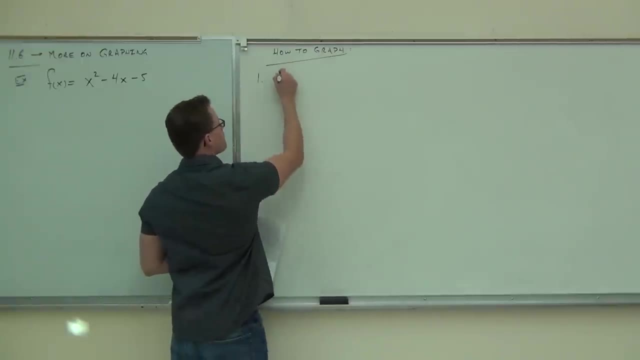 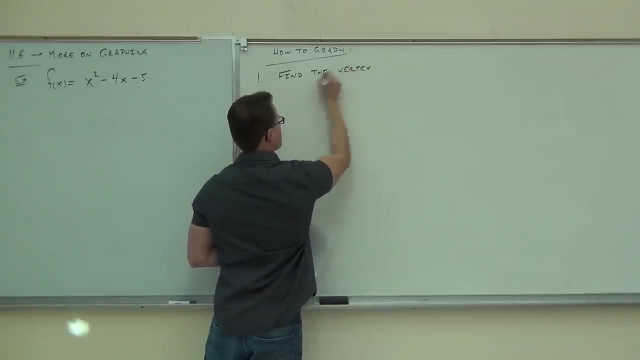 vertex is the highest or lowest point of your parabola. It's where you switch from decreasing to increasing, or increasing to decreasing. It's that point, Oh my gosh. now how do we find the vertex? 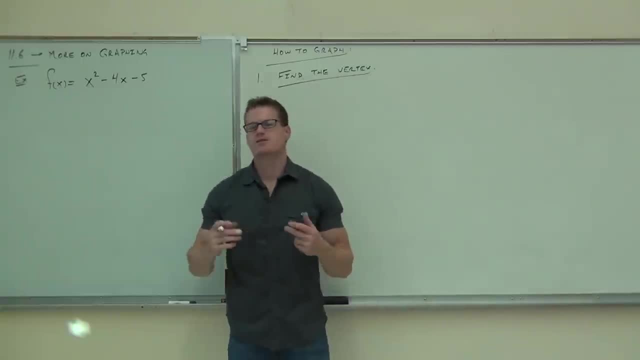 Well recognize. firstly, the vertex is a point right. It's an x comma y or an x comma f of x or an x comma. It's what you, your x coordinate, combined with your vertical component, there, your horizontal and your vertical. 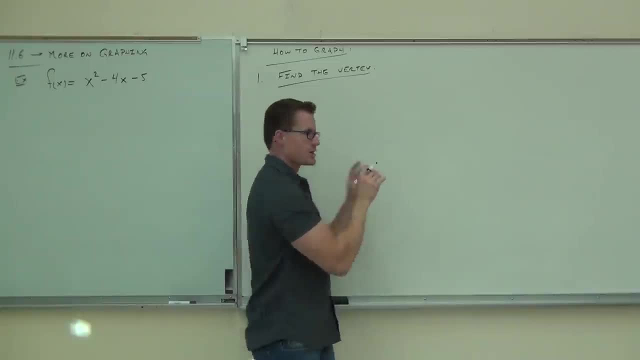 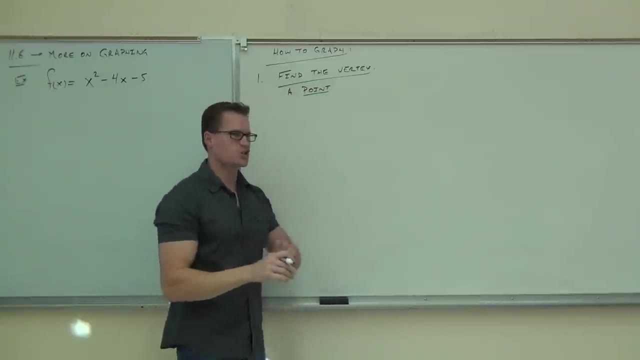 You with me on that. It's something, comma, something. You follow me? This is a point. The vertex is not just one number. okay, You don't say, oh, my vertex is four. You got to say four comma something, because otherwise, 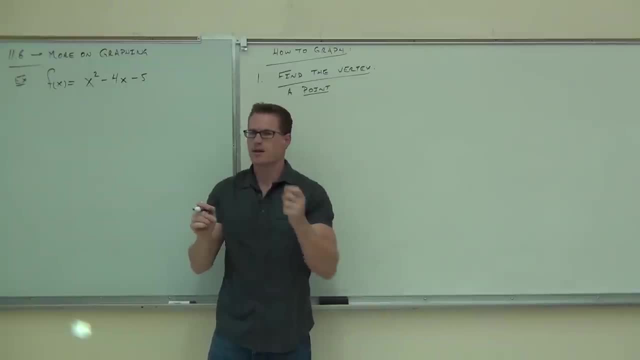 you just go over to four all the time, or two. Well, that doesn't make any sense. We got to have some sort of point. So here's what the vertex looks like. It is a point. I'm going to show you how to find the vertex. 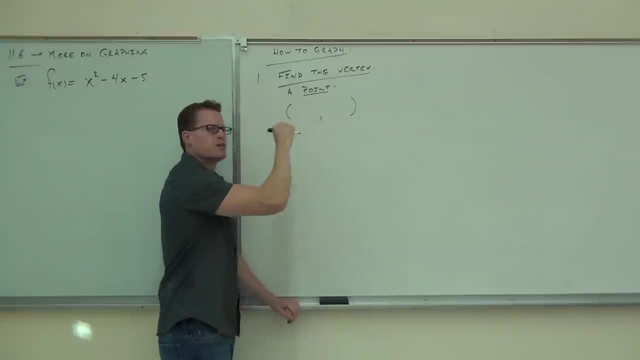 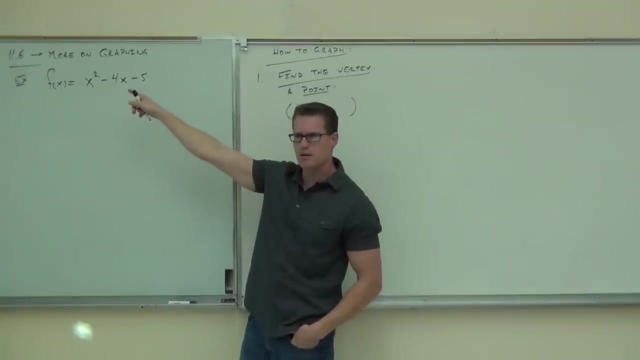 The x coordinate is given by this little bitty formula. It's not a hard formula. You just got to make sure your signs are right. By the way, can you all Identify a? How much is a again One? How much is b? 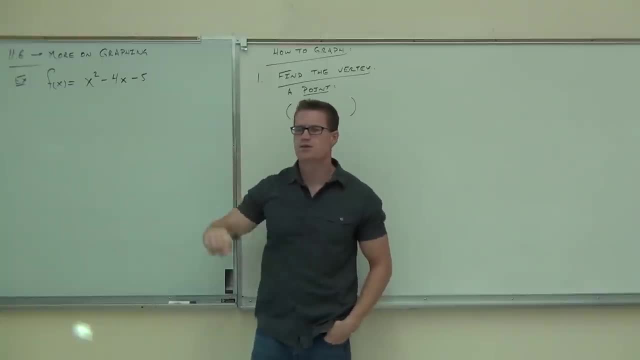 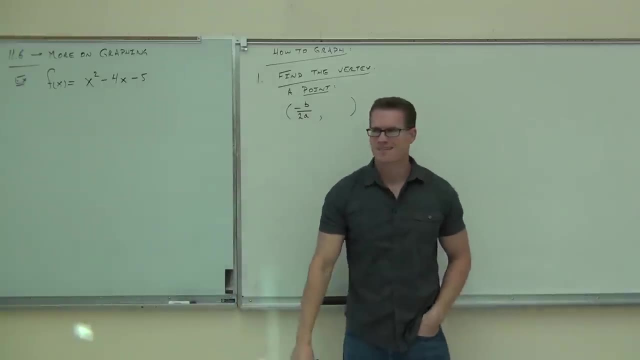 Negative four. Negative four. good, How much is c? Identify our left. Here's your vertex. Negative b over 2a. Does that look familiar? Does that look familiar? Yeah, that's part of your quadratic formula. That's actually what we subtracted from both sides. 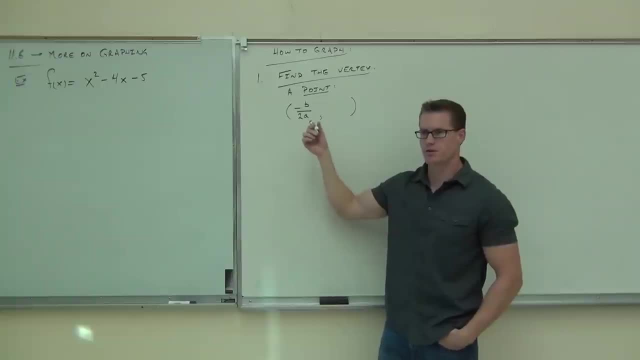 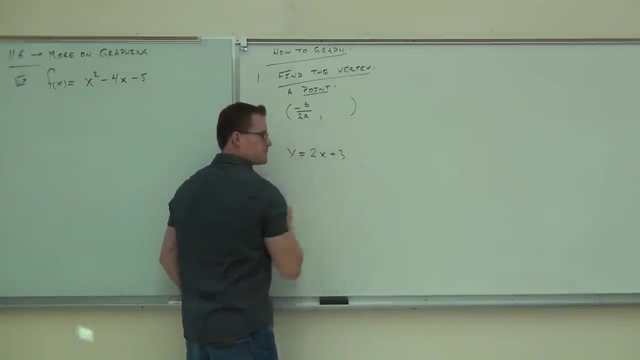 after we completed the square, That right there gives you an x coordinate for the vertex. Now wait a second. How do you find that one? How do you find that? Let me get you there mentally. okay, If I said y equals 2x plus 3, and I said find the point 5 comma something. 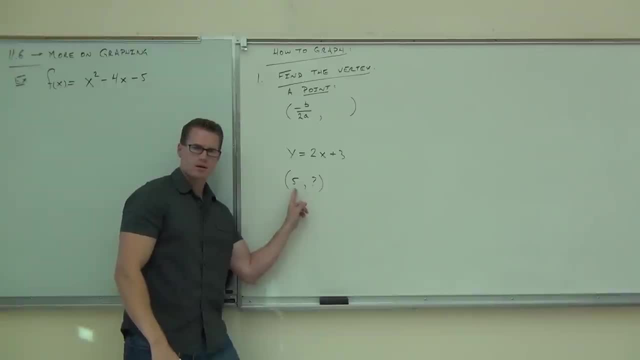 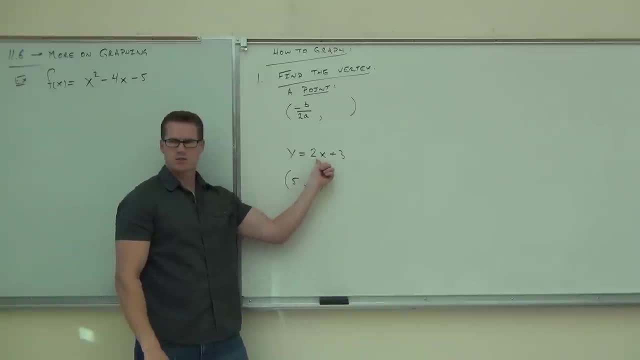 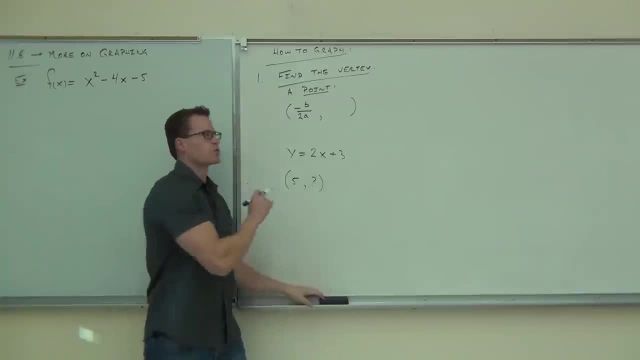 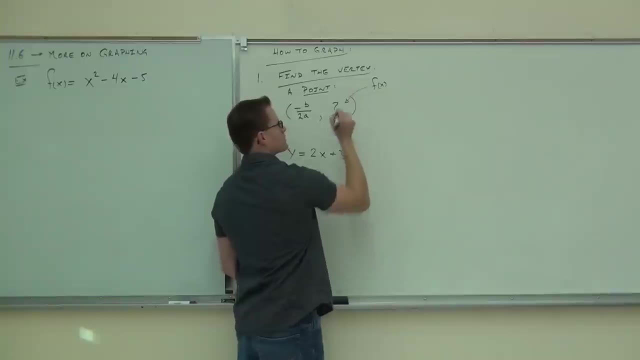 That would be 13. are you following on that? That's what we're gonna do here. This is a question mark, but we get that by plugging it into f of x or whatever your function is. Let's try that over here and we'll stop there. 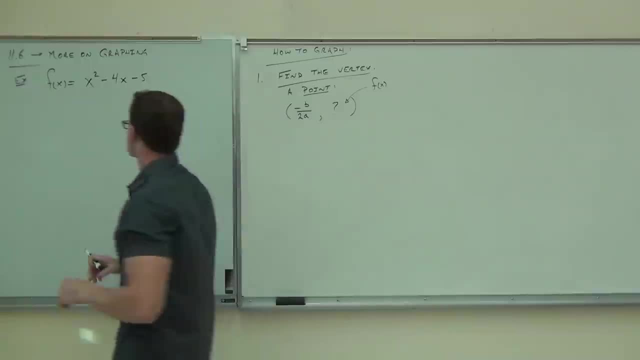 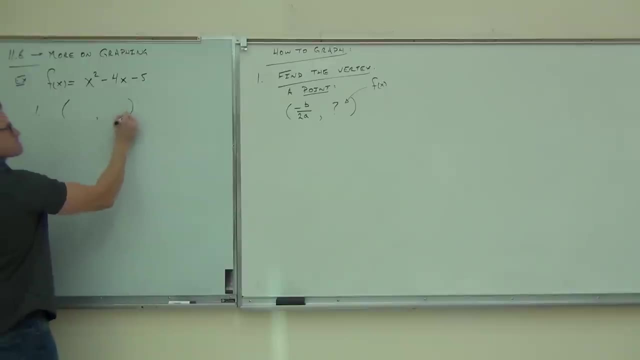 Remember that clock's five minutes fast. I told you that at the beginning of class. So first thing, we're going to find the vertex, step number one. Vertex is a point. It's negative b over 2a. So in our case, what's our b again? 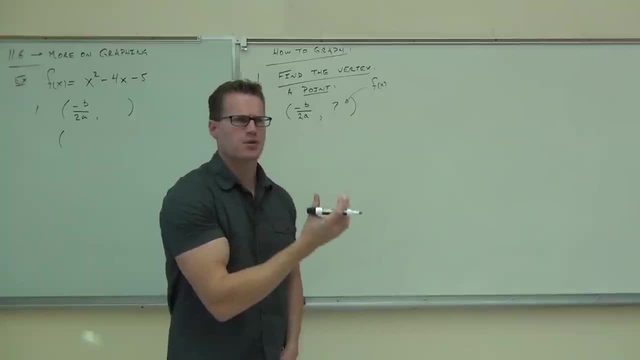 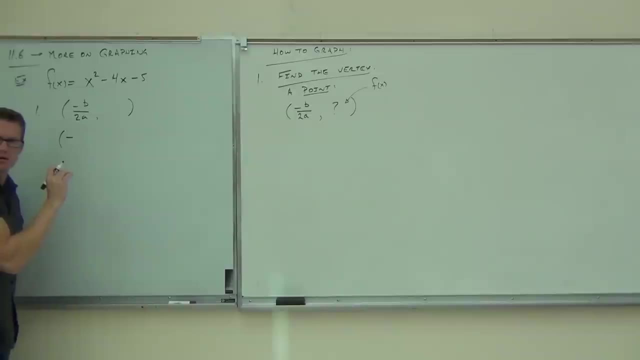 Negative 4.. So write this out. Don't do any math in your head, Just write everything out first. I have a negative, regardless of what b is. How much is b now Negative 4.. So am I going to have negative 4 or negative negative 4?? 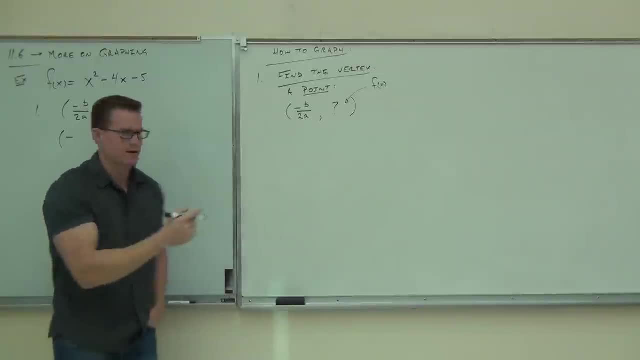 What do you think? Negative, 4. Negative, negative 4. Okay, Over 2 times. what was that? 4. Comma question mark: I don't know what that is yet. Okay, Now, let's go slow on this. 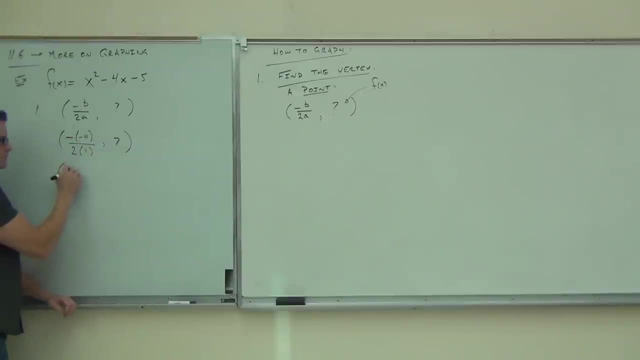 What's negative? negative 4, folks. What's 2 times 1?? 2. Comma question mark: 4 over 2, that's 2 comma. Now don't leave it. I'm having to write this in the point notation the whole way down. 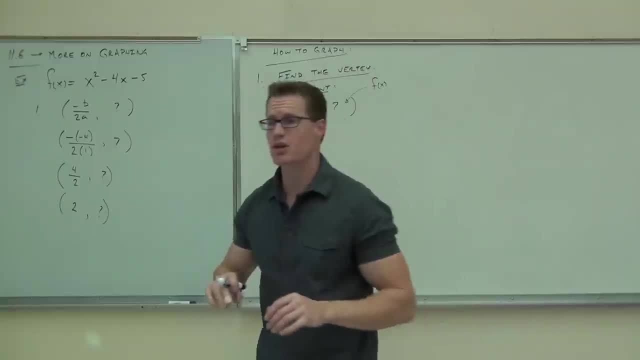 so you don't forget that. it's a point. You see, the problem is, I have a lot of people who do this and go, oh, the vertex is 2.. I go: oh, what? What do you mean? the vertex is 2?. 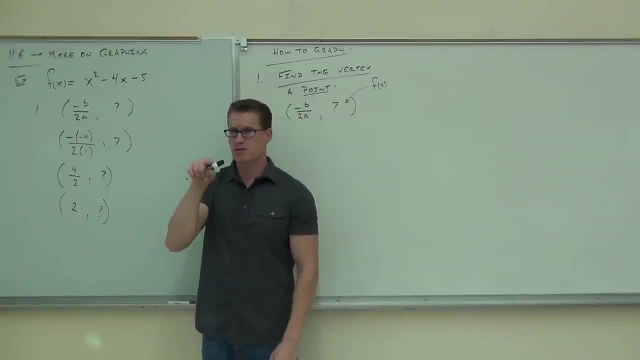 You can't just say 2.. It means you go over to 2 and then you just: where do you go? right, If you mean 2, 0, you put 2, 0.. You want 2 comma something. 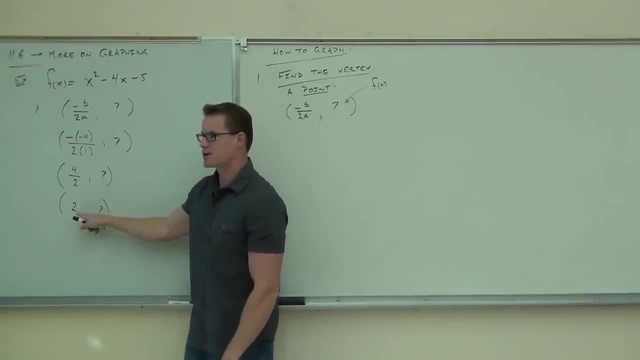 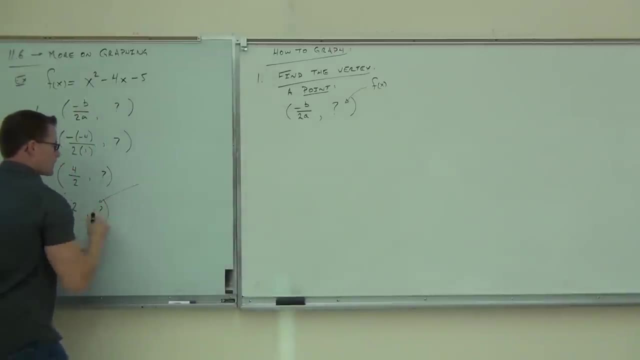 It's going to tell you the height. now, The way you get your height is you plug this into your original function. Are you with me on that? So what we're going to do off to the side here. that's why I left a whole bunch of room over here. we're going to have f of 2.. 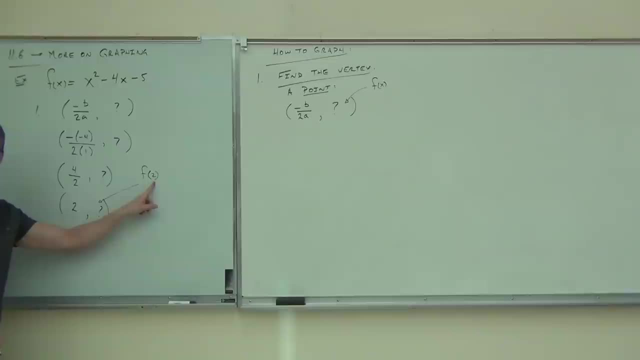 f of 2.. Where am I getting that 2 from, ladies and gentlemen? Where am I getting the 2? From the left, What you just found? Okay, you find this first, then you plug it in. What's f of 2 mean? 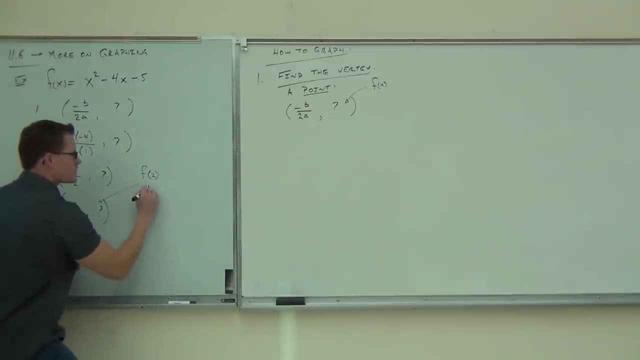 Well, it means look back up there, plug in 2.. You're going to get 2 squared minus 4 times 2,- I can use parenthesis there if you'd like- minus 5.. That's 4 minus 8 minus 5.. 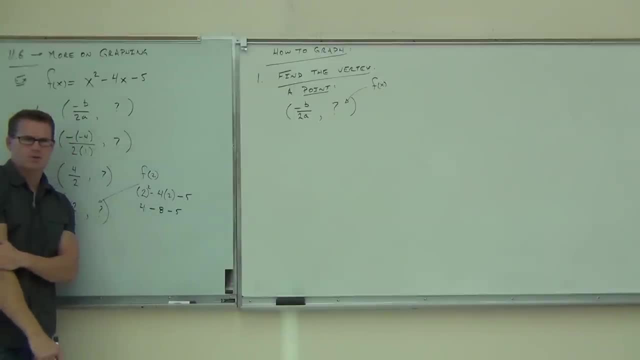 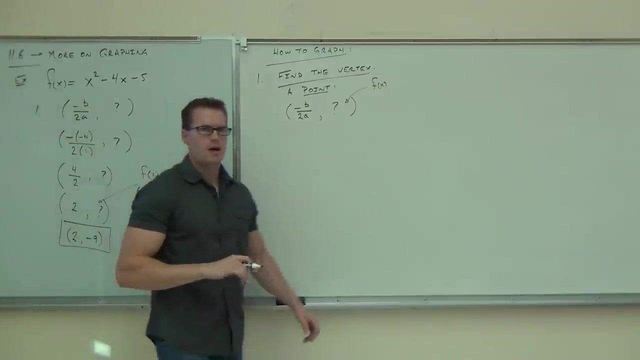 You see where those numbers are coming from, folks. Yep, What's 4 minus 8 minus 5? Positive or negative? 9? Negative, Negative, 9.. That right, there is your vertex. That vertex is going to tell you the highest or lowest point of your parabola. 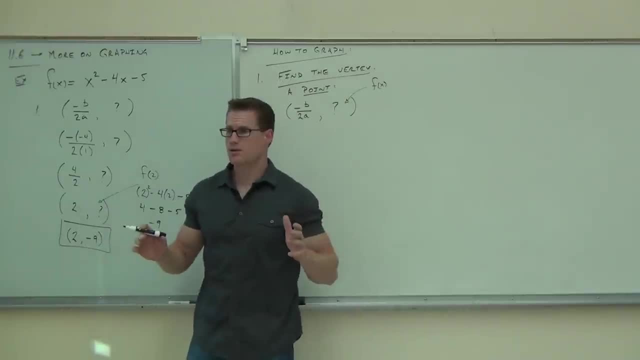 Next time we're going to work on steps 2 and 3.. They're very quick. Steps 2 and 3 are very nice. They use what you've learned before in this class. This is honestly the hardest part for you. Can you do the hardest part? 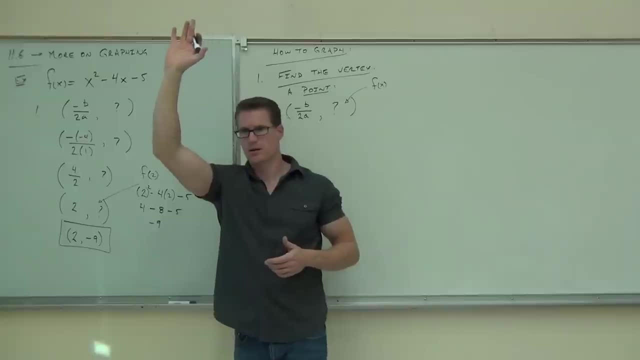 I know. I mean we'll feel okay with what we've talked about so far today. Okay, if you're not raising your hand, I'm going to assume you you don't? are we okay or no? no, I still got time. 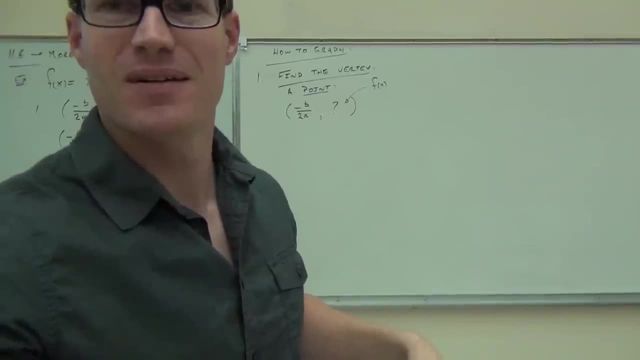 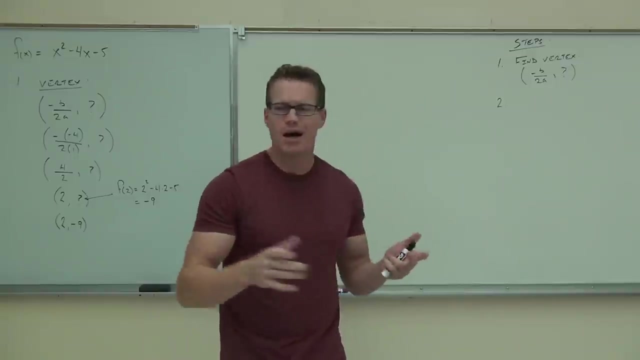 I mean, we can continue, I'll do. I'll do what you want. So, if you remember from last time, we're trying to graph this thing a little bit more accurately than just shifting things around. Last section we were just shifting, but when we get quadratic functions like this, 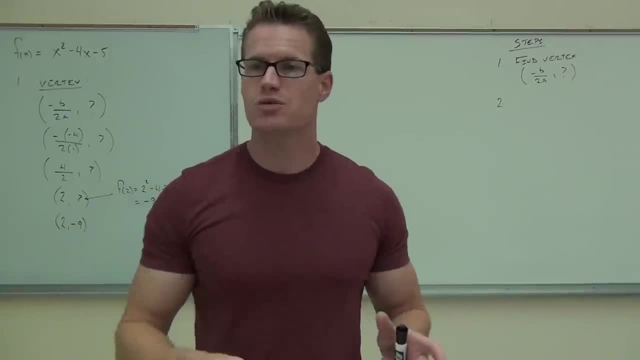 it's not really the appropriate form to shift it. Now we can do certain things with it, and the first step to graph these- remember, you've got to do these in order- the first thing is to find the vertex. The vertex is a point. 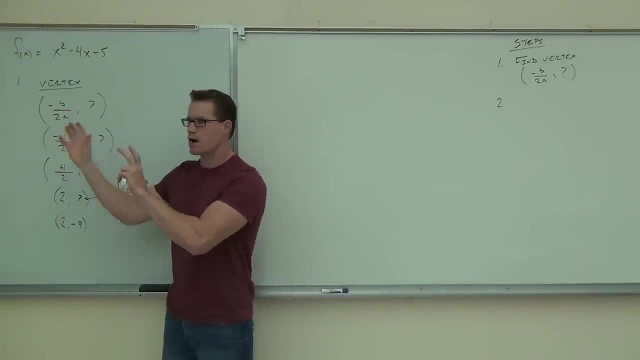 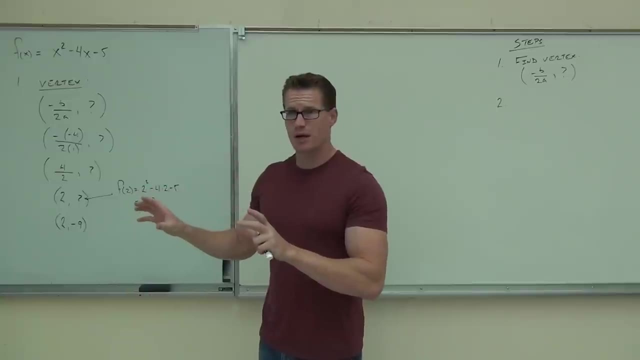 So when we have this, of course we're going to, we're going to have a point: something x coordinate comma, something A- y coordinate, how you find that you take the negative b over 2a. you remember finding the a, b and the c right. 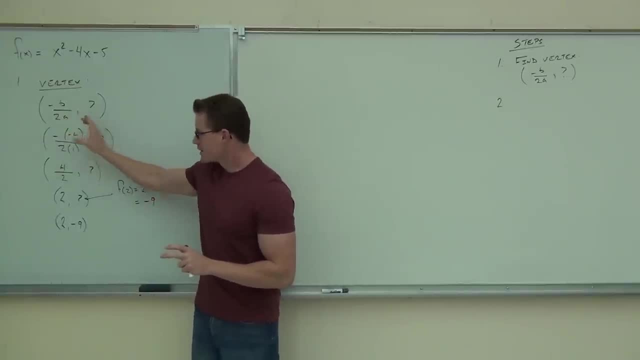 Just like quadratic formula, we use just the a and the b. we plug that in, we substitute it in, we figure that out. how do we find this y coordinate? What do we do to find that, that negative 9 in this case? 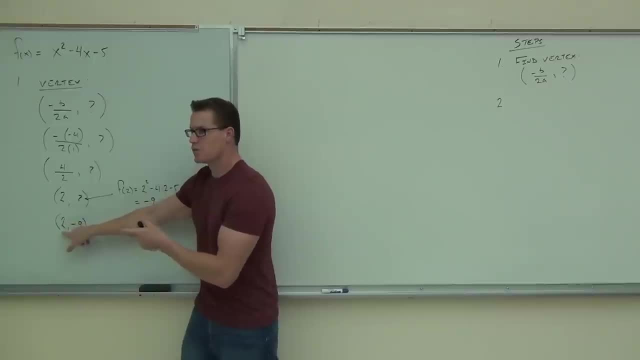 Good, okay, so this is my x right. So once you find your x, you plug that in for x. That'll give you your y coordinate and that gives you your point. Raise your hand if you felt. okay about that so far. 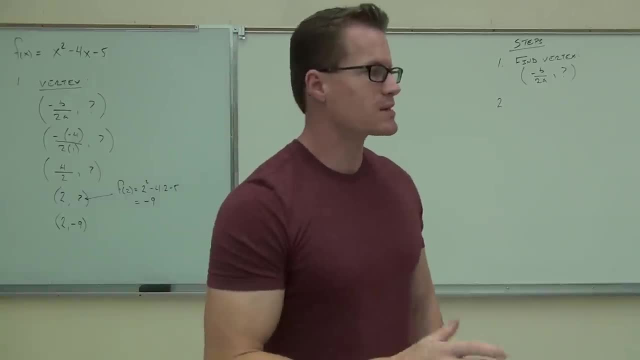 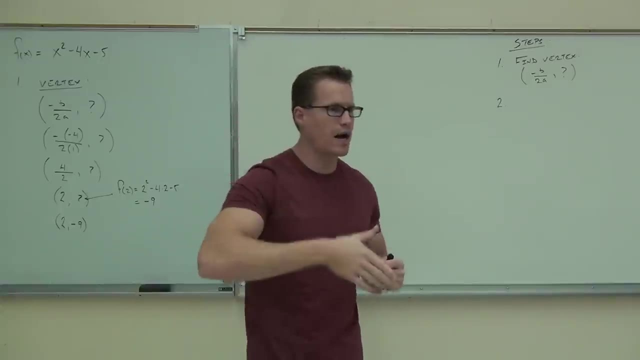 Good, now we do have a couple more steps. you see, in order to be really, really accurate with these things, we need to find what's called our intercepts. Our intercepts are where we're going to cross the y axis and the x axis, so there's two. 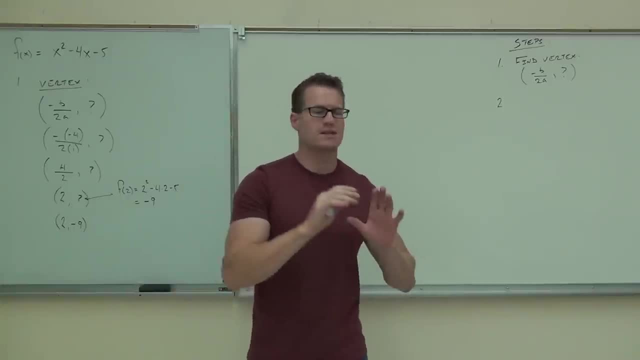 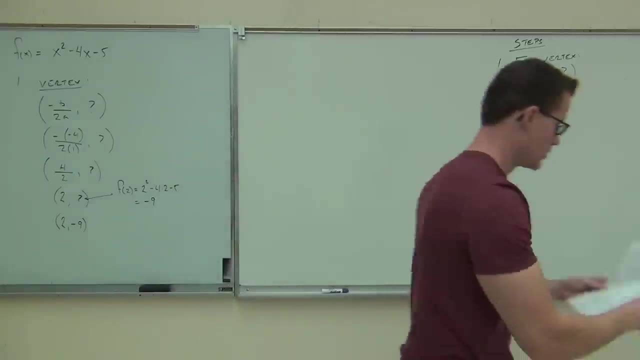 sets of intercepts. we need to find The y intercept, that's the easy one, and the x intercept, which takes just a little bit more work. but hey, you know how to do it already. So step number two, which we're going to do up here, is find the intercepts. 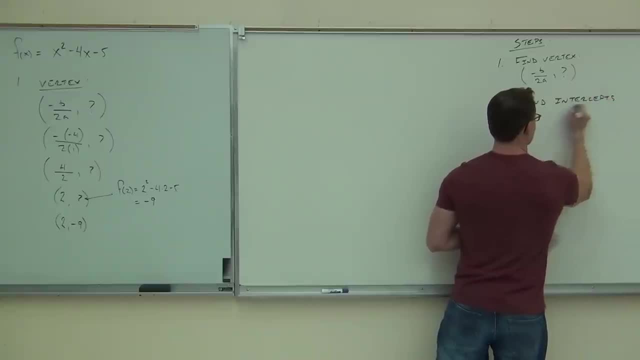 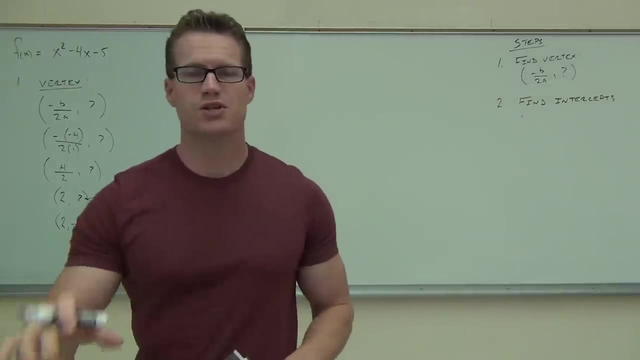 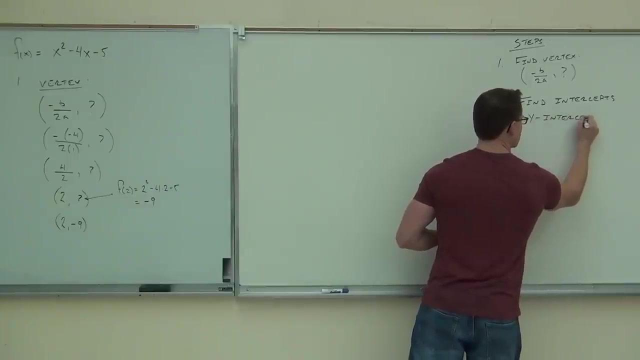 Find the intercepts. We'll talk about the y intercept first. That's the nice and easy one. you're going to see this in just a second To find the y intercept. by the way, if you don't remember what the y intercept is, that's: 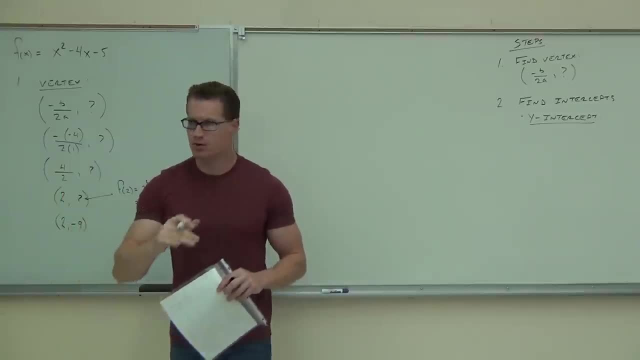 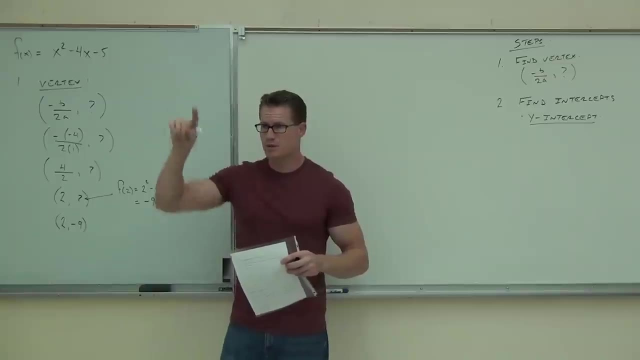 the point where the graph crosses the y axis. Every graph is going to cross the y axis, Not every graph is going to cross the x axis. I need you to look up here for a second. Remember that with parabolas we have this shape right. 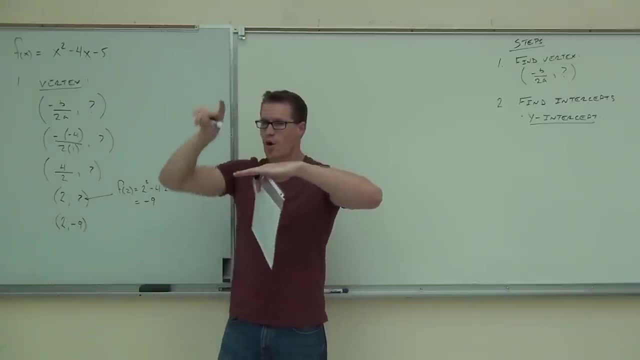 So you could be above the x axis, or you could be below the x axis, or you could be right on the x axis, or you could cross it once and then cross it again. So we have several options for us to have for x intercepts, but every graph with parabolas. 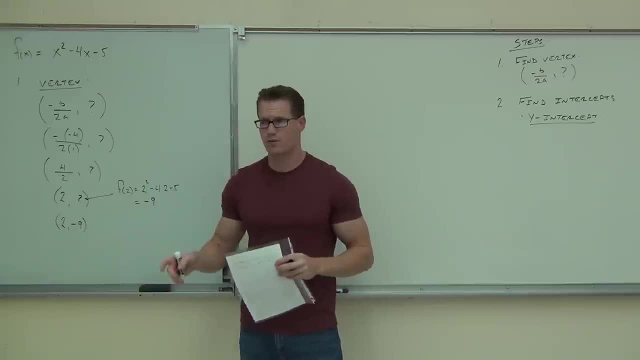 is going to cross the y axis. You with me on that, Every single one of them. Here's how you find it Very, very nice and easy. Can you guys look back up here? Can you tell me what the constant is? 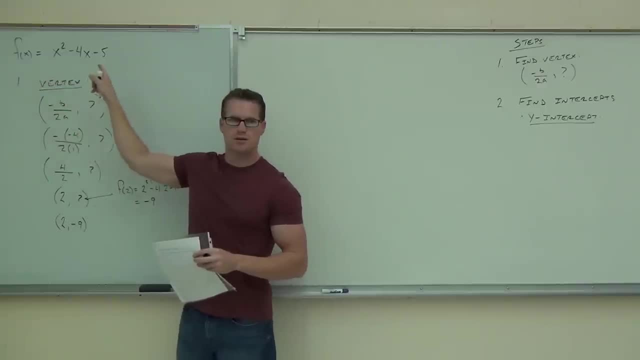 What constant number is Five, Negative five, Five or negative? five Negative five, Negative five. That's the y intercept, It's just the constant. And here's how you figure that out, And we're going to graph this in a second, so I'll make my graph up. 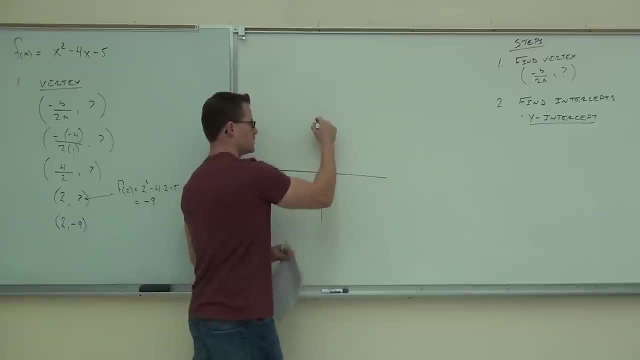 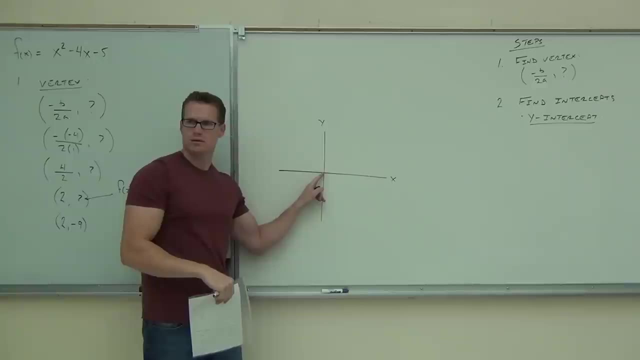 Which one's my y axis, Option one or option two? Option two, Definitely. If I want to find out where I crossed my y axis, my x coordinate is zero, right? You see that If I plug in zero, what happens? 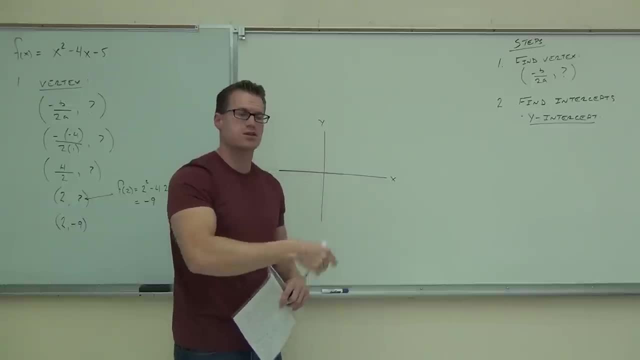 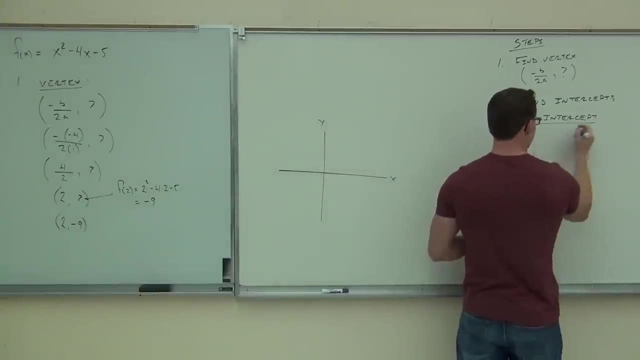 Zero, zero, negative five. That tells me where I'm going to cross my y axis. So right here, when we're trying to find a y intercept, the y intercept is simply the constant. It's that c. So the y intercept is c, just that constant. 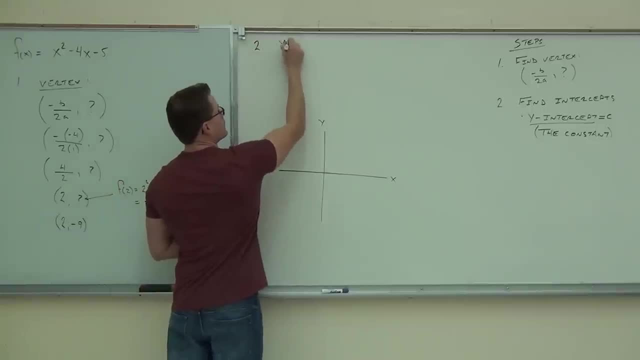 So over here we're going to put our step two and we're going to put: y equals the y intercept. I'm sorry, I'm going to be a little more specific on that. The y intercept equals, in our case, what was our y intercept? again, ladies and gentlemen, 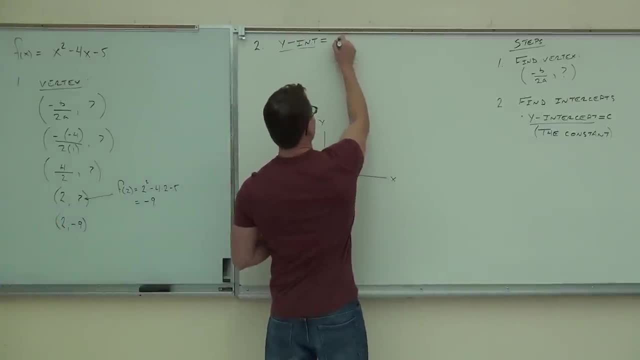 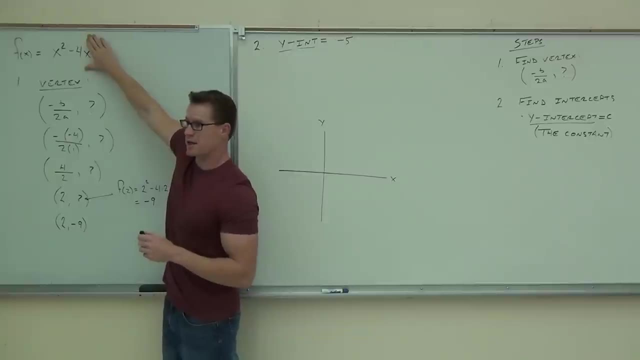 Negative five. Negative five, It's just the number, Just that constant off to the back end. Now, by the way, what if there was no number? Look up here at the board. What if I had x squared minus 4x? 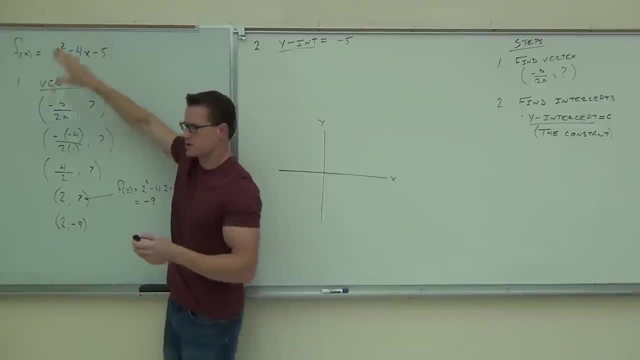 That's still a quadratic. What would the y intercept be there? Zero, Good, Okay, You're getting the hang of it Now. the next set of intercepts takes a little bit more work, but you're going to see that you've already done this before. 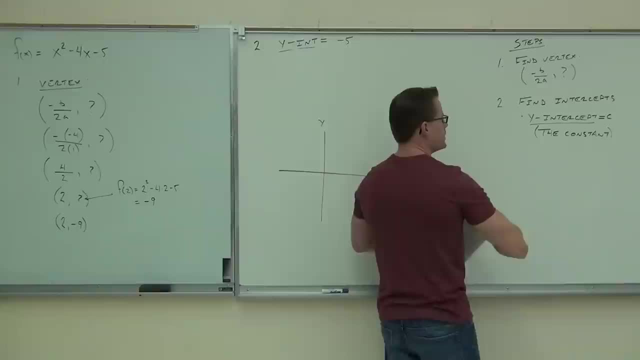 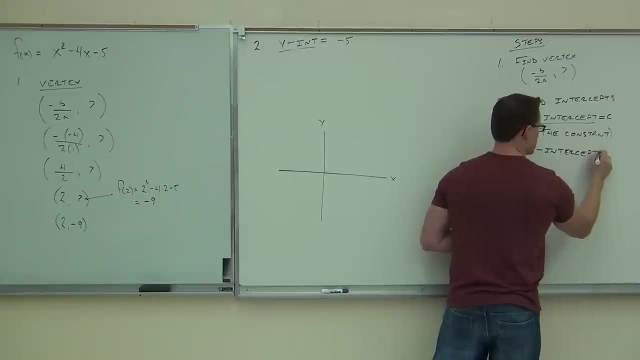 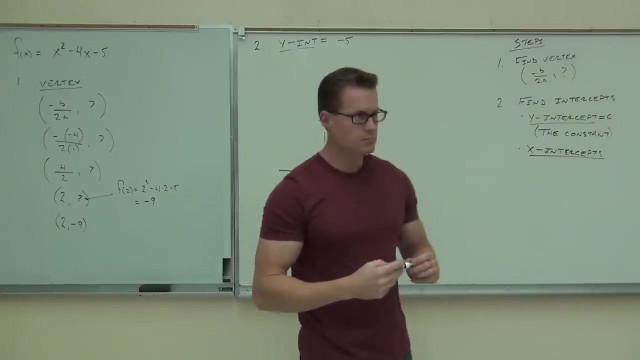 This is kind of cool. It wraps some things together for you. The next thing we've got to do is talk about our x intercepts. Talk about your x intercepts. Well, what we learned a long time ago was when we're actually solving the quadratic equations. 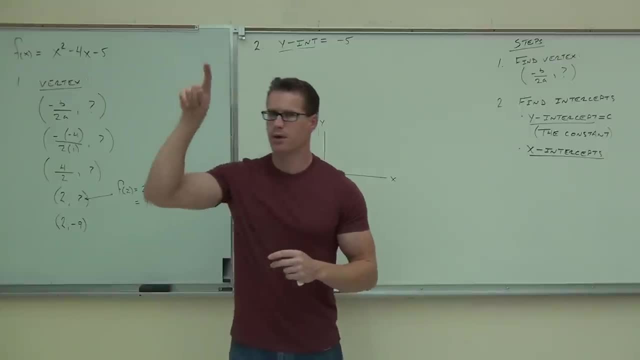 when we're solving those things, we're finding out where that parabola crosses the x axis. Do you remember talking about that? I hope you do, If you don't look back at those videos, because I said it was just a blurb. 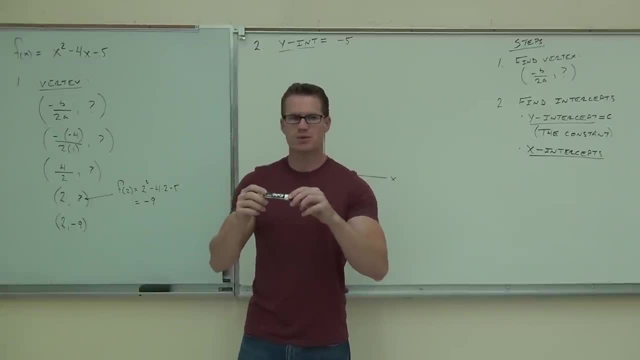 It was maybe a minute-long speech, But what we're doing is we're finding out: if the parabola crosses it once, it crosses it twice. If it touches it, it might only touch it at one spot on that vertex. It might not even touch it at all. 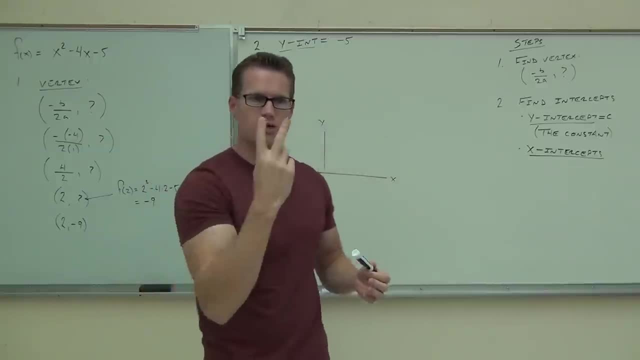 We find that by solving the quadratic equation- Remember doing that- We get two solutions. That was those two crossings. Or we get complex solutions which means we don't cross that at all, Or we get one unique solution. That means the vertex is touching that x axis. 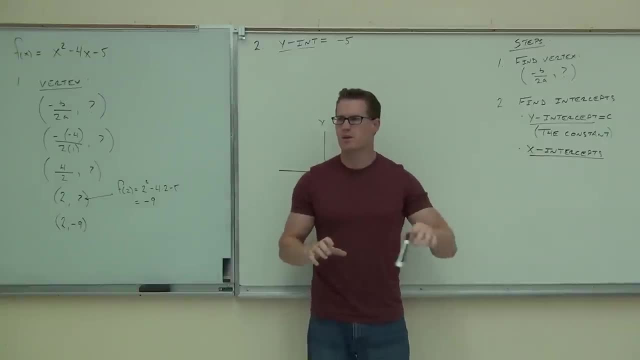 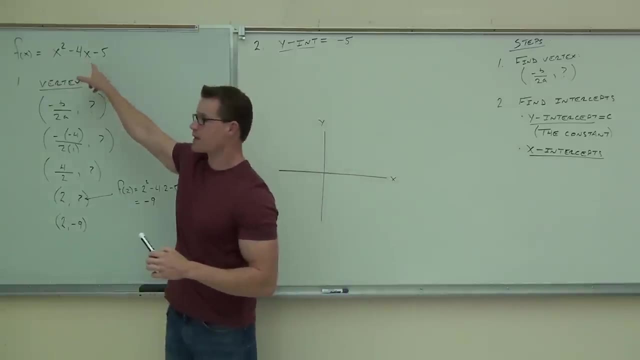 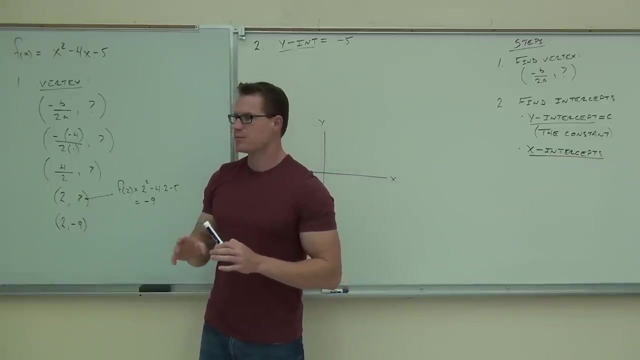 But in every case we found those x intercepts by solving the quadratic equation. So here's what we do. You look back at your quadratic. Our quadratic up here is x squared minus 4x minus 5.. If you set that thing equal to 0, if you set that thing equal to 0 and you solve it. 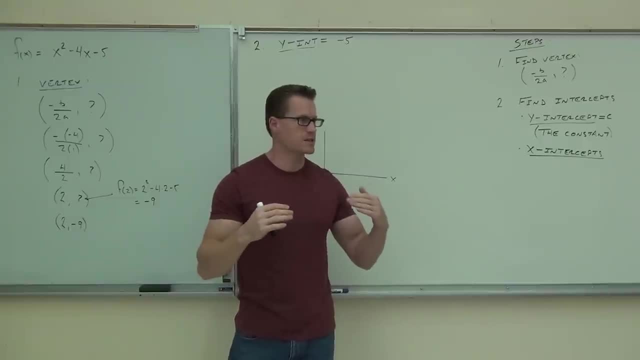 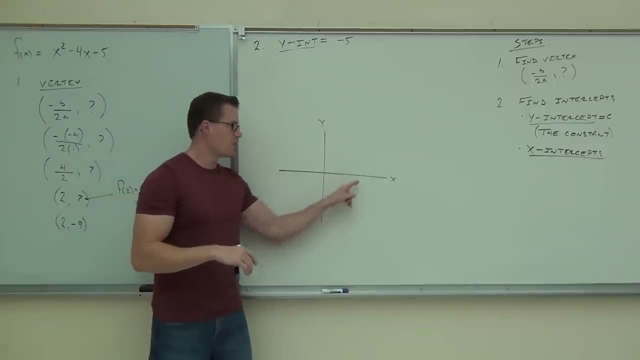 you're going to find out where that graph crosses the x axis. Think about that for a second. Think This is our x axis, right? We're trying to find out the x intercepts where it crosses. What's the y coordinate? 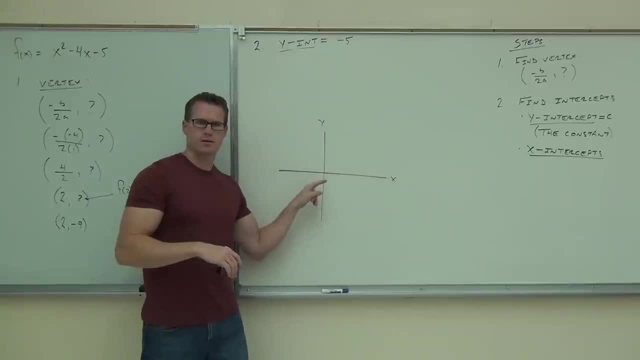 What's the y coordinate all along this x axis? 0. 0.. Yeah, The y value is 0 for this whole thing, right, Yes or no? Yes, This is 1 comma 0, 2 comma 0, 3 comma 0, negative. 4 comma 0, right. 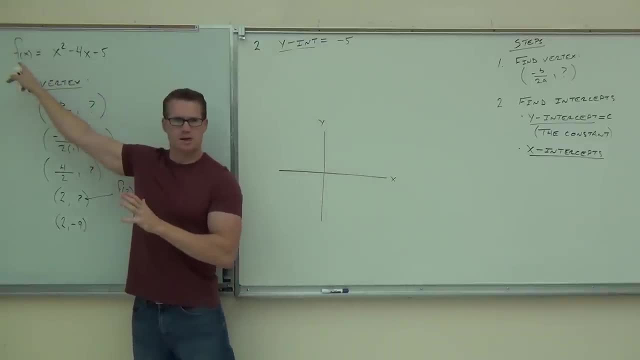 So if we set this equal to, That's like your y. You notice that for a second right, That's your y really. I mean we just call it f of x, but that's y. If we have 0 equal to this, it's going to give us where we cross our x axis. 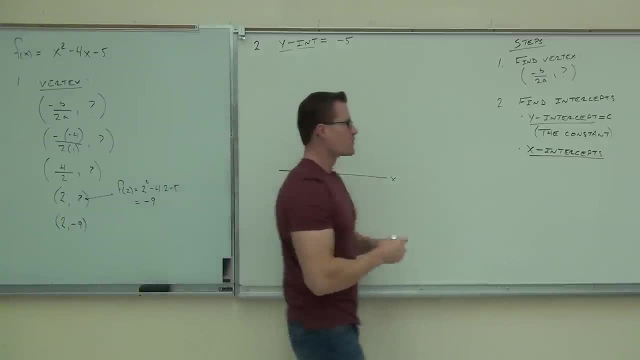 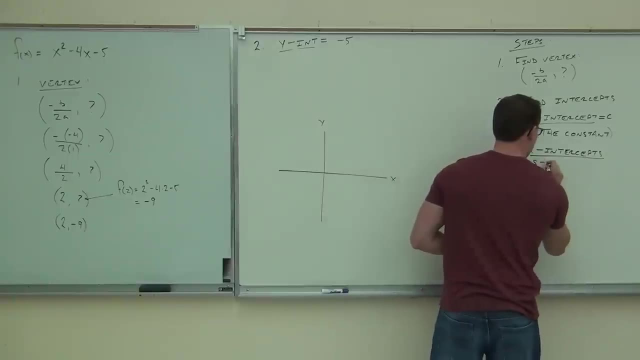 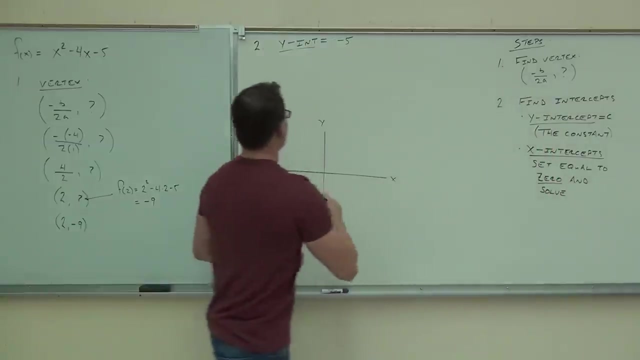 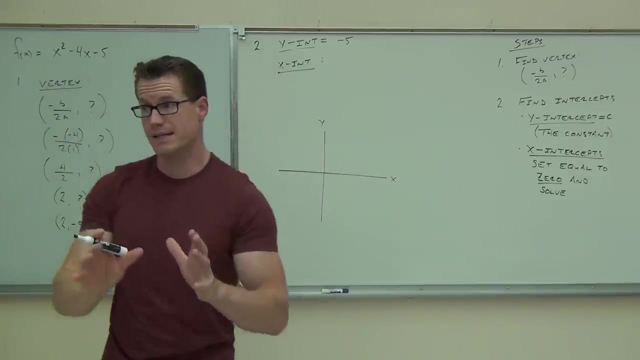 Not sure if you're with me on that. Okay, So for x intercepts, we're going to set the equation equal to 0 and solve it. So y intercept: very easy, It's just a number. So x intercept: a little bit more work. 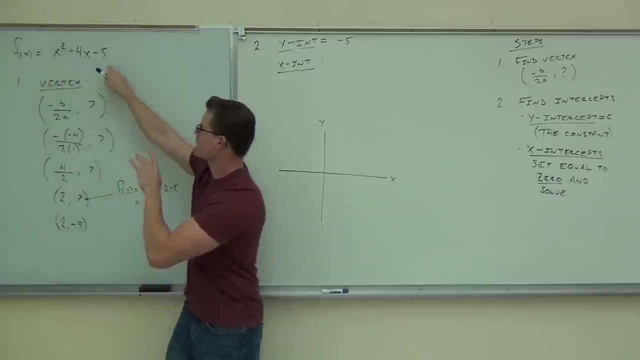 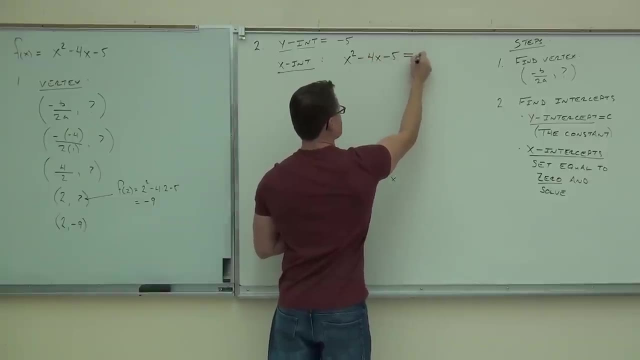 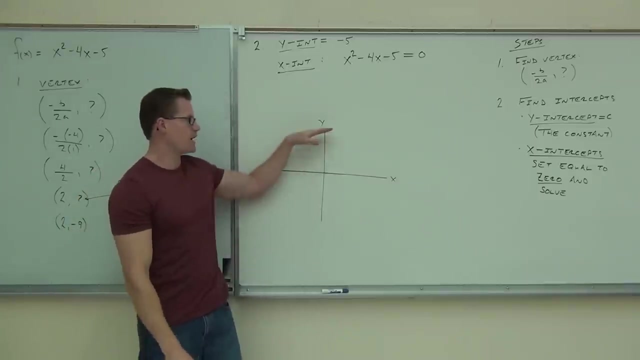 Let's see how we do this. The quadratic equation right here is going to be x squared minus 4x minus 5.. And we're going to set it equal to 0.. You see where the 0 is coming from. 0 is coming from the fact that I'm going to find out where y or f of x is equal to 0.. 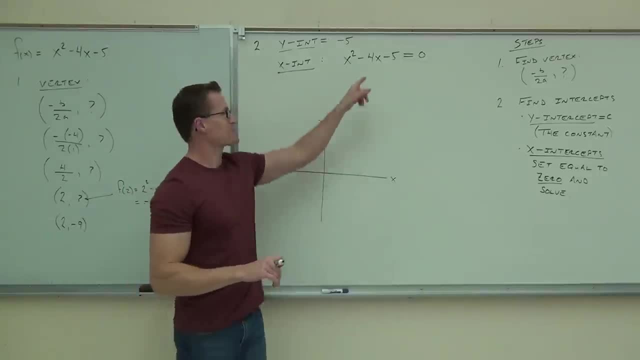 That's going to give me my x intercepts. Hey, does that look familiar? Does that look familiar to you? Oh yeah, We've been doing that since chapter 7.. Actually, before that, We have a couple of ways we're supposed to look at this. 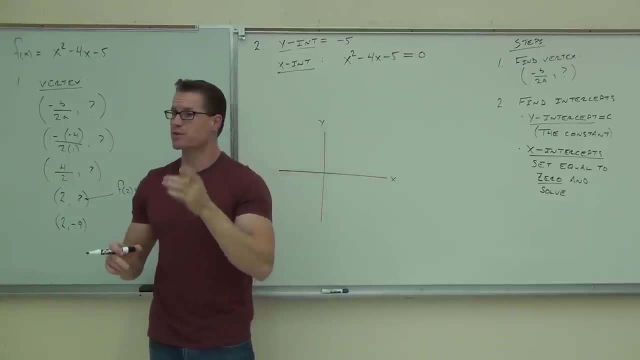 What's the first thing we should do to try to solve that equation? How long should you spend trying to factor, And if you can't do it in 10 seconds, what else are you supposed to do? Great, So now you have two options. 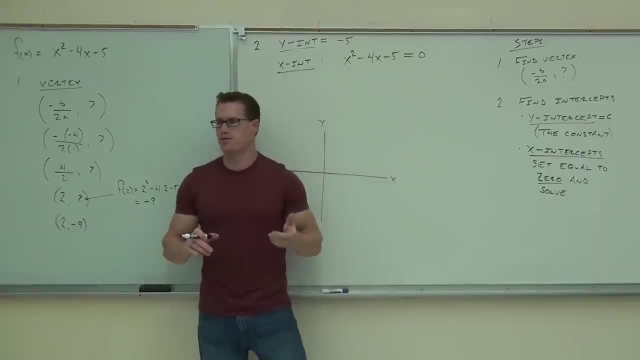 The quadratic formula will work every time, but factoring is often quicker. if you can't do it, You guys ready to try it? Let's see if we can factor it. Of course we'll do a diamond problem. We'll spend 10 seconds trying to do that. 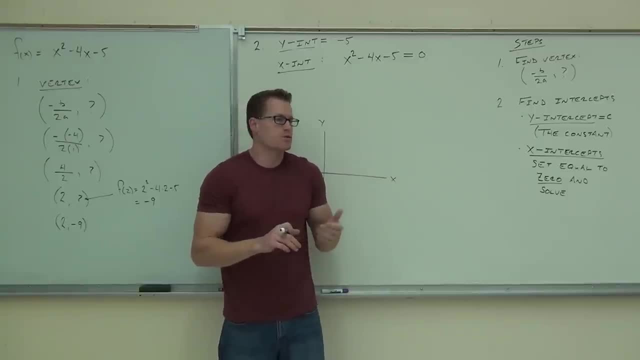 Okay, So now we have two options. The quadratic formula will work every time, but factoring is often quicker. if you can't do it, You guys ready to try it? Let's see if we can factor it. Of course we'll do a diamond problem. 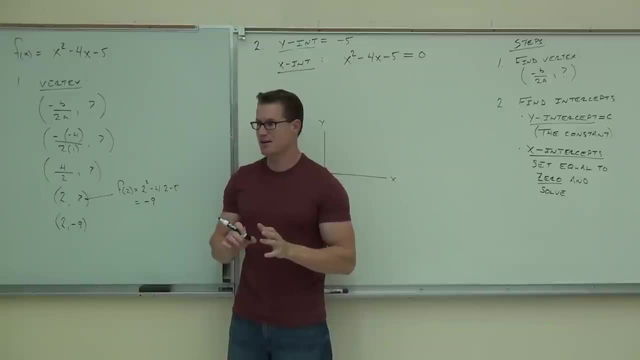 We'll spend 10 seconds trying to do that. Were you able to factor it? I'm getting like minus 5, minus 1.. I'm sorry, minus 5 plus 1.. Good thing I'm not getting the other one right. 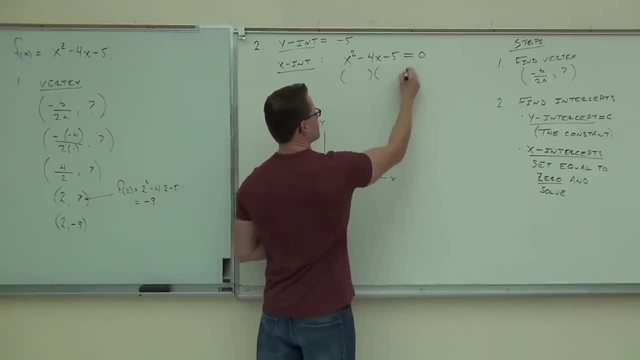 That would be wrong. Okay, So now we have two options. What's the first one? The quadratic formula will work every time, but factoring is often quicker. if you can't do it, You guys ready to try it? Let's see if we can factor it. 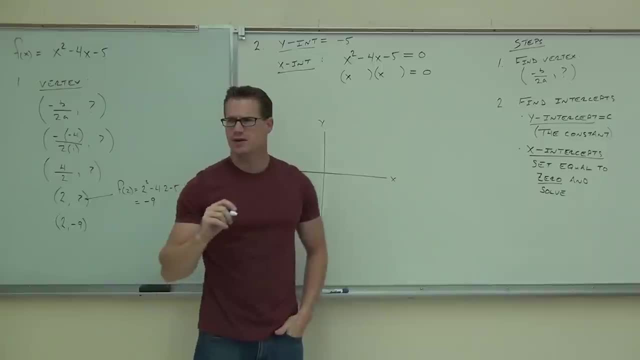 Of course we'll do a diamond problem. We'll spend 10 seconds trying to do that. Were you able to factor it? I'm getting like minus 5, minus 1.. I'm sorry, minus 5 plus 1.. 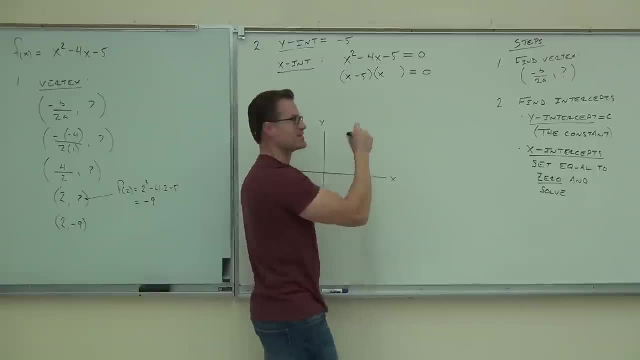 Good thing I'm not getting the other one right. That would be wrong. Okay, Now are you done on that? You done on that? What else are you going to do? Yeah, So don't forget the things that we know how to do already. 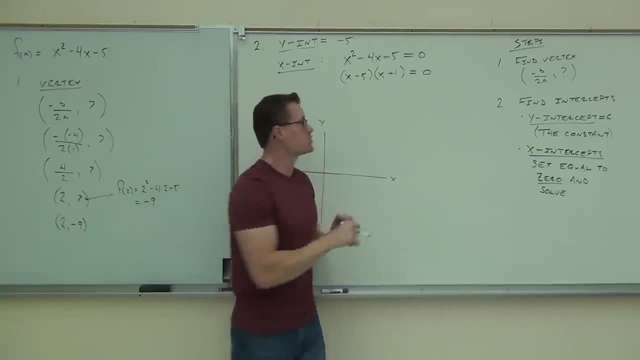 So we're going to do x minus 5 equals 0 and x plus 1 equals 0. If we solve these, we get x equals 5 and x equals negative 1.. Okay, I need an honest show of hands. How many of you feel okay getting down to that far? 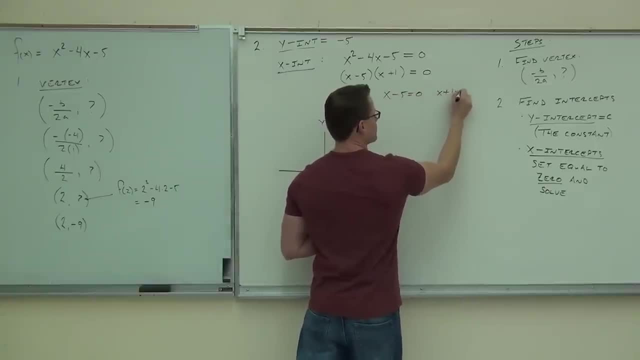 So, really, let's look at what we're doing. Okay, Just a simple recap from last time. First thing we're going to do is: we're going to do this, We're going to do this, We're going to do this. 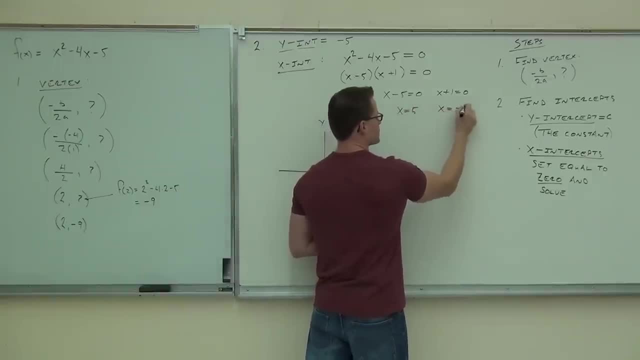 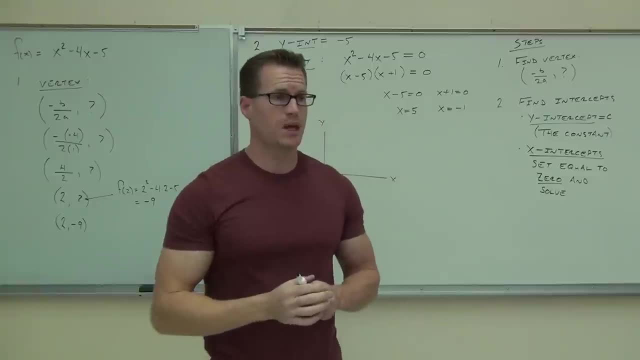 So really, let's look at what we're doing. Okay, Just a simple recap from last time. First thing we do, we make sure we have a quadratic. That's x squared Quadratic function. That's what that means. We find the vertex first. 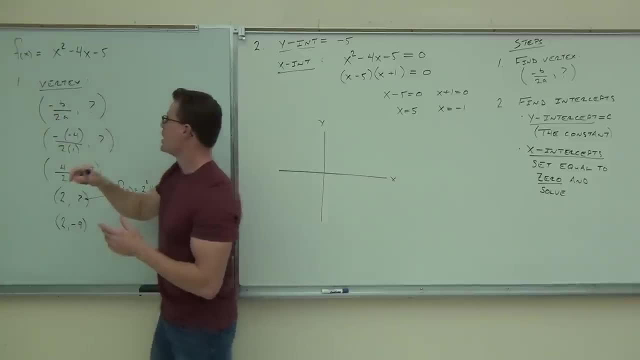 That's the first thing you've got to do, Because sometimes on this step we'll change some signs around. I'll show you that in about three examples. Find our vertex first. That's negative b over 2a. It's just a formula. 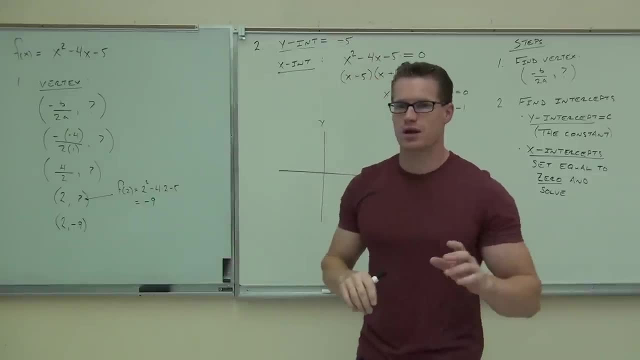 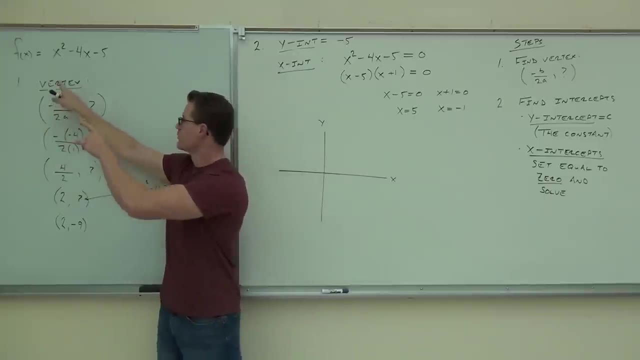 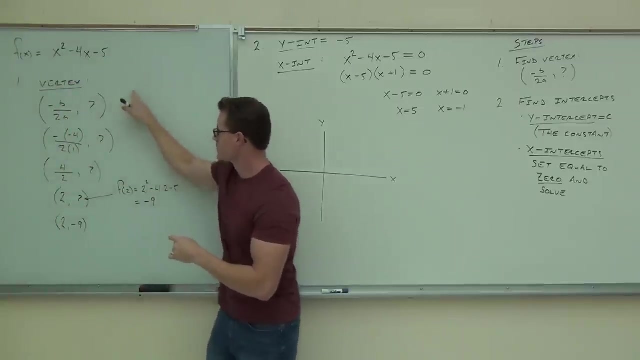 You find that from your coefficients of negative b over 2a, You find that from your coefficients of negative b over 2a, You find that from your coefficients of negative b over 2a, We figure out our x coordinate first. We plug that back in to figure out the y coordinate. 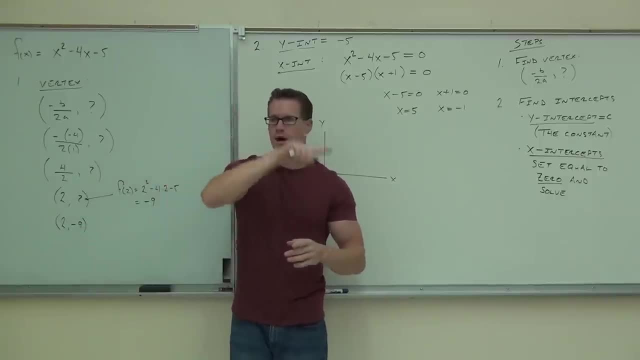 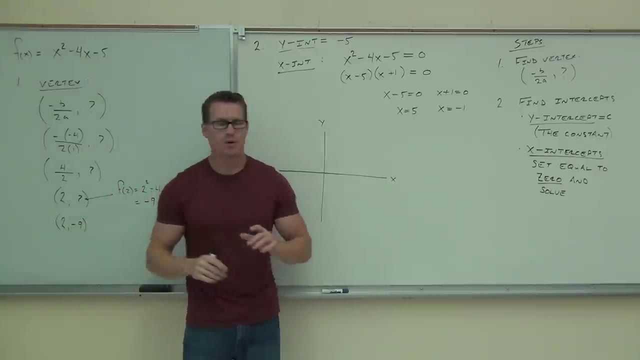 That gives me the point that is either going to be the lowest or the highest point of my parabola. You with me on this so far? Then what we do is we find our y intercept. That's the easy one, It's just that constant number. 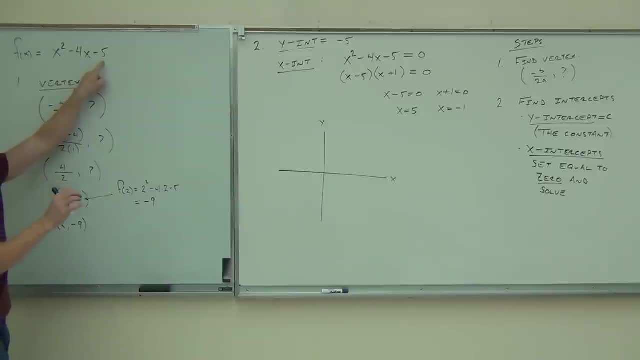 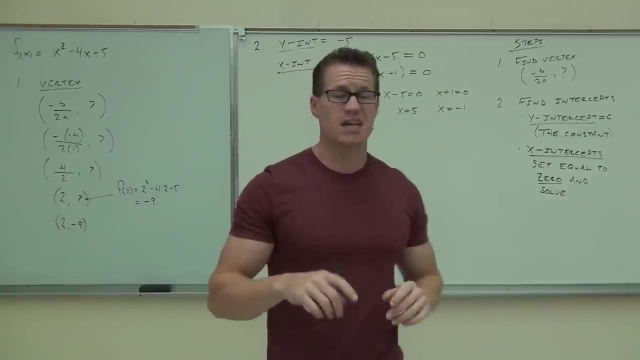 It's always going to be at the back end of your function. It's with a constant number with the sign. that's what you have out of that. So here we got negative five. Lastly, the very last thing you do, you find your x-intercepts, if you have any. 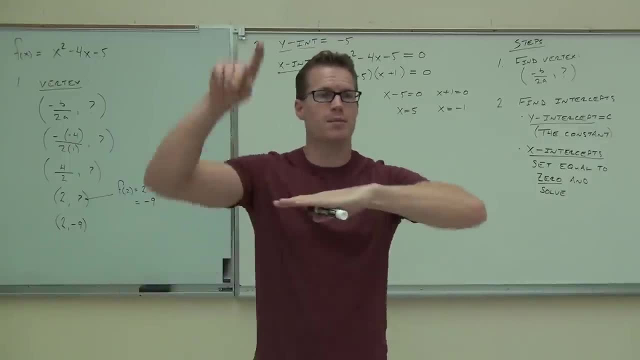 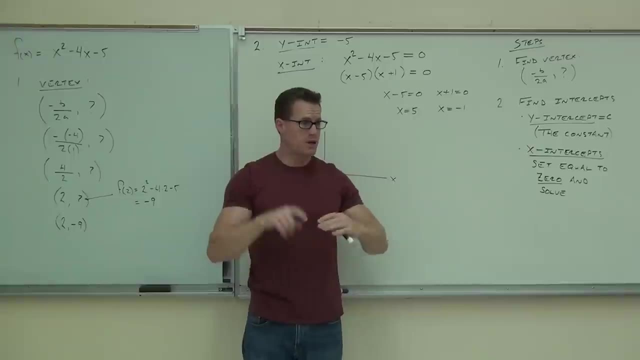 You don't necessarily have to have them in every parabola. You could be above or below the x-axis, You could be right on the x-axis, like that This one. are we not crossing the x-axis, or are we crossing and coming back? 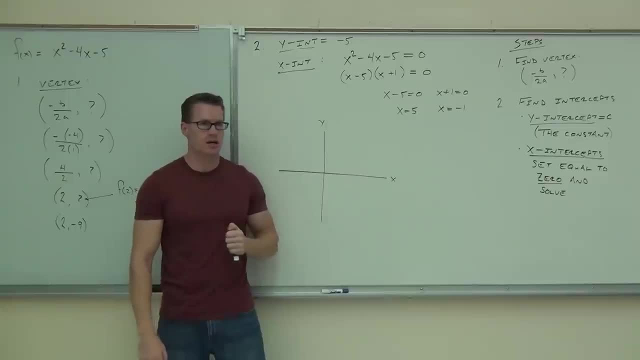 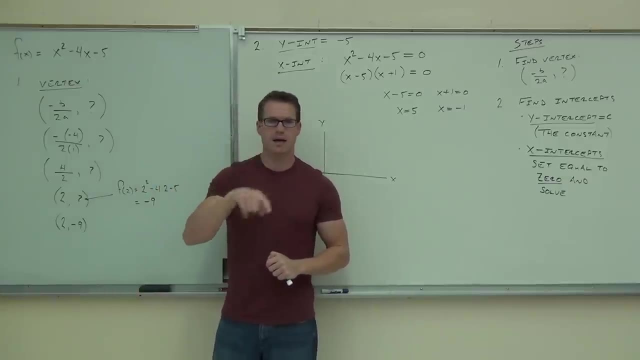 What do you think? How many solutions did you get? Two, Are you gonna be able to plot those on that line? Yes, So you cross that parabola. I'm sorry, you cross the x-axis and you come back at it. 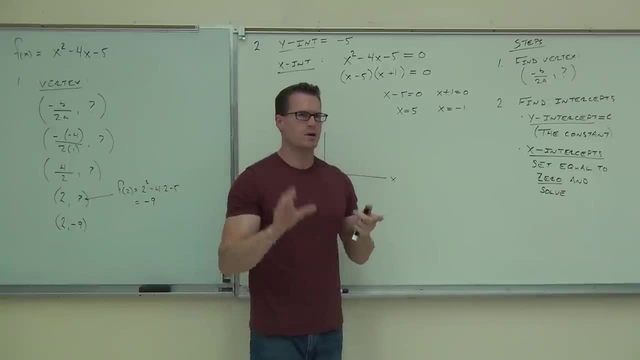 Does that make sense to you? Also, one more thing: Is our parabola going to be upward facing or downward facing, and how would you find that out? Upward, And how are you finding that out? Because there's no negative on the x. 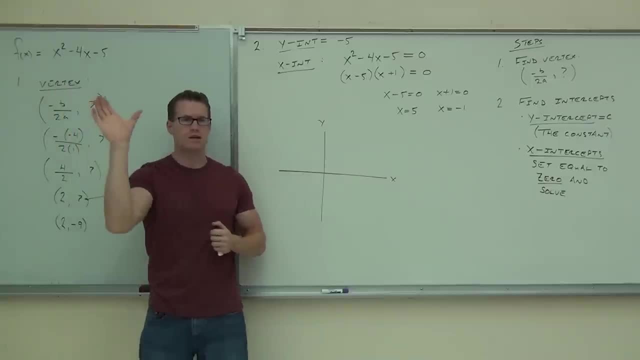 Oh good, so we look right here. Remember that a. That a tells you whether you're upward facing or downward facing. Also tells you whether it's gonna be a narrow parabola or a wide parabola. That still holds true. 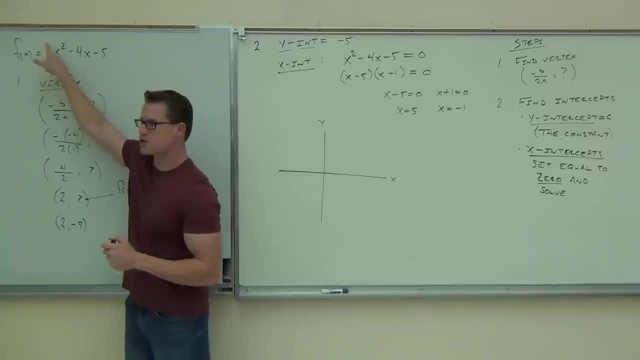 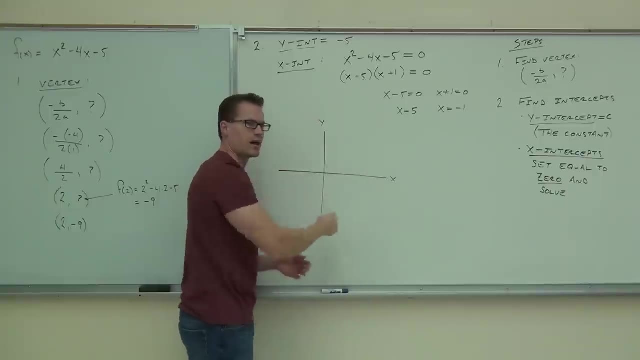 That's still true for us. So here is a normal-shaped parabola. There's no number besides one. It's positive. It should be upward facing. So we should get some graph that looks like this somewhere out of that, And it's good to think through that. 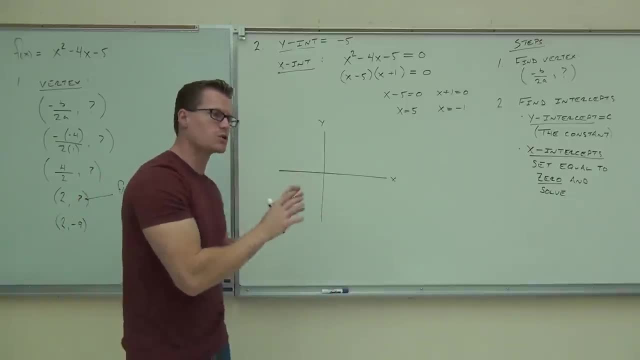 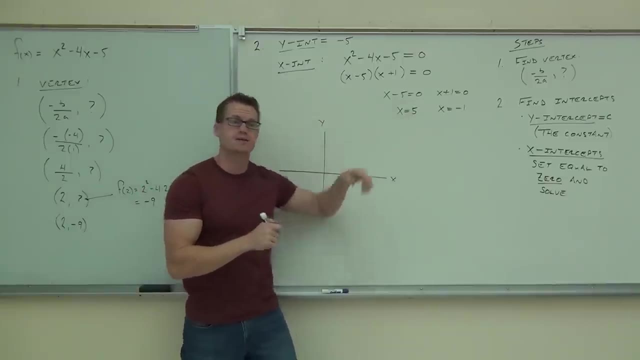 before you actually start your problem. So we'd be thinking about that. We know what we're supposed to get. Let's see if we in fact get it. Firstly, are you guys okay, getting to this far on this problem? Okay, so last step: we're almost there. 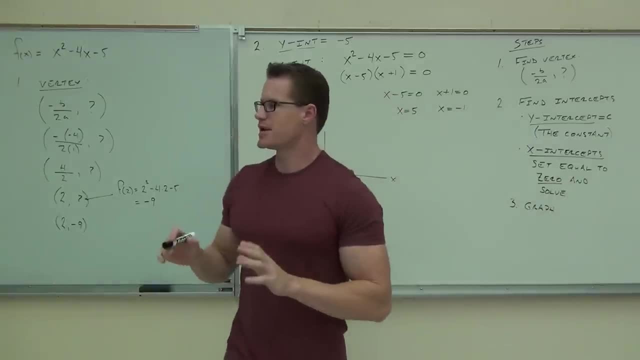 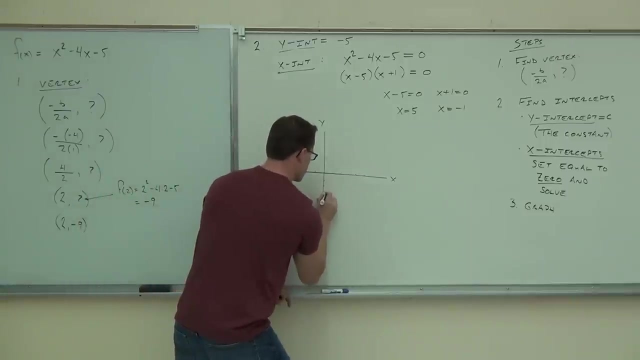 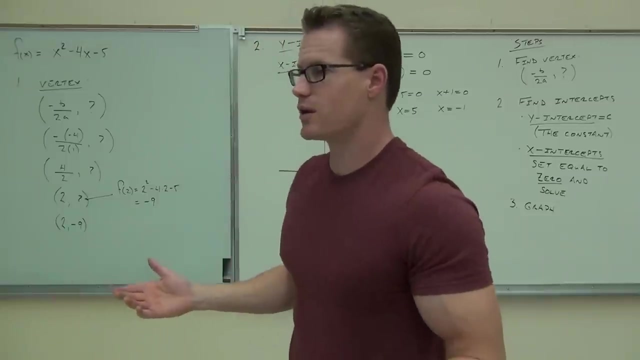 You can graph it. How we graph it is the same exact order that we did our steps in. Make these graphs nice, though Make them nice and neat. Hey, if you can plot points, you can graph these parabolas. So let's look back at our vertex. 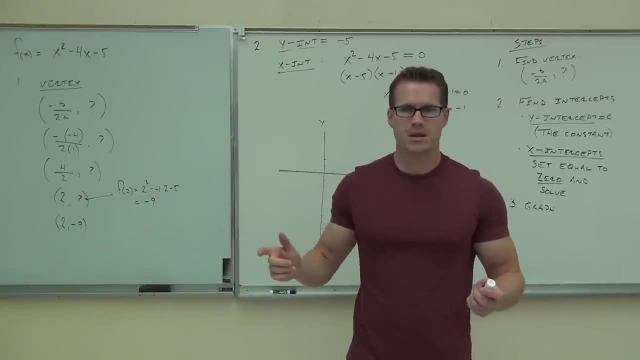 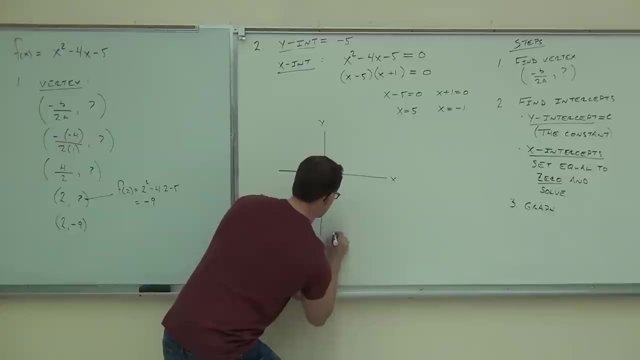 What's our vertex, ladies and gentlemen? Two, What was it? Two, Plot that point right now on your graph. So 2, negative 9, that's down here. Hey, just thinking back. should this be the lowest or the highest point of my graph? 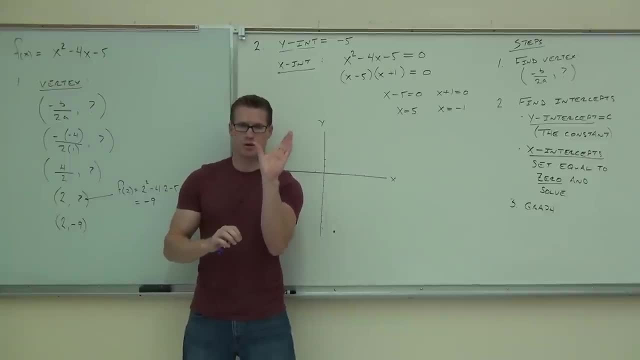 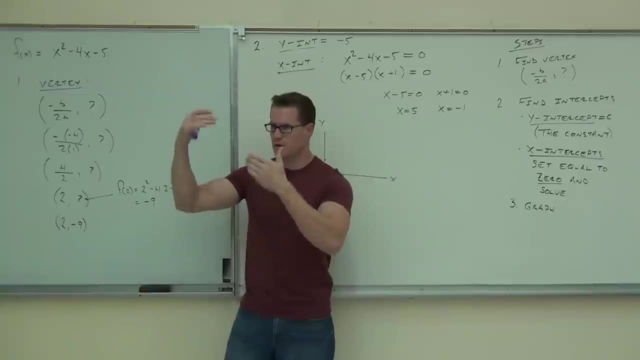 Lowest Because it's upward facing. you're right, That should be the lowest point of my graph. Now the next thing you do: you plot your y-intercept. So we're going in order: step one, two, three, all the time. 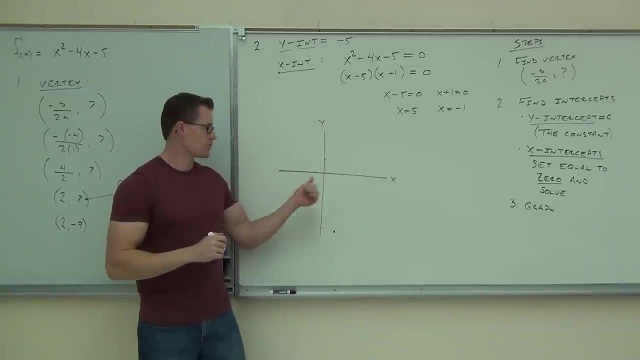 One, two, three. What's our y-intercept? So from here? From here, am I going to go up 5 or down 5, or left 5 or right 5?? What's my y-intercept? mean Down 5.. 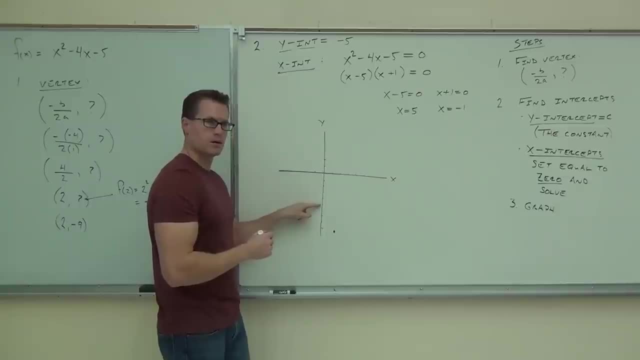 So one, two, three, Right here. Wait, is that 5?? Yes or no? Yes, Is that 5?? Yeah, I counted 5.. One, two, three, four, five. I tried to count 5.. 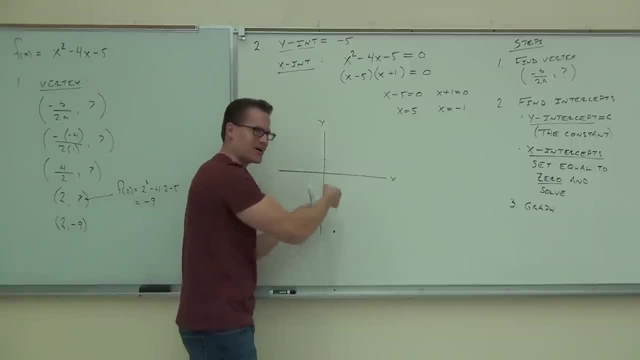 If this is 5, is this right? Yes, OK, good, This is down 5, negative 5.. y is negative 5.. This is the y-axis. go down to negative 5.. You OK with those ones? Yes, 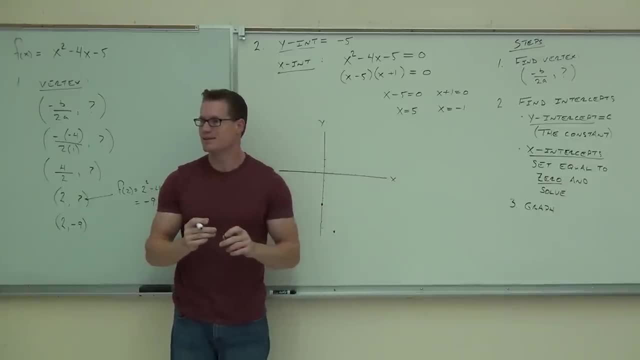 I'm not trying to trick you here. I'm just trying to make sure that you get this in: What is a y-intercept? What is it? y-intercept tells you where you cross the y-axis. So this graph must cross this axis right at that point. 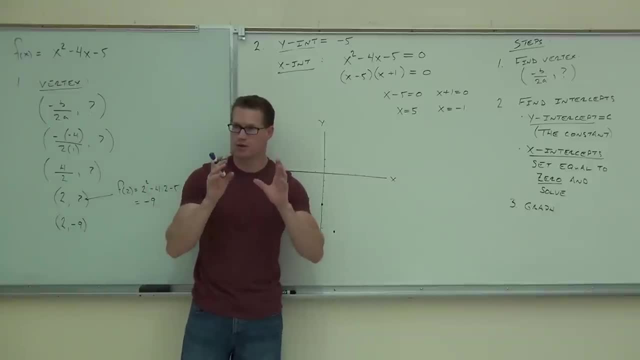 If you have it below there or above there, it's wrong. You need to have it crossing exactly at that point. Are you with me on that? So you're going to be able to graph these with only four points: vertex y-intercept, which you will always have. 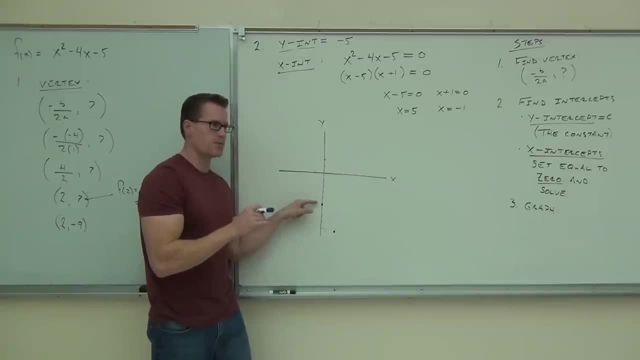 maybe even two points: Vertex y-intercept, which you must always have. then you're also going to need the x-intercepts, if they exist. So are you OK with the vertex? Raise your hand if you're OK with the vertex. 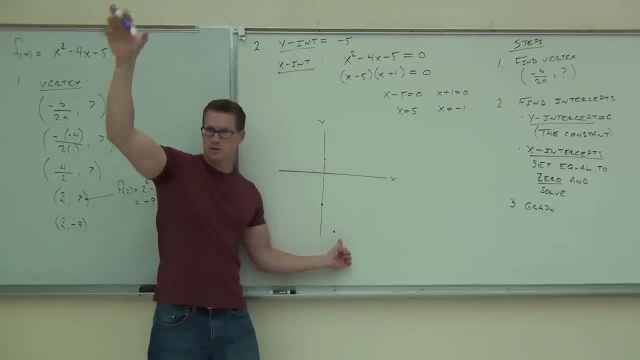 How about the y-intercept? Are you OK with the y-intercept? Yes, no, Yes, no, OK, The last thing we graph is the x-intercepts. Now, you might not have x-intercepts all the time If you were reversed this way upside down you. 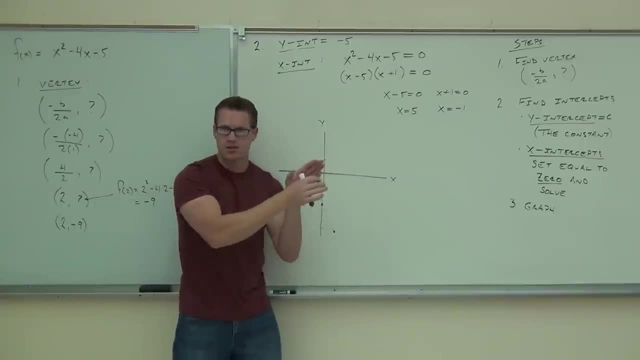 wouldn't have any x-intercepts. We're going this way, so we must have some x-intercepts. The factoring gave it to you and the factoring hadn't worked. the quadratic equation, the quadratic formula, would have given it to you. 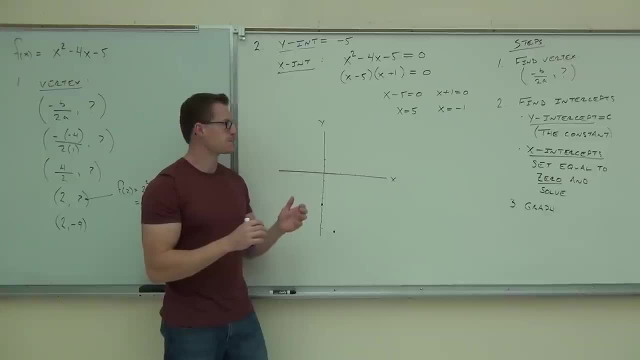 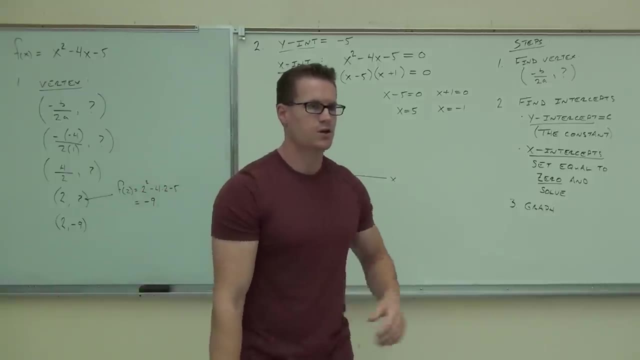 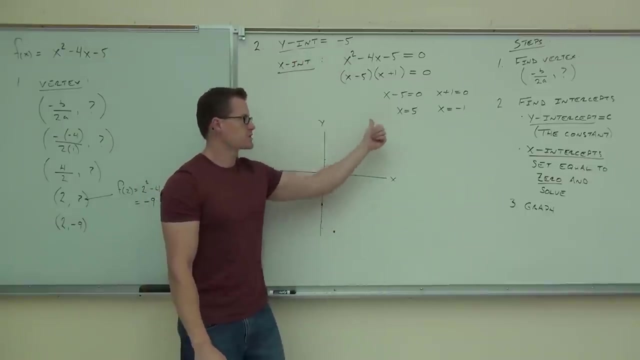 What are my x-intercepts? I want you to plot those right now on your x-axis. So y equals says you're going to the y-axis, negative 5. You, OK with that. one x equals says you're going to the x-axis. 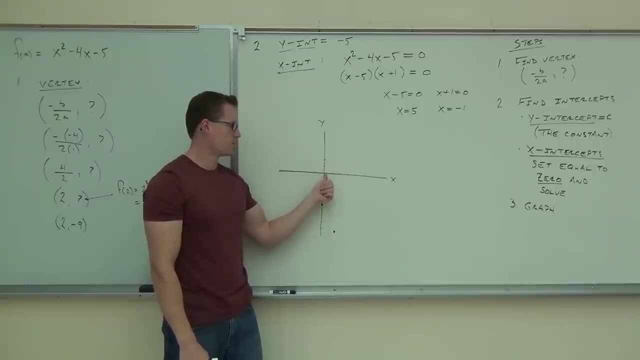 Put those points on there. Where's negative 1, left or right from my finger? No, How many 1.. Yeah, that's negative, 1. Negative, 1.. Where's 5?? 5. Right, 5.. 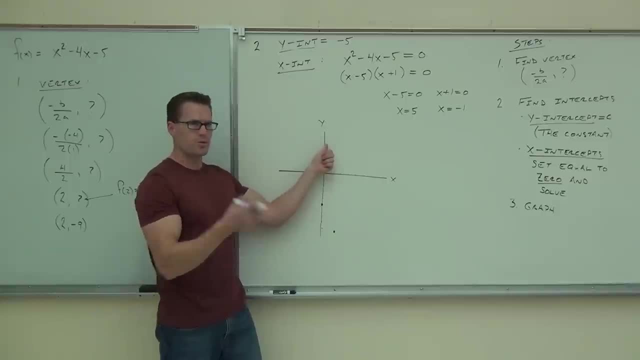 It's at 5,. yeah, it's at 5.. Is it up here at 5?? No, That would be y, right? No, we're talking about x. Hey, is it important for you to know how to factor? 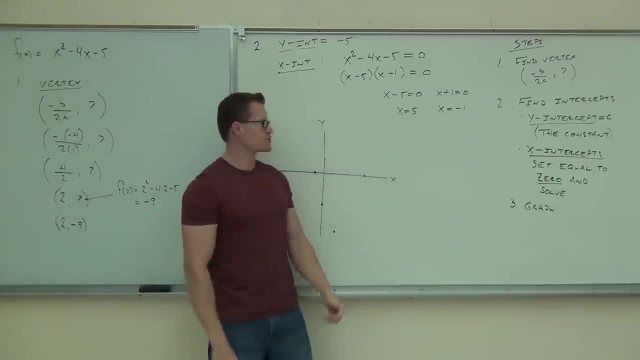 What if you get your signs wrong? Is this problem going to look right? No, If you get your signs wrong, you know what You're going to have: 1 and negative 5. You're going to be like: ooh. 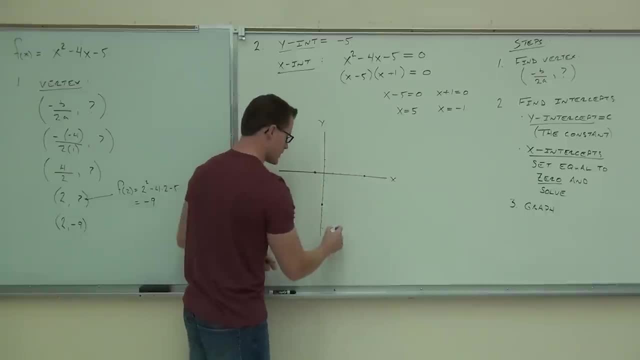 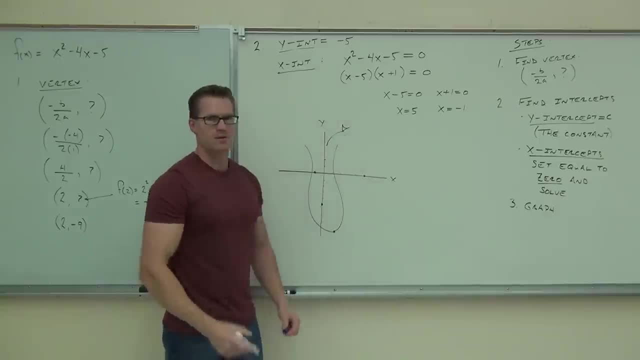 Hold some flowers. That's my flower. Good thing I'm not a florist. No, no, no, We've got to make sure we can factor, because that factoring was really the reason why you factor should do this. That's it. to get down to this far, to make sure you could go in. 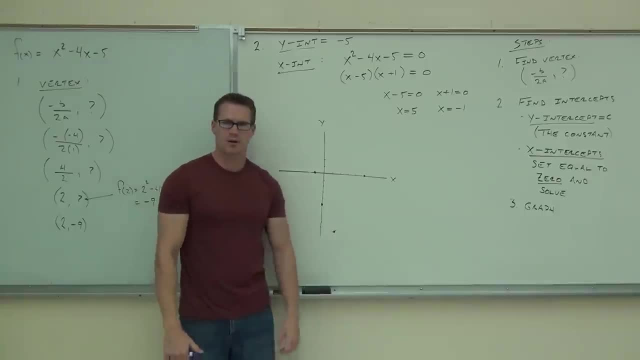 f for this far. that's it to get down to this far, to make sure you could go in find your intercepts here. So can you draw me the parabola from this picture? Do you see it? Can you see it visually? Can you see how it's going to look? 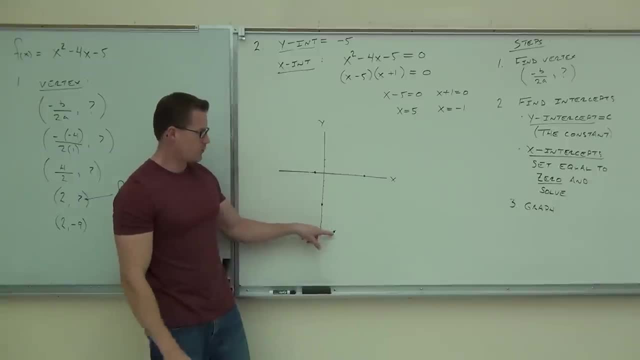 Here's what you do: You graph the side of the y-intercept first. The reason is because this has more points, right? This is a little bit more accurate than this side. This has just two points. This has one, two, three points on this side. You're. 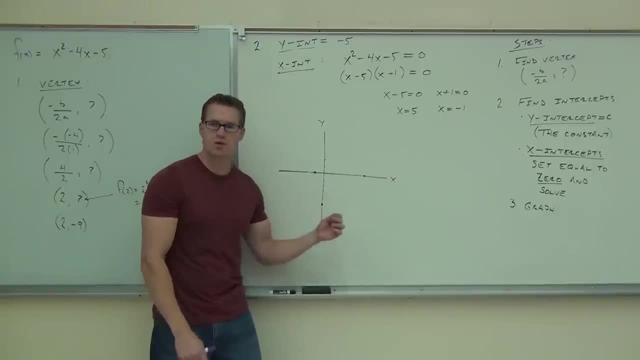 going to do this side. first, connect all three dots with a nice smooth curve, not straight lines- okay, Parabolas are a smooth curve. And then, because these things are symmetrical, do the same thing on the other side. So here we'll go: nice smooth curve. 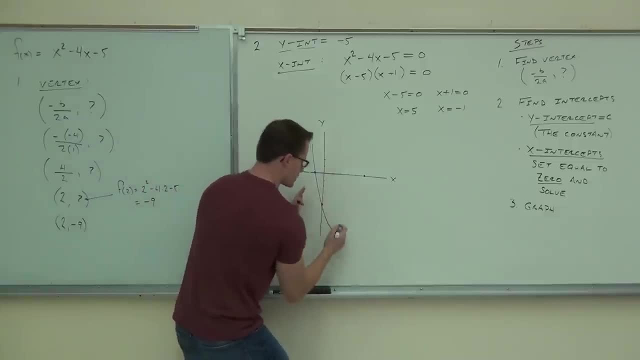 Isn't that pretty, Not bad? And then we're going to draw the same curve on the other side. Try to make the bottom of this curve. it's not a V, okay, It doesn't come to a sharp point, It's a nice curve. And then, of course, you label this with your name. 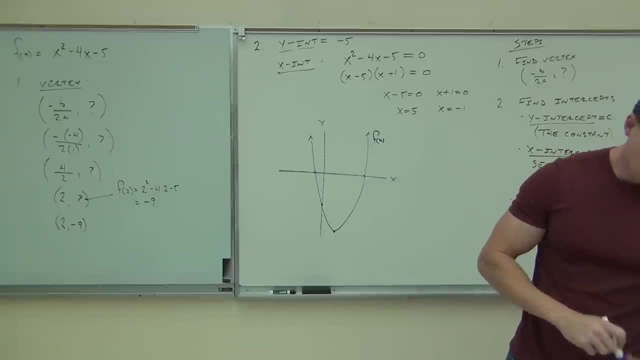 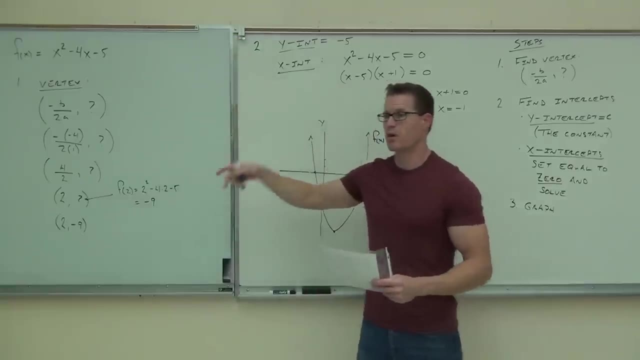 of your function, f of x in your deck. Would you raise your hand if you feel okay with this? So far, Okay. so vertex, no problem. Y-intercept- got it. X-intercepts: that's something we've done before. It's awesome. We just have the problem on the graph when 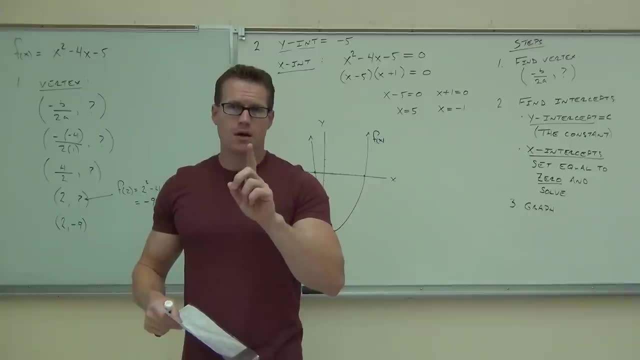 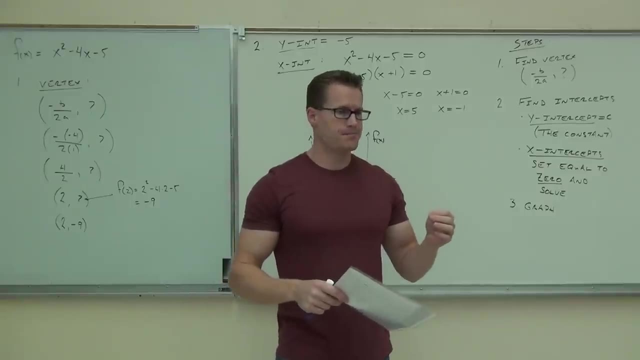 we're done, Let's try. would you like to try one more together? We'll do one or two more together. I'll show you one unique problem that we're going to make easier, And then we will have you do one of your own and be done. 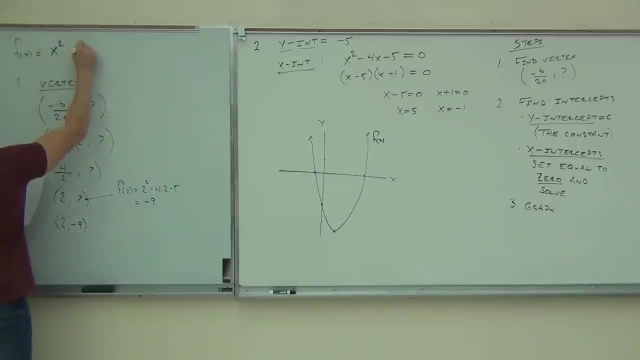 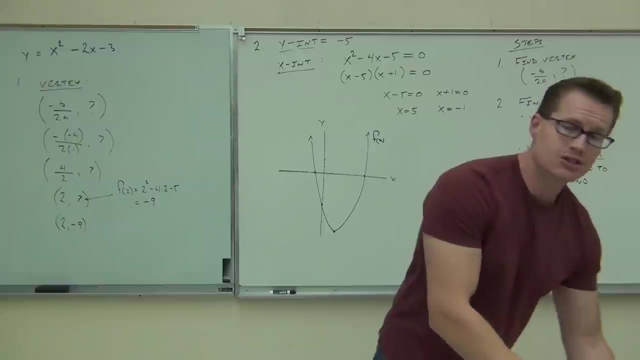 By the way, it doesn't always have to give it to you as f of x. It could very well give it to you as just y equals. Is that going to change what you do? No, No, y and f of x mean the same exact thing. Let's go ahead and go through this step by. 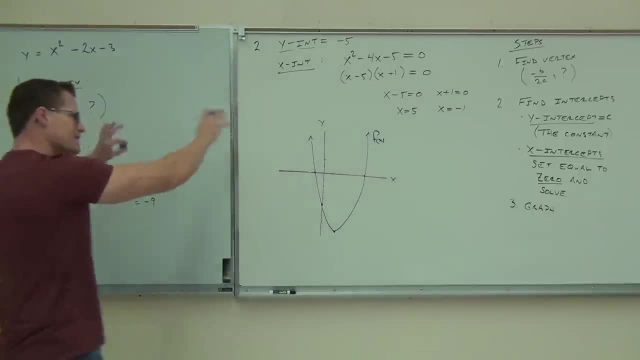 step. We're going to move a little bit quicker though this time, because we've already kind of had the concept down. So, first thing, what is your first step? I've left this on the board, but what is your very first step? What are you going to do? 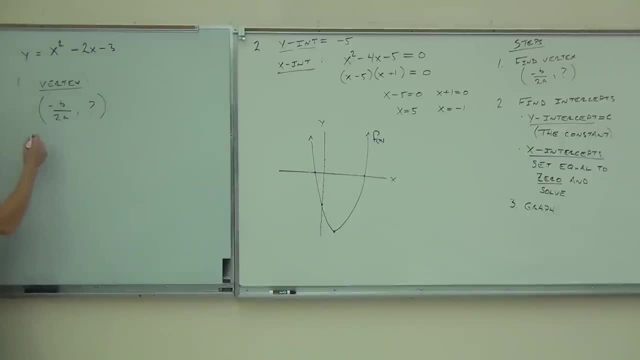 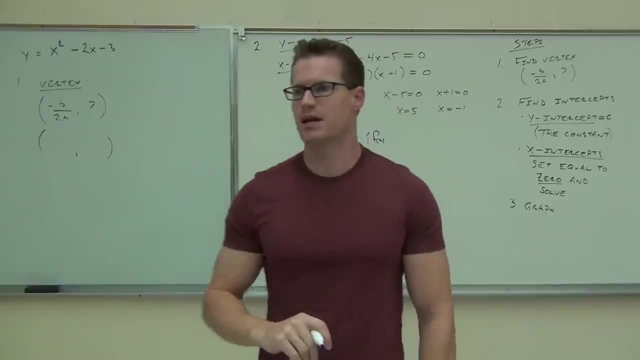 Okay, vertex, great okay. So negative b over 2a. what I'd like you to do right now- I'll give you about five seconds. fill out the formula. You don't have to do all the math, we'll do that together, but fill out the formula correctly: Negative b over 2a. 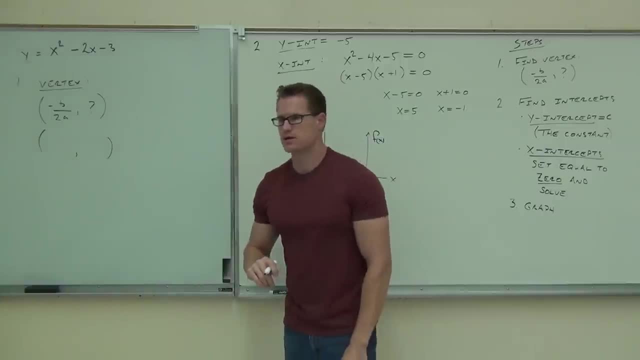 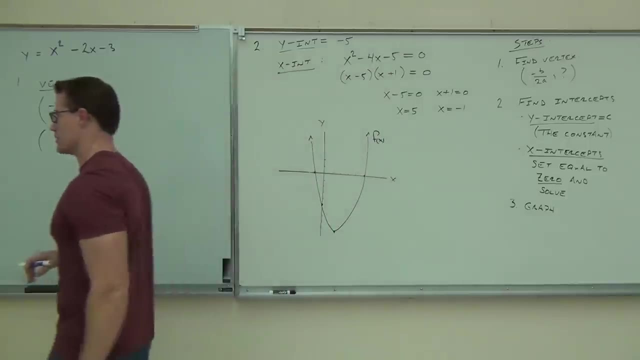 Firstly, what is your a One? It is one. What's your b Negative, 2a. What's your c Negative, 3a? You don't actually use that here until the y intercept, but you should know it. 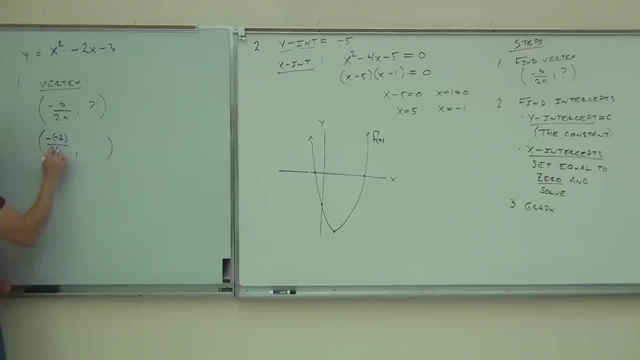 Did you all get that on your paper? Negative, negative 2 over 2 times 1? And then over here we got a question mark. We go: okay, I don't know how to do that, yet Let's do this math together: How much is negative, negative 2, folks. 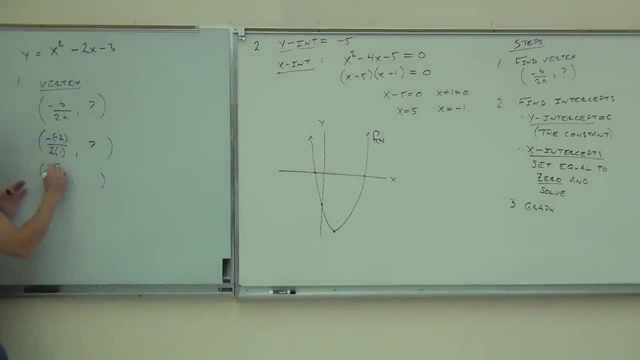 Two. So remember, we're plugging it in without doing any math and then we start doing it little by little, Two over Two. Oh, that's kind of nice. So we're going to get one comma something. One comma something. 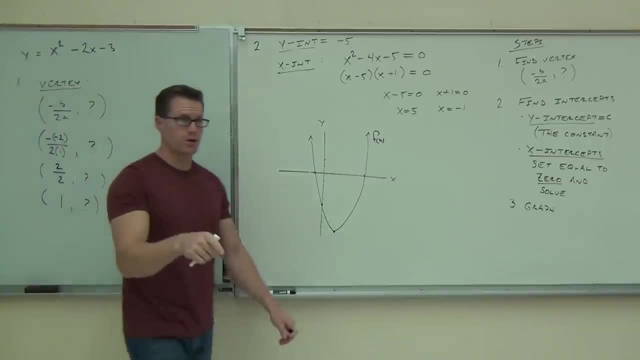 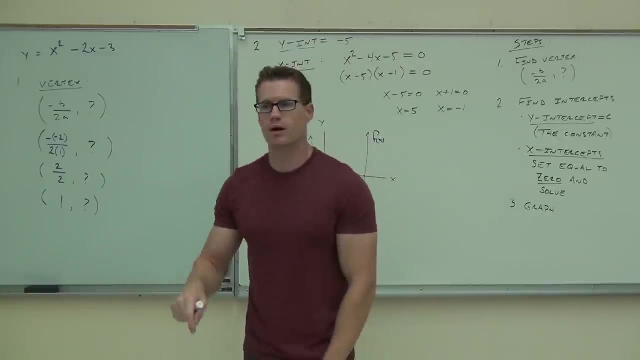 One comma, something y coordinate over there. Did you all get one on yours? Yes, What do you do with that one? We plug it in back into the original. Okay, do that right now, See if you can do it. Plug in that one and see what my y coordinate. 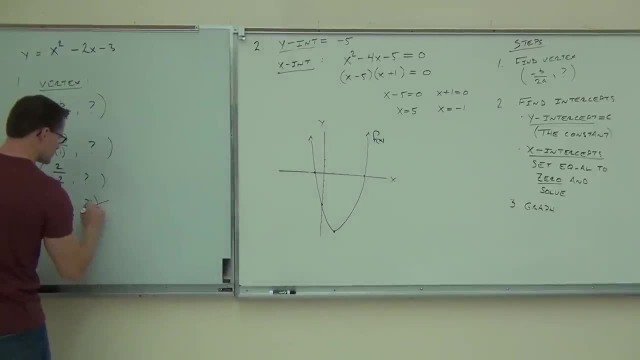 is going to give me. So you should have 1 squared minus 2 times 1 minus 3, and that's going to give you your vertex: One comma something, One comma something. It's a point. That's why we draw it as a point, to make sure we have that. 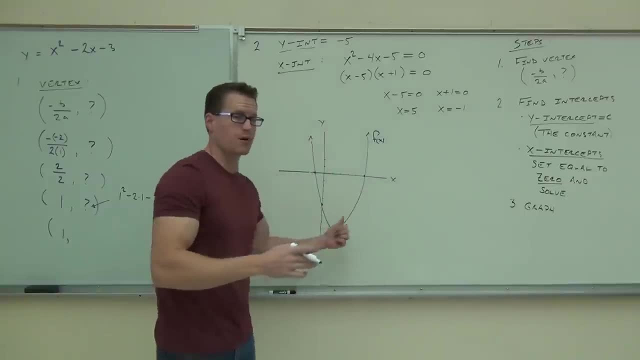 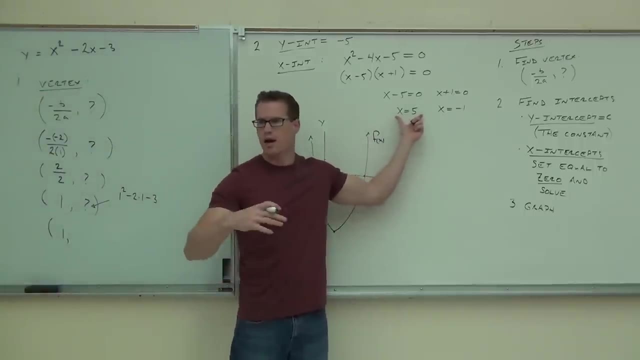 If you're giving me just a vertex of 1, well, you're not going to be able to graph that, But you have to have a point to graph. The x and the y intercepts are unique because you know they're on the x-axis or the y-axis. 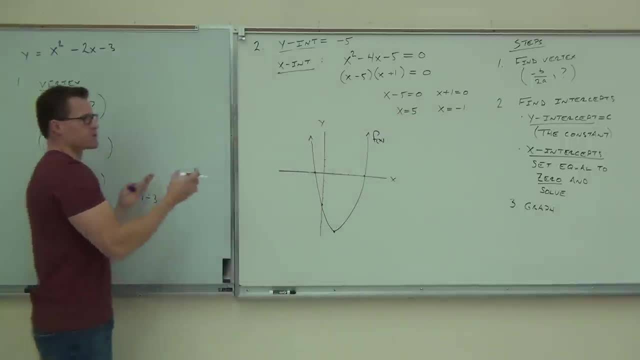 already. That's why you can have one point there, one value, But for the vertex you need both. What is 1 minus 2 minus 3, and which is that Negative 4.. How many people found the negative 4 out of that? 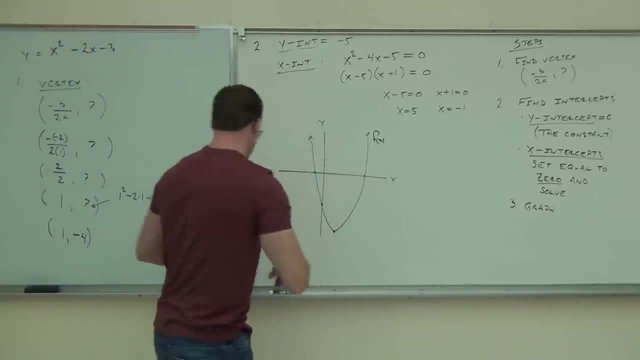 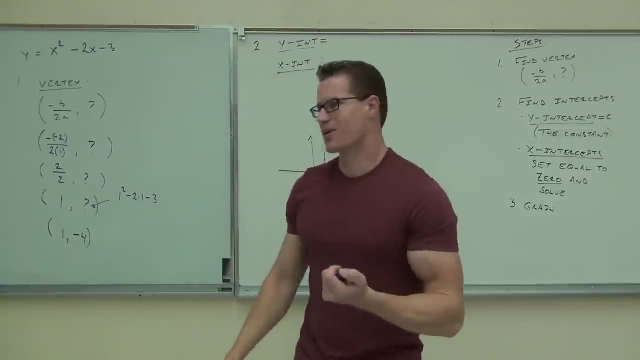 Okay, good, So we got our point. Next up, we're going to look at the y-intercept, So y-intercept right now. Man, this is the quickest part, This is the awesome part. Everyone should get this one right. 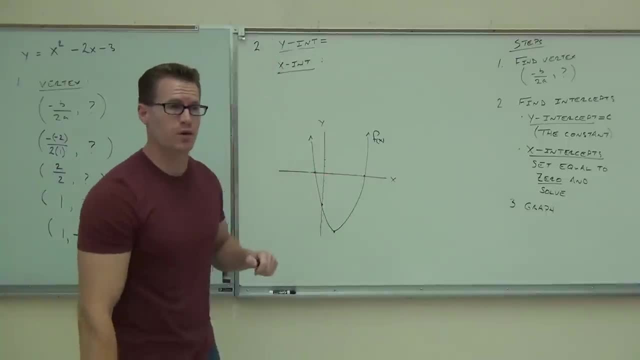 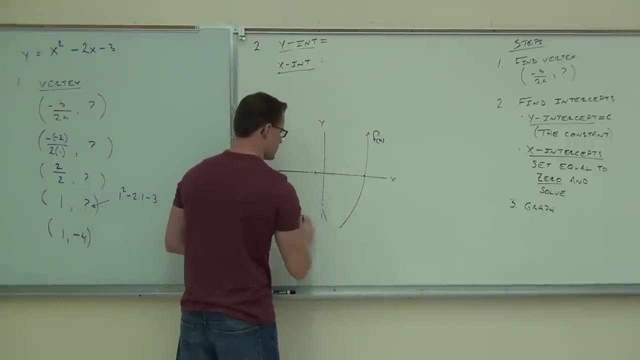 Go ahead and find your y-intercept right now. Don't say it out loud, but write it on your paper. okay, Do the y-intercept now. What's the y-intercept here, folks, It's kind of nice right. 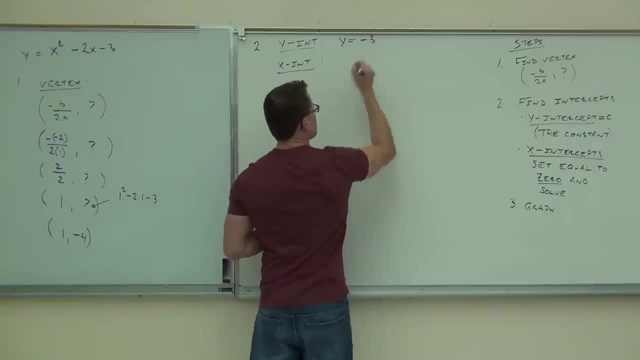 Just that constant off to the back end with a sign. By the way, should our parabola be upward-facing or downward-facing here? Can you tell me that? Should it be narrow, wide or normal, Normal, Normal, Good. 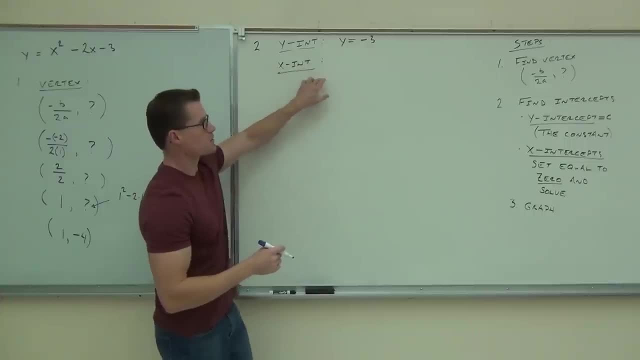 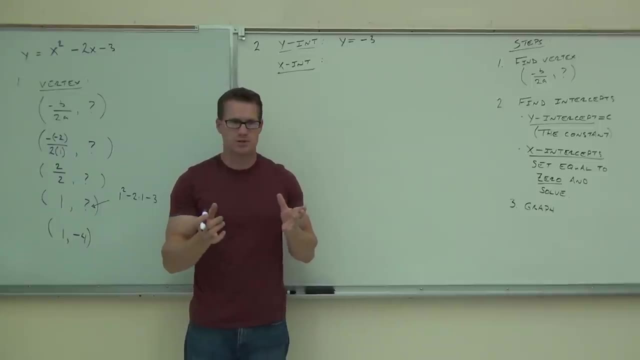 Upper-facing, normal-looking parabola is what we should get out of that. Now the y-intercepts are easy. X-intercepts take a little bit more work. What are you supposed to do with your x-intercepts? How are you supposed to find your x-intercepts? 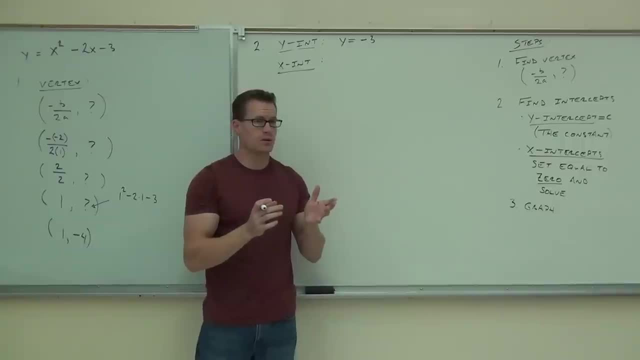 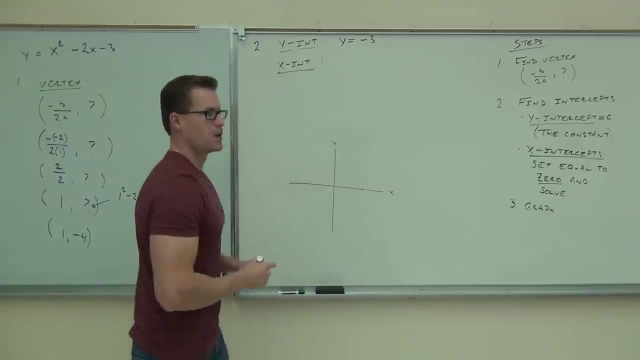 Set what equal to 0? Zero, Zero. Okay, Go ahead and do that. now See if you can factor, If you can great, Solve it all the way down for your x-intercepts. Go ahead and do that, So when you're solving the x-intercepts. this really is old, old stuff. 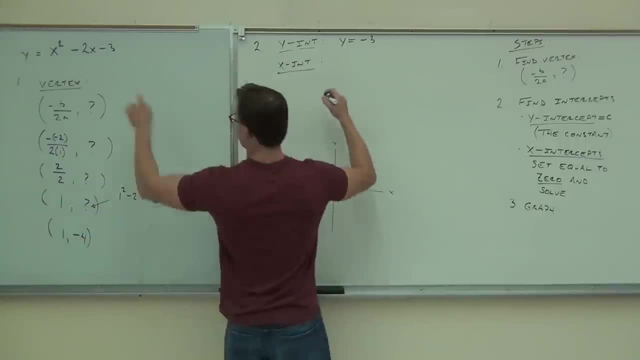 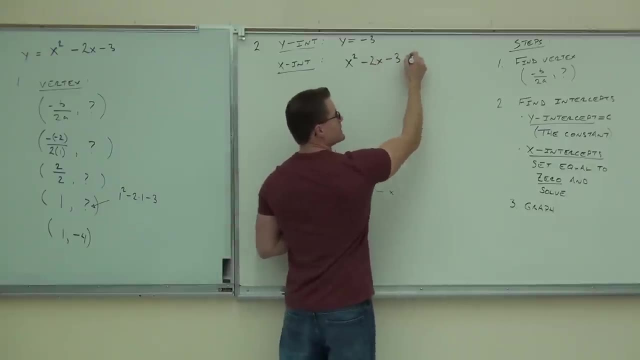 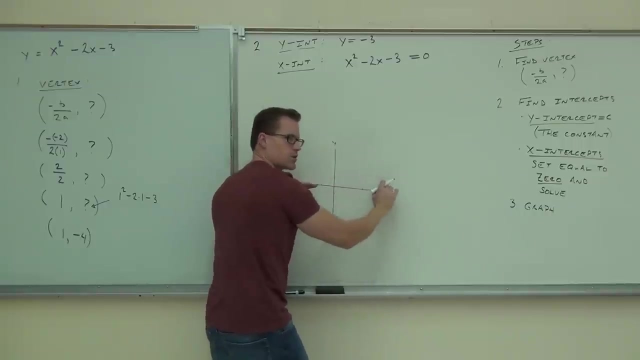 And we have literally been doing this the entire semester. You take your original equation, the quadratic part x squared minus 2x minus 3. We set that equal to 0. And what we're trying to do here is find out the values that make the y equal to 0.. 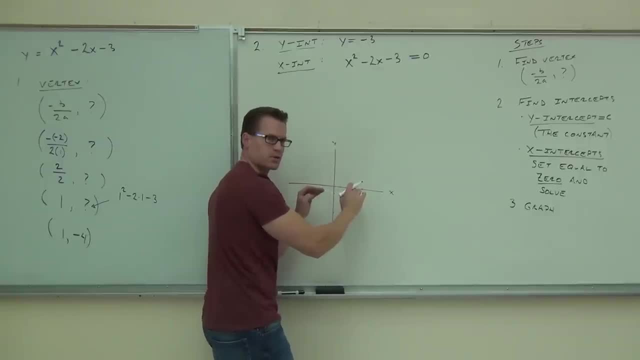 That means the values where you're crossing the x-axis. Are you following me on why we set that equal to 0? Level is 0, right here. That's where we're trying to find those points. Then we try to factor. If we can't factor, if we use quadratic formula, we'll give you the same numbers. 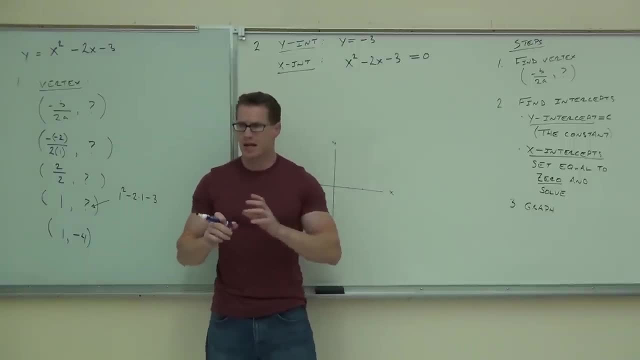 By the way, if you get the quadratic formula and you can't figure out the exact numbers, like the square root of 13 or something, we get that sometimes right Like 1 plus or minus the square root of 13 over 2.. 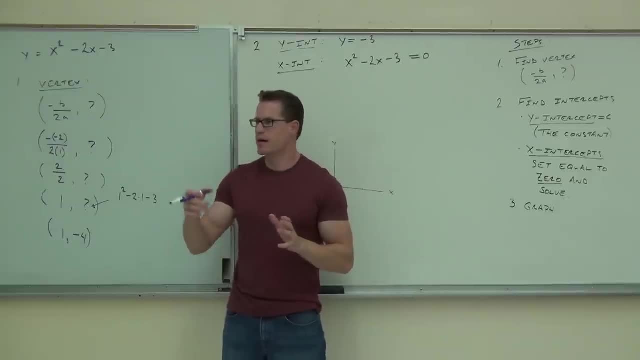 Use your calculator. Approximate that. Take 1 minus the square root of 13 over 2.. Take 1 plus the square root of 13 over 2. And figure out the decimal approximation to graph that. Are you with me on that? 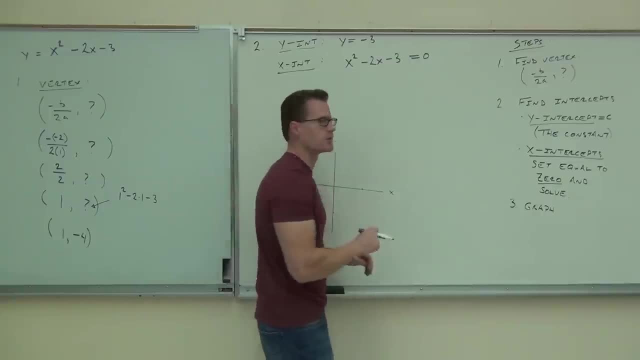 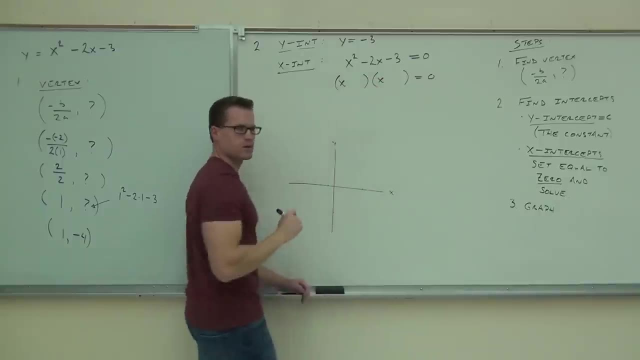 So quadratic formula will still work. You might just need your calculator Here. fortunately for us, we don't really have to use that. We've got some factoring that's involved. We've got x and x. What's it going to be? 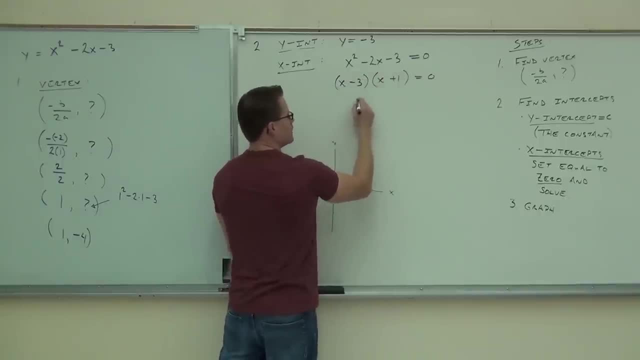 Minus 2.. Of course, you take that a step further. You don't want to do this right. You don't want to put negative 3 and plus 1 right here, because those signs are going to change when you set them equal to 0.. 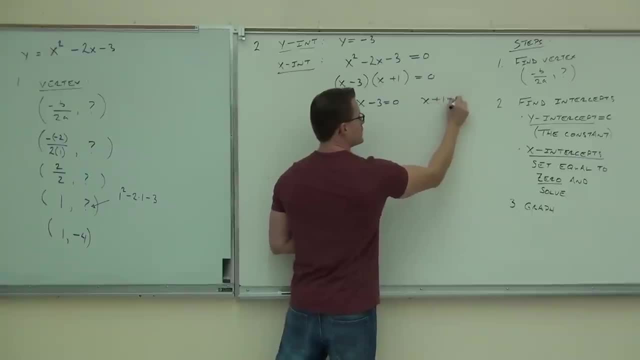 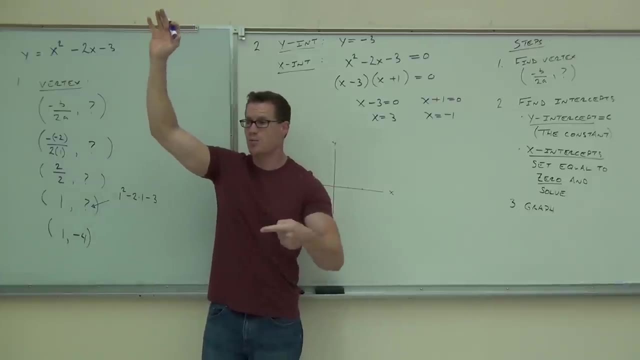 Minus 3 equals 0 and x plus 1 equals 0. So x equals positive, 3. x equals negative. 1. Raise your hand if you found that Great. Are you starting to see how important factoring is for you? 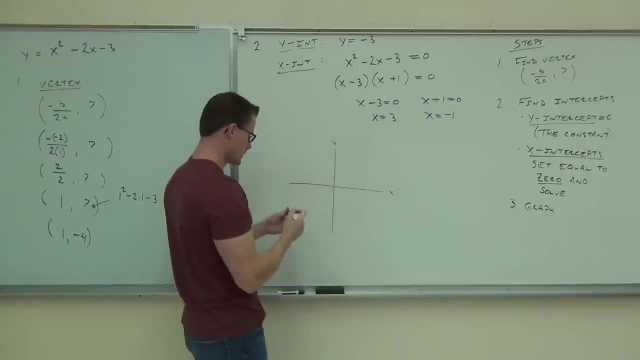 We really need it every step of the way through this course. Okay, so we're going to start from the very beginning. We're going to graph our vertex first. Go ahead and do that now, if you haven't done that already. Plot your vertex. 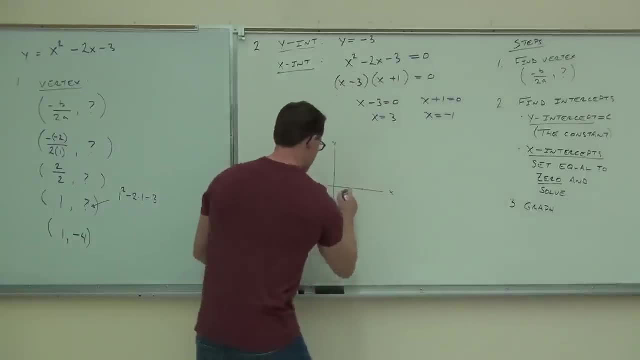 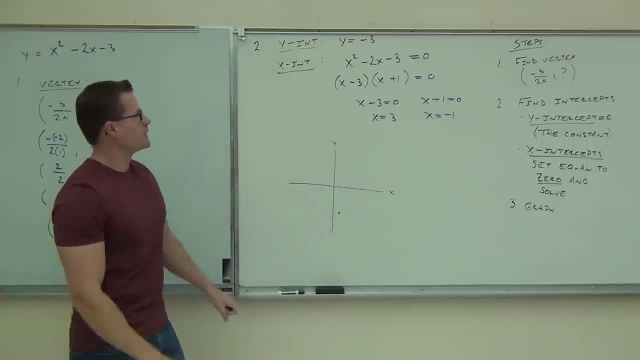 So vertex is 1, negative 4.. In this case that will be the lowest part of my parabola because it is upward facing. What's our y-intercept? Go ahead and plot that, if you haven't done that already. 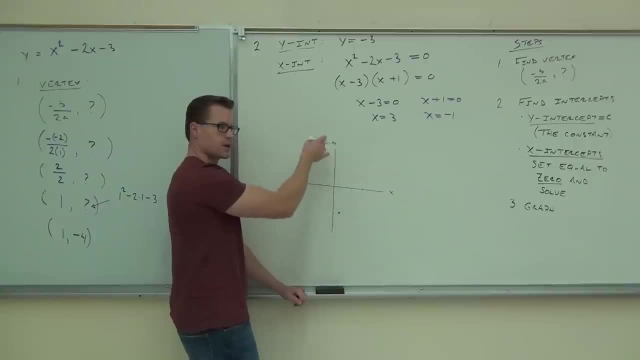 So negative 3, that says you're on the y-axis, You're going up or down. Definitely down. Negative right here. Last thing: we have our x-intercepts. Go ahead and plot those if you haven't done that already. 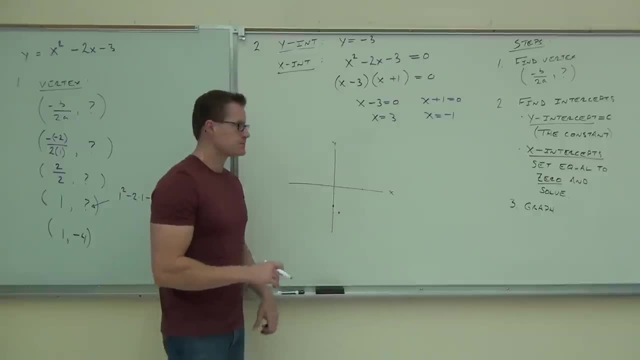 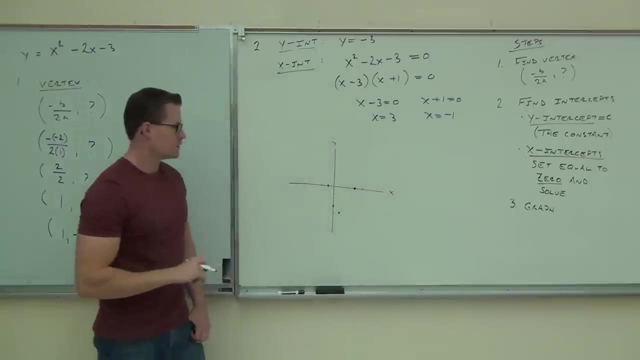 We've got x equals 3 and x equals negative 1.. We're going to do this again. We're going to do it again. We're going to do this again. Let's try this. Does it look like how it should look? 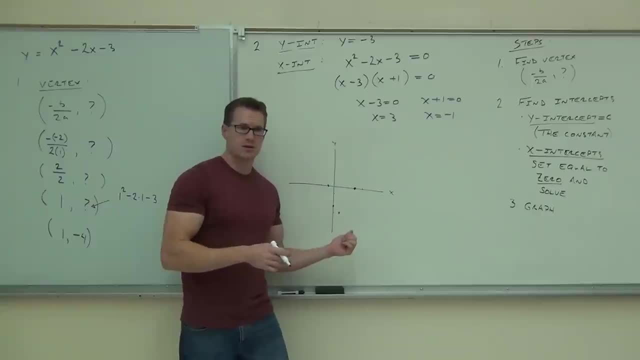 At the very beginning we said it's going to be an upward facing parabola. Is it upward facing? Good? If you got downward facing, you probably did something wrong. right Yeah, Is it really narrow or really wide, or is it more normal looking? 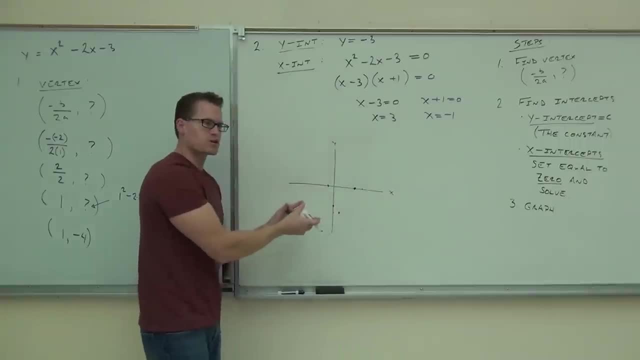 Normal, More normal, And it should be normal looking. So this is probably the appropriate picture for us. We know we did all the work right, so we're going to do the appropriate thing. We're going to graph the left side first, because that's the side that the y-axis is on. 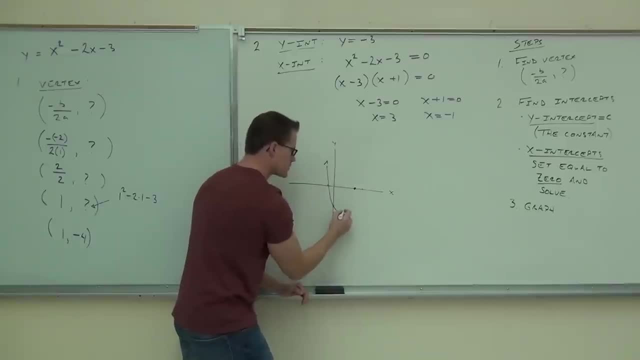 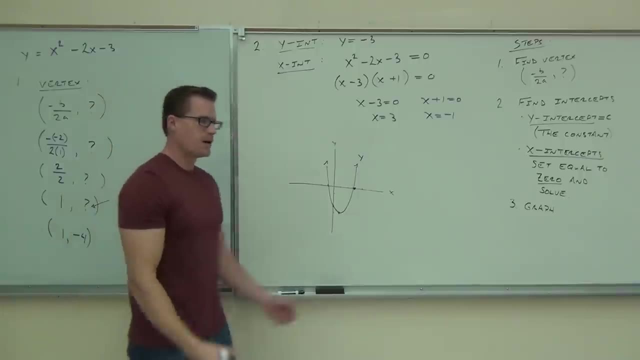 So we're going to graph here. We'll make it symmetrical, Label it. In this case, that's just the graph y. That's a perfectly good parabola. It's much more accurate than those shifting that we did last time. 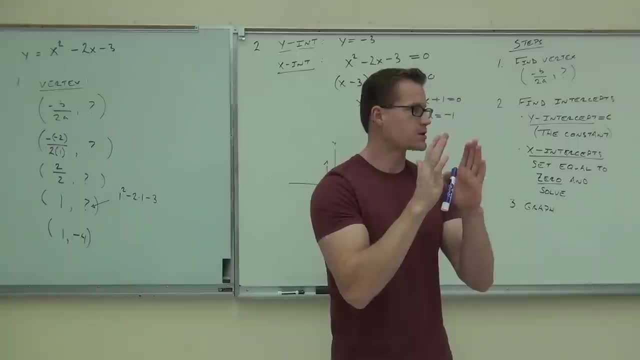 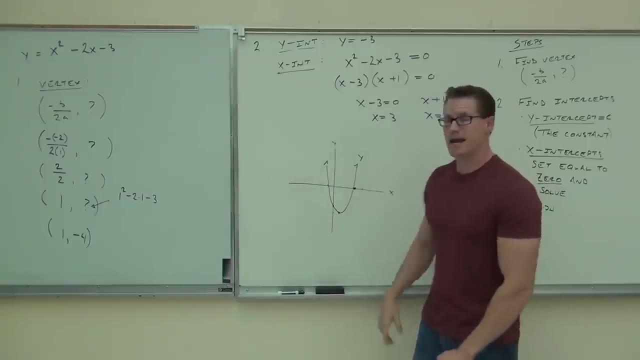 The shifting. we didn't know really exactly how wide or narrow it was. We didn't know exactly what these looked like. right, We didn't know exactly where it crossed the x-axis. Now we do. That's a pretty accurate graph for only doing maybe five minutes. 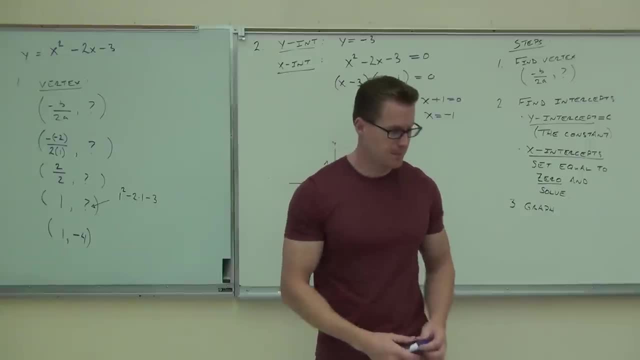 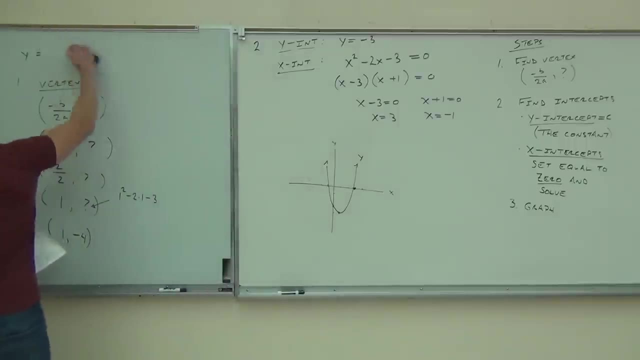 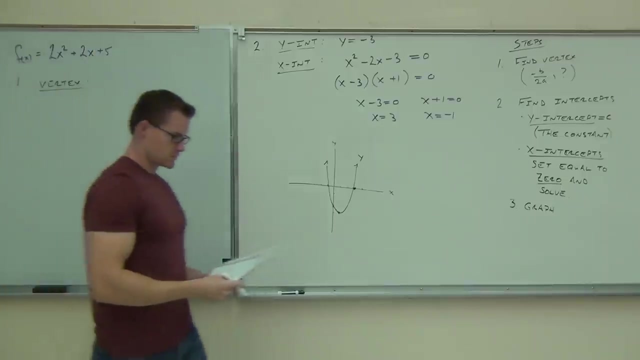 of actual work, right, Not too too bad there You ready to keep going? Okay, let's get started on this one First thing we've got to do: we've got to find the vertex. So what I'd like you to do right now is plug. 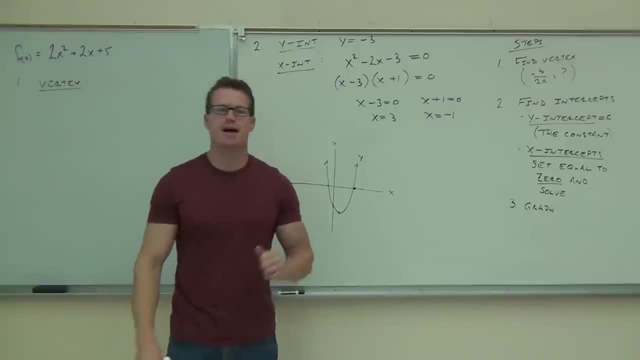 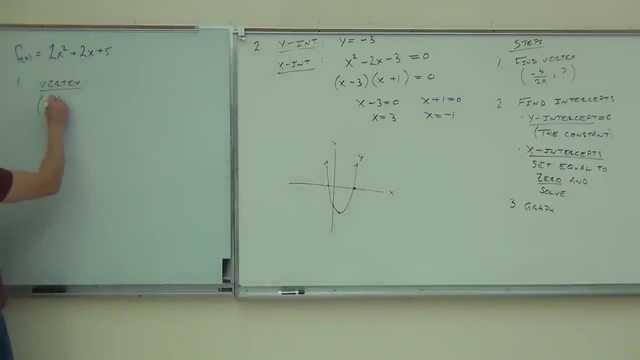 in those numbers for the vertex, Work it down and find the x-coordinate. We'll do the y-coordinate together. Go ahead and do that on your own, as I'm doing it up on the board. Why, What'd you get for your x-coordinate? 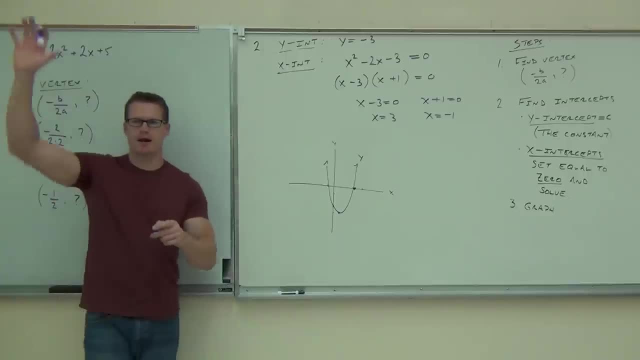 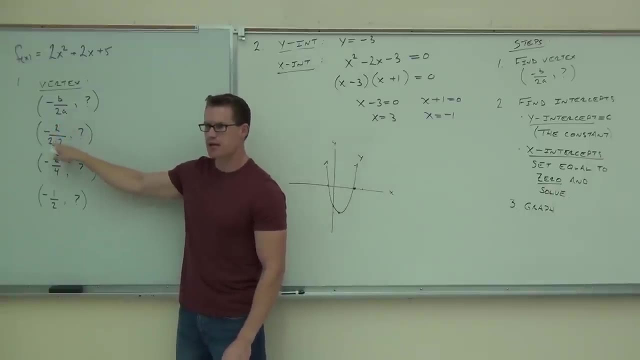 How many of you have gotten negative 1 1⁄2,, negative 1 1⁄2?? Why did we get negative 1 1⁄2?? Well, we got negative 2, that's our b right over 2 times a. 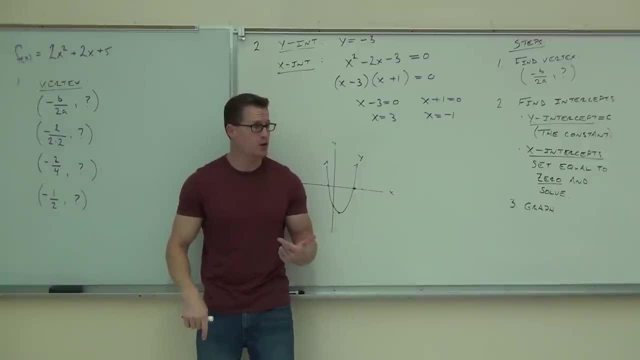 Don't forget about your a. Your a is not always 1.. In this case, your a is 2.. So do you see how we're getting the negative 1 1⁄2, folks, Are you sure you're with me today? 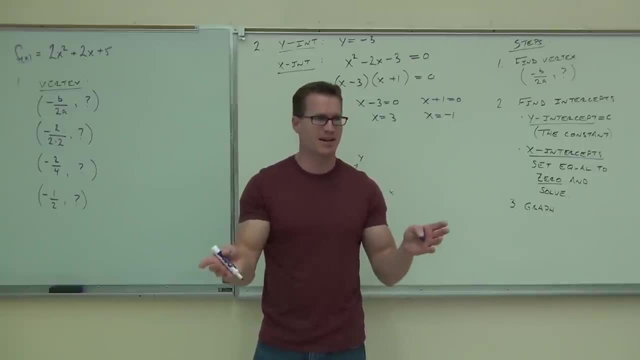 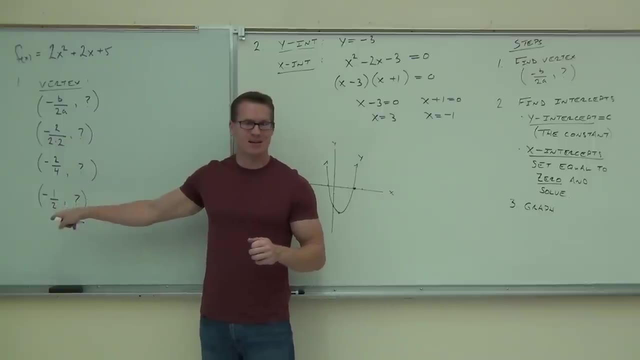 Some of you look a little sleepy. I'm, of course, way caffeinated today, so I'm the opposite of you who did it this morning. Anyway, are you okay getting the negative 1 1⁄2, yeah or no? Now we got a fraction, right. 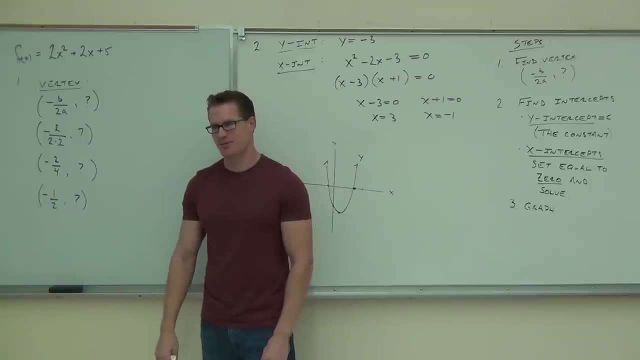 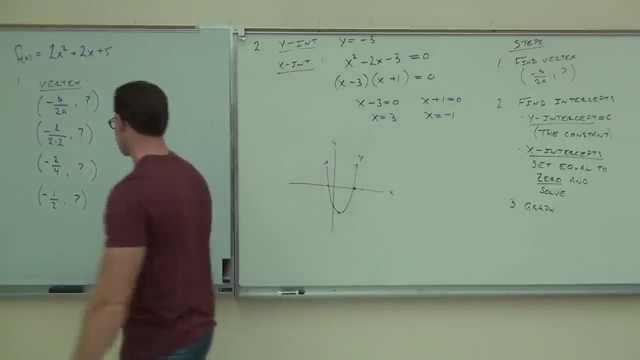 Fractions happen. It's not even Friday, We still got Friday. It's not even Fraction Friday. We got fractions in here. But that's okay. Can you plug in a fraction? Let's do that together. Watch what can happen. 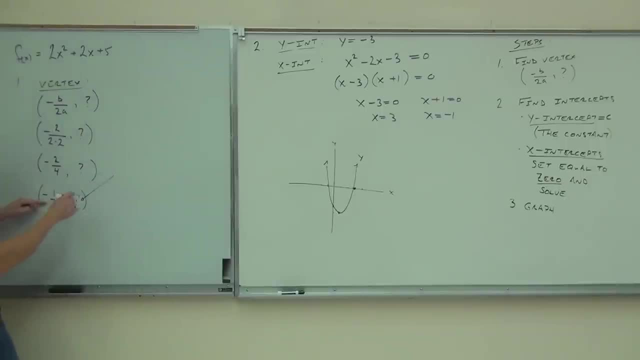 When you plug in this fraction, it says: take your negative 1 1⁄2,, just be careful with it. You got to do exactly what I'm going to do up here. We've got the 2 from the 2.. 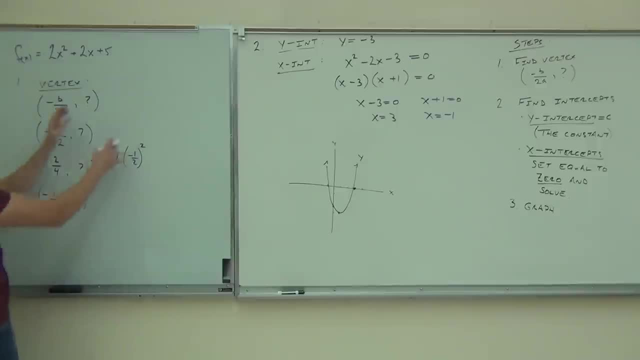 I'm going to put the negative 1 1⁄2 in parentheses. It's squared because there's lots going on. right, We got a fraction and we got the negative. Make sure we have the parentheses around now. Then I have a plus 2, but that's going to be multiplied again by negative 1 1⁄2 and 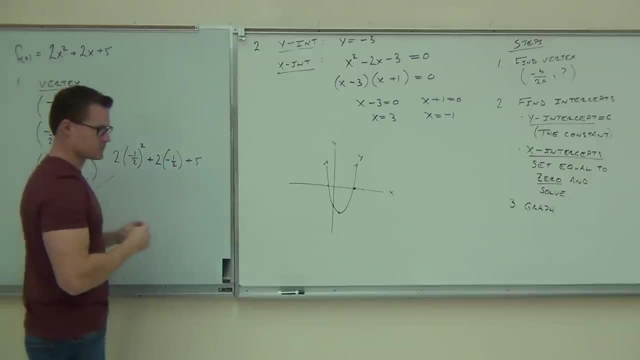 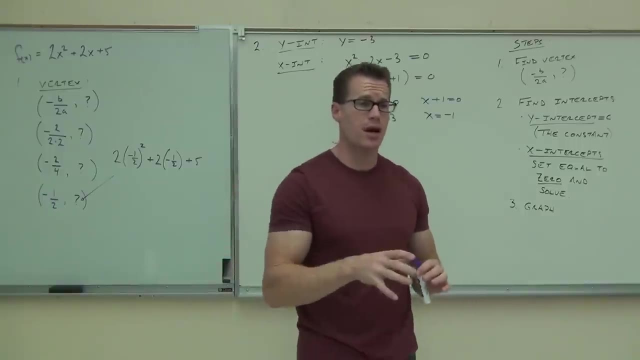 then at the very end, I have plus 5.. Now use your calculator if you'd like to, That's fine. I don't care if you do these fractions or you're headed with a calculator, Just make sure you get them right. So in our case, right here, we'll go down a little bit slower here. 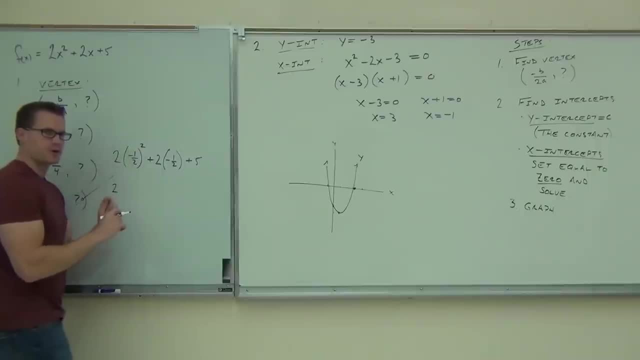 We've got the 2.. Can you tell me how much is negative 1 1⁄2?? How much is negative 1 1⁄2 squared, please? How much is negative 1 1⁄2 squared? 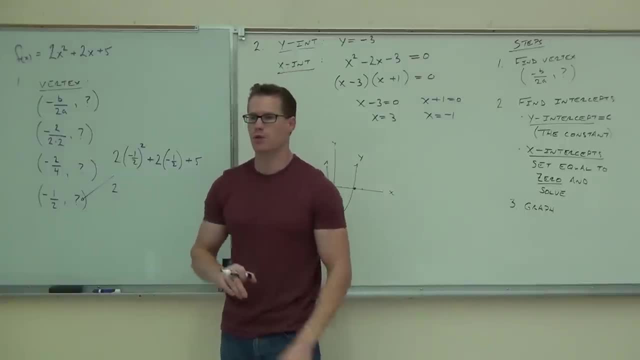 It's not 1.. That would be adding 1 1⁄2 and 1 1⁄2.. We're actually multiplying 1 1⁄2 and 1 1⁄2.. Well, you should know. 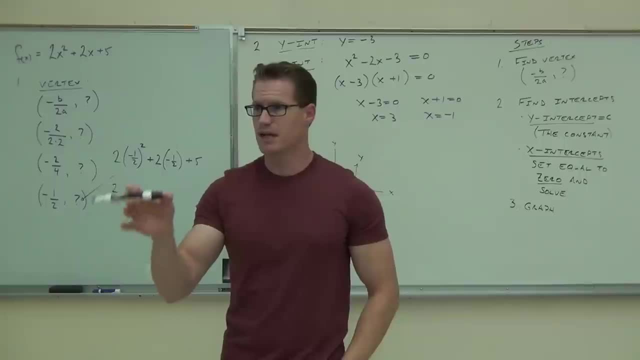 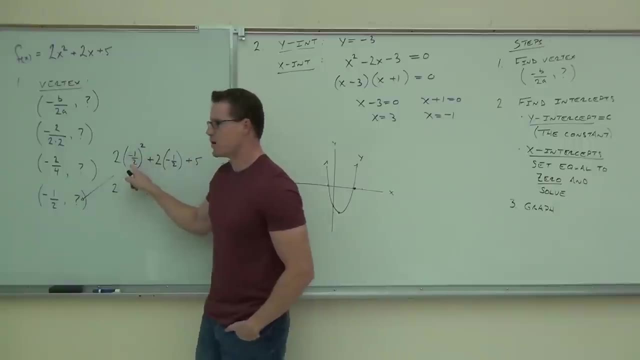 I mean, you really should. You should calculate it if you have to, but take negative 1: 1⁄2 and square it. It's definitely 1⁄4.. You square the top, you square the bottom, you get 1 over 4.. 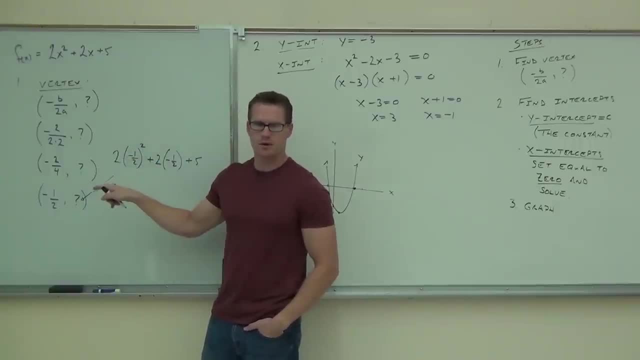 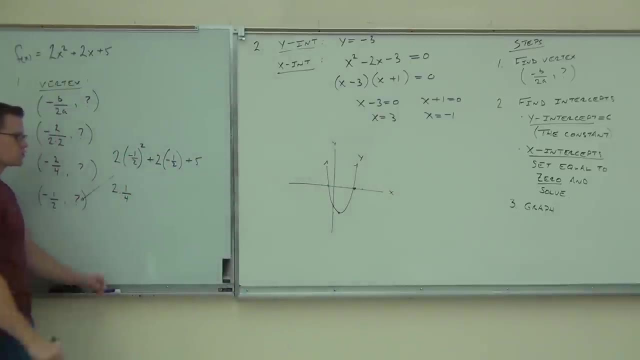 You with me on that. Is it positive or negative? Positive, Absolutely positive, Yeah for sure, Because we're scoring negative. So this is going to be 1⁄4.. So you have 2 times 1⁄4.. 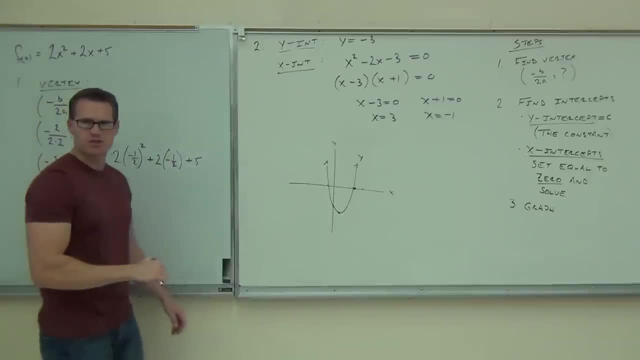 Now, what is this going to give you? 2 and then times negative 1⁄2? What's 2 times negative 1⁄2? How much is that Negative 1. Negative, 1.. So I should have a minus 1 and then a plus 5.. 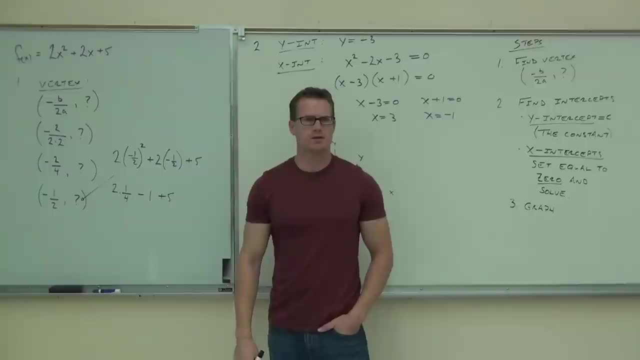 Give me the head nod if you're okay with that. so far, Okay. So this is fraction work. I mean, this is way what we should have down already, but I understand that a lot of you are not so great with fractions right now. 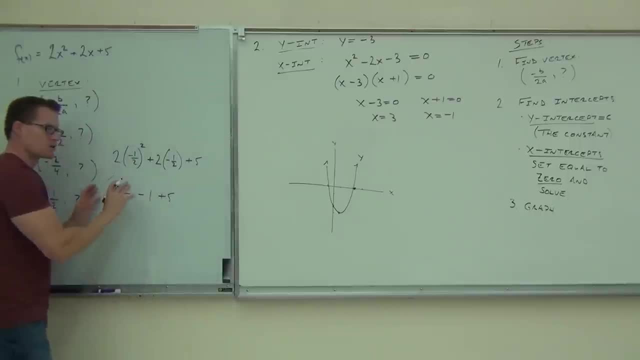 Maybe you need a little more practice, though That's okay, Just make sure that we're getting this part right. What's 2 times 1⁄4?? 2 times 1⁄4.. So this is going to be 1⁄2 minus 1 plus 5.. 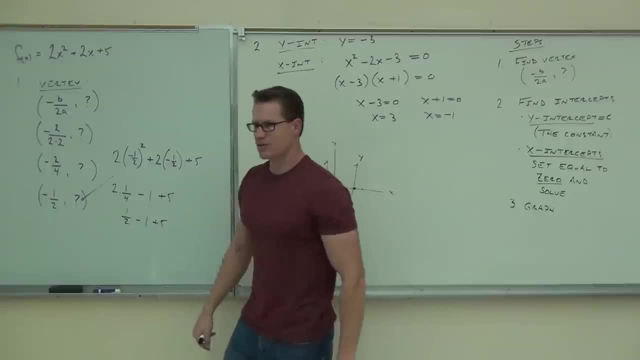 From here on out, we have some basic fractions: 1⁄2 minus 1 is negative 1⁄2.. Okay, Okay, Okay. So this is going to be 1⁄2 plus 5.. If you think about that, that's negative 1⁄2 plus 10⁄2.. 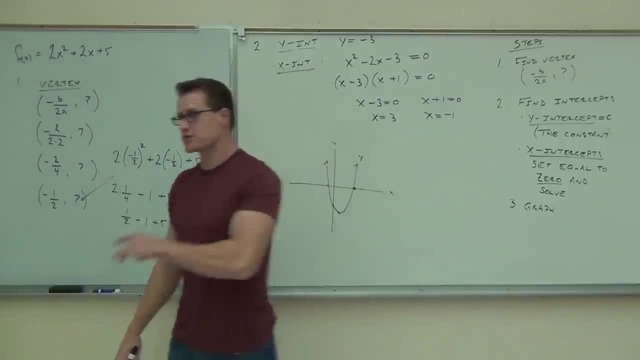 That's going to be 9⁄2.. So this answer is 9⁄2.. Hey, is it okay to? By the way, that's right, right, Okay. So I'm not going to spend a whole lot of time doing fractions with you. 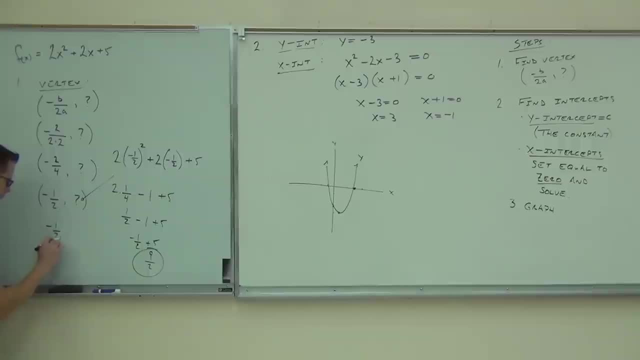 Do you understand the idea? Raise your hand. if you understand the idea about where these numbers are coming from, Raise your hand if you get that. Okay. So I'm going to do this for a second. I'm going to do this for a second. 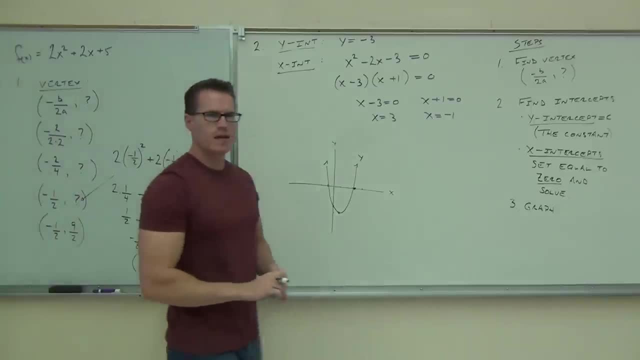 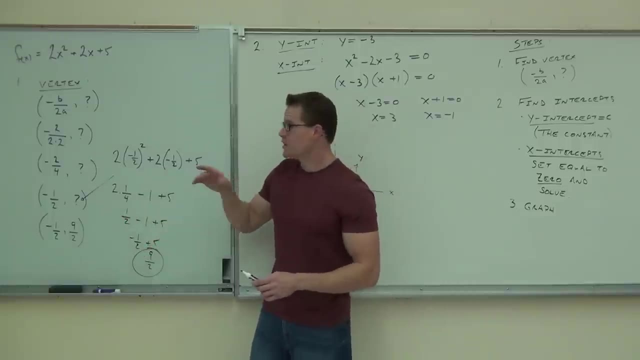 I'm going to do this for a second. Let's see. Let's see, I'm going to do this for a second. Let's see, I'm going to do this for a second. Okay, good, The fraction part. yeah, you're going to have to work on that on your own, okay. 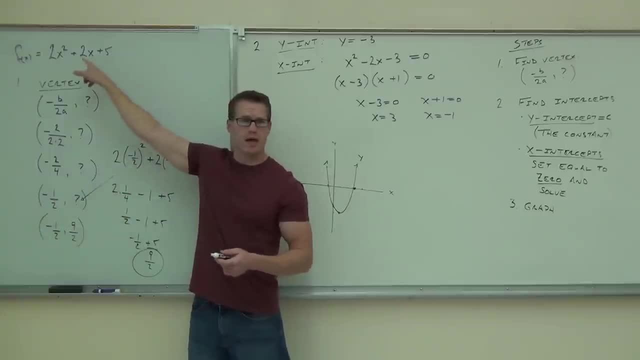 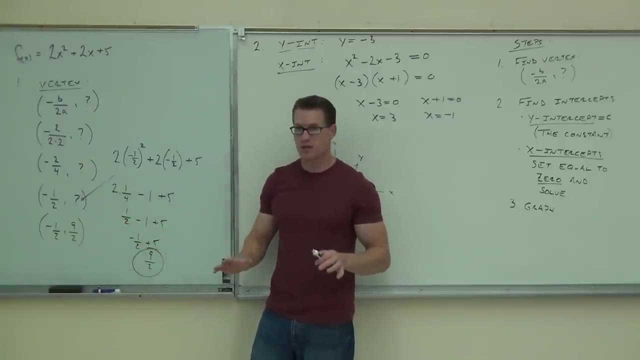 But the idea is you plug in negative 1 half to your function, which you guys already know that That will give you a vertex: yes, You got it or no. If not, then say no, That's okay. But if you got the idea, then sure. 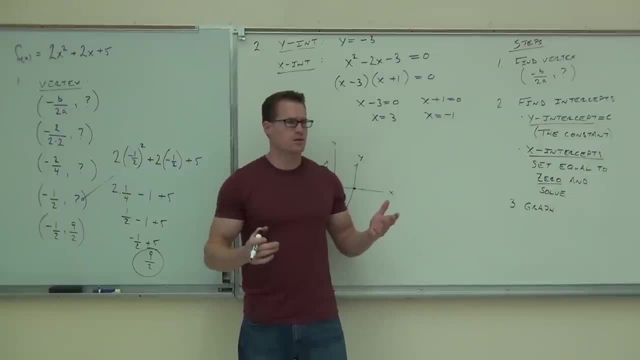 Is it okay to plot a vertex with fractions? Sure, What do you think? Do fractions fit on this graph? Yeah, Yeah, Let's go ahead and continue this. Let's do the easy part. I want you to do that right now. 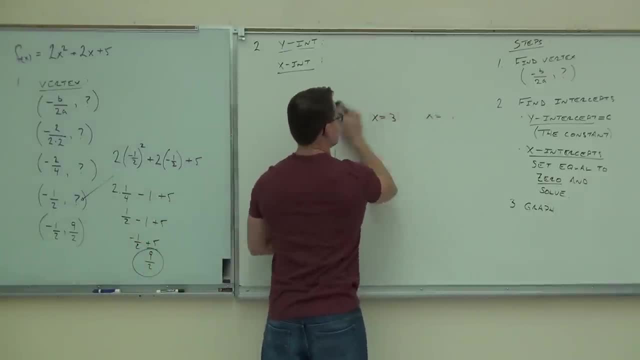 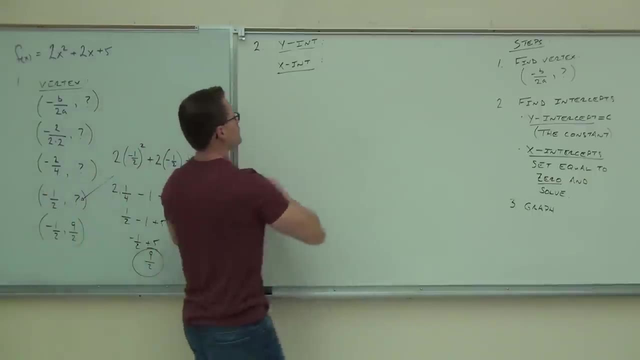 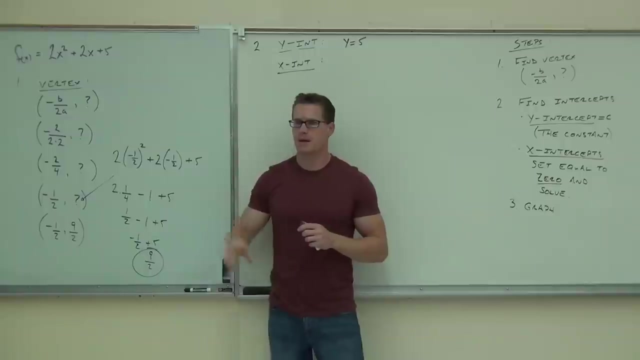 Find me the y-intercept. Hey everybody, What's the y-intercept here? Perfect. Now quick question: This graph is it upward facing or downward facing? Upward, Okay, Is it wide, narrow, normal, Wide? 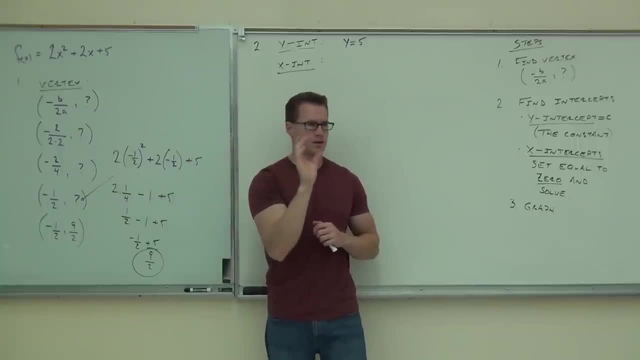 Narrow, A little bit more narrow than normal because of that 2.. Okay, That 2 is making it a little bit skinnier. So the bigger the number, the closer it is. From yesterday: yes, Yep, Same principles as yesterday. 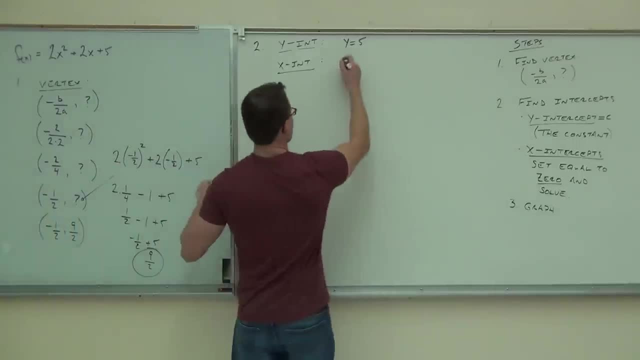 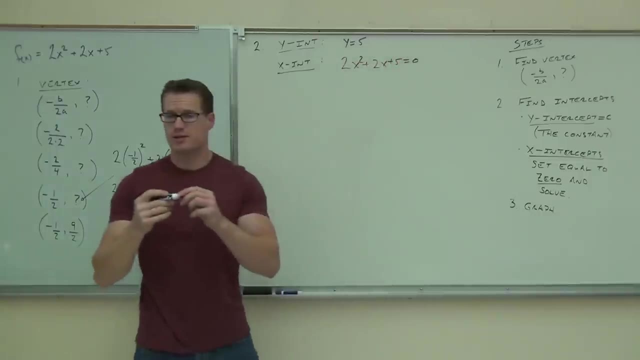 Now the x-intercept. we do the same exact thing. We're going to have the 2x squared plus 2x plus 5 equals 0.. What are you going to do to try to solve that? What's the first thing? 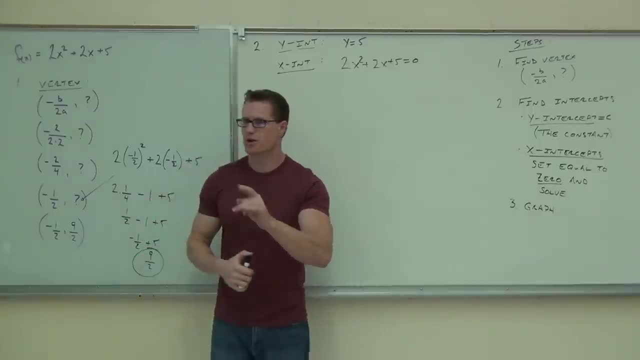 Try to factor. Try to factor. Okay, Go ahead and spend 10 seconds. Try to factor that You should have a 2 on the top and a 10 on the bottom. Okay, You should have a 2 on the bottom. 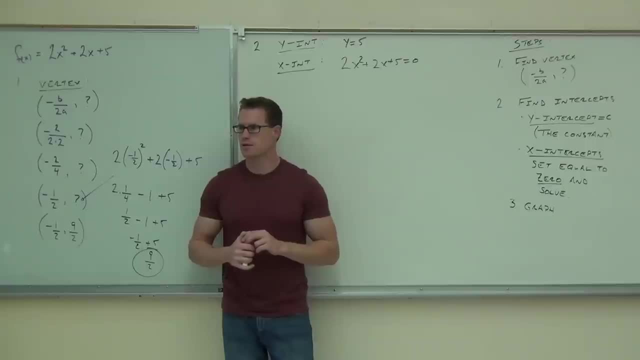 That's about 10 seconds. Have you factored it yet? Anybody, Nobody, Then it's probably not factorable or it's taking too long. anyway, You got it. So what are you going to do now? Okay, Everyone, right now write down your ABC. 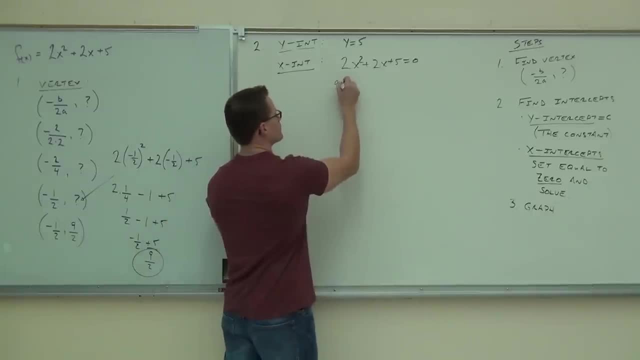 Write down your ABC. What's your A folks 2. What's your B 2. What's your C Prime? What's the quadratic formula? Negative B, plus or minus the square root. Okay, Slow, slow, slow. 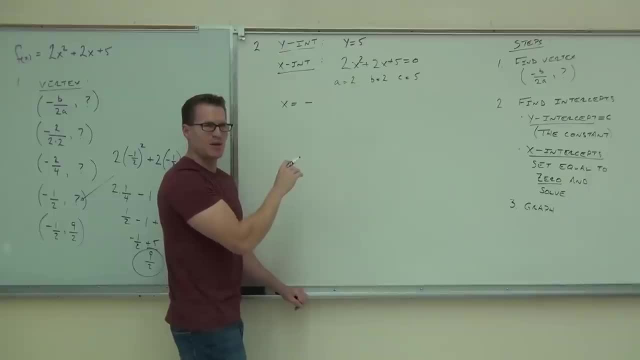 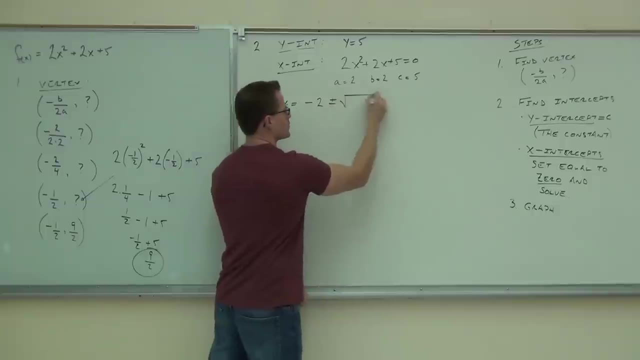 Hang on, I'm writing. You guys are too fast, Too fast for me. What's the quadratic formula? Very slow. What's the first thing? Negative, negative, B, Negative B, Plus or minus the square root. What's inside that? 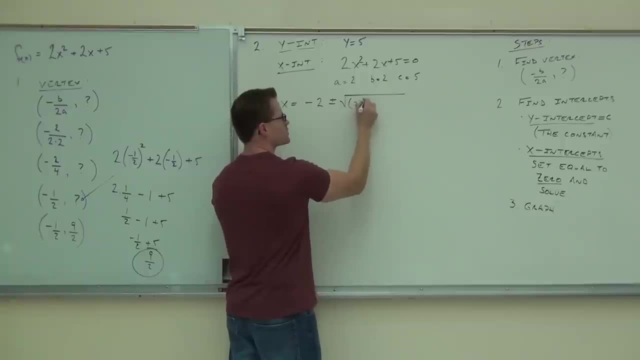 B squared. B squared is first. I always put that in parenthesis just to make sure if I have a negative hanging on to that, I square it. Then I do a Minus 4.. Minus 4.. Okay, That's always going to be there. 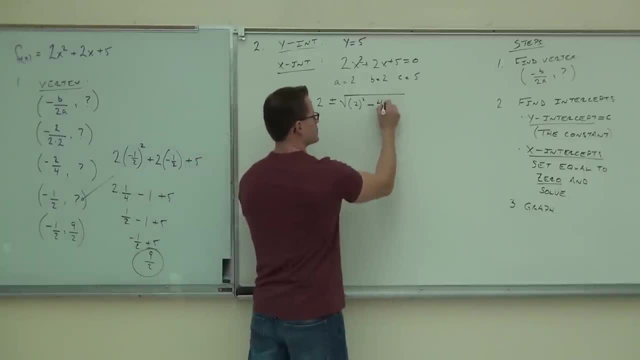 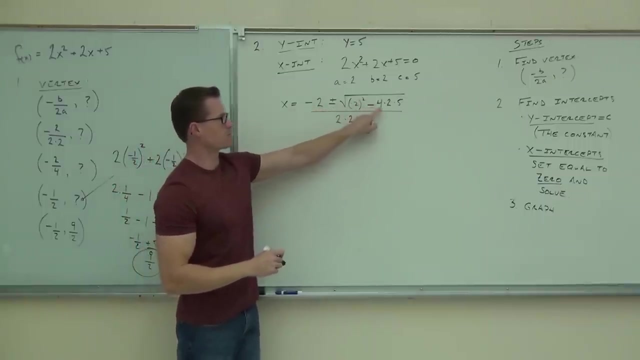 Times. what A Times A? A is 2 in this case. Times C, Which is 5 in this case, All over 2.. 2 times A: 2. 2. Okay, Negative B plus or minus radical B squared minus 4. 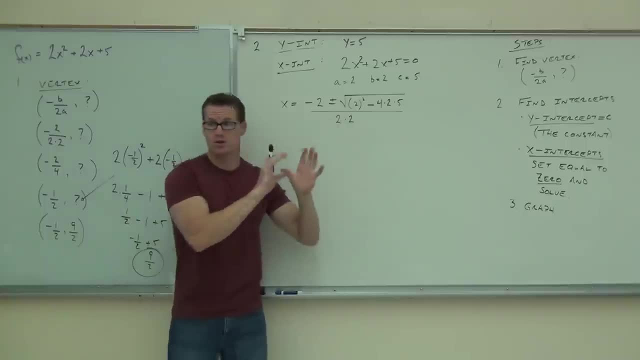 times A times C, all over 2 times A. This should be no surprise right? We've done this a lot in this class, So you guys are okay. You guys are okay with those numbers. Good, Now check this out. Watch what happens here. 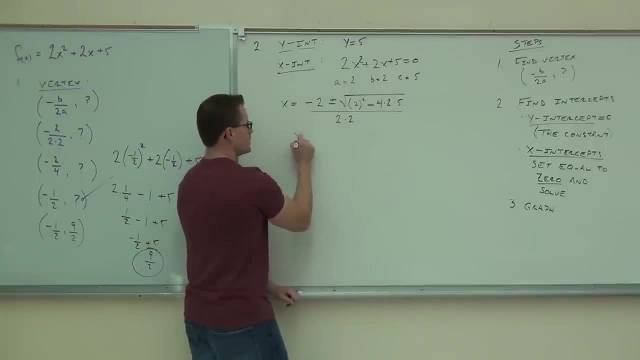 You only have to do one step on this. Two steps maybe. X equals negative 2 plus or minus the square root of 4 minus 40.. Do you see it? Over 4.. What's going to be inside of my radical? 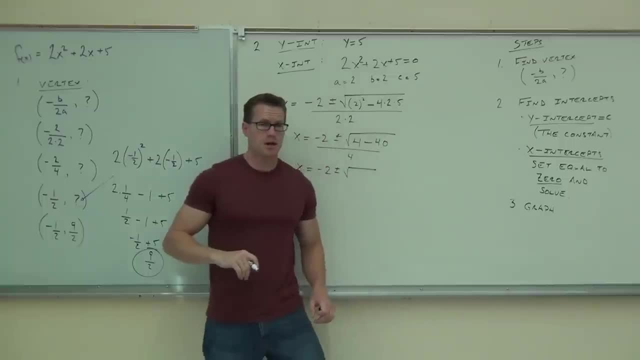 Negative 36.. Wait, 36 or negative 36?? Negative 36.. Is it important to get that sign right? Look at this. Oh my gosh, What is the square root of negative 36? 36. 6i, Not 36i, right? 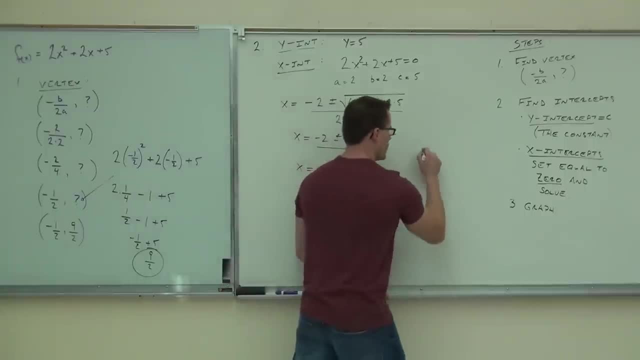 Some of you are giving me that It's 6i. By the way, just a little note for you, If you have the square root of negative 15, some of you are doing this- 15i, It is not 15i. 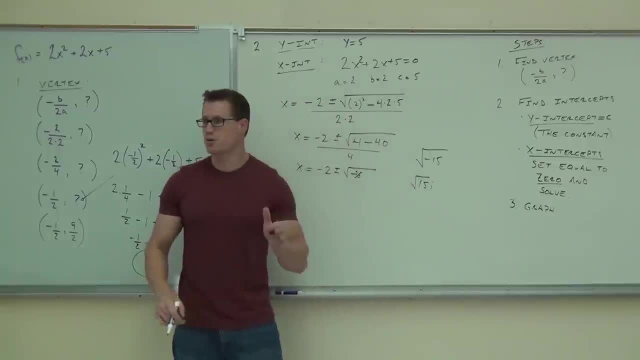 You're forgetting all about this square root that you never took care of. It's a square root of 15.. So you have, i root 15.. Just a little side note for you: A lot of you are doing that right now, So be very careful on that. 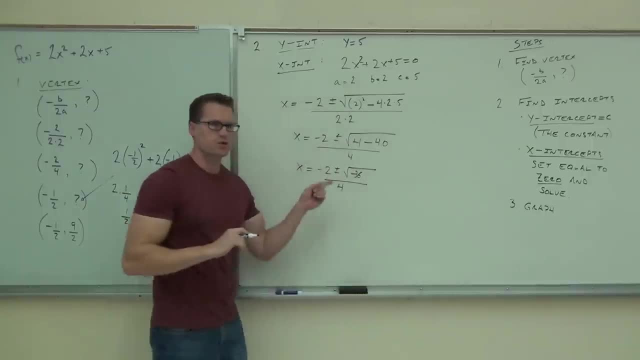 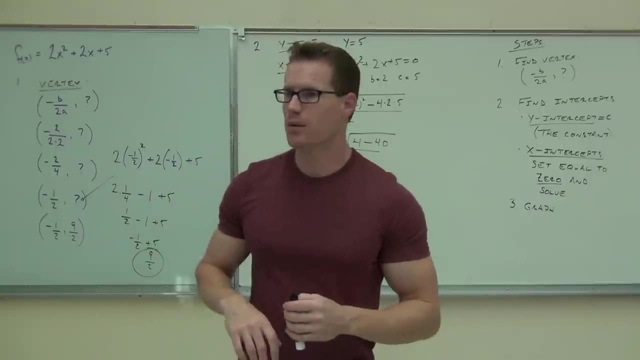 Anyway. so back to here. Is this giving us real solutions or complex solutions? Complex solutions: Hey, If you get a negative inside here, you're going to get a negative Negative Inside your square root. what it means is that your parabola will not cross the x-axis. 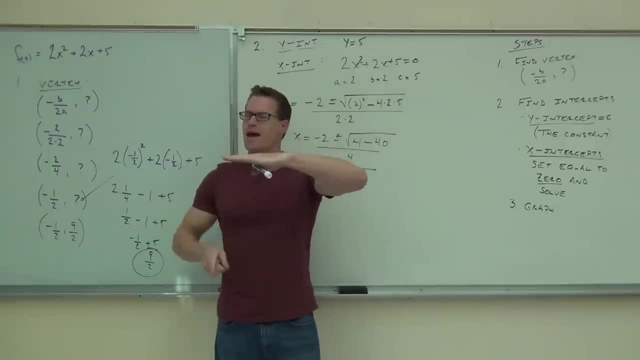 That's all it means. You're either like this or you're like this. Thinking back to our original graph, which one are we? Are we upwards or are we downwards? Upwards? So we're like this. We should be all the way above the x-axis. 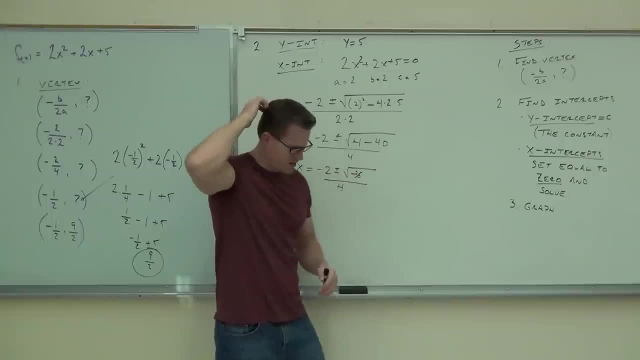 So when you do this and you come up with a negative inside your square root, you go: oh man, did I do it wrong? No, No, you might not have done it wrong at all. You might not cross the x-axis. That's what those complex solutions mean for you. 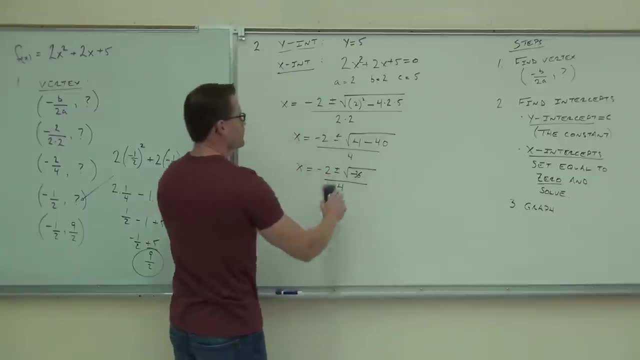 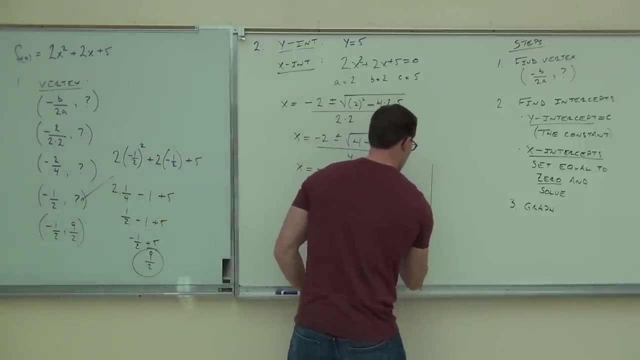 You follow. So no x-intercepts Because of that. This is really just going to have two points that we're going to be able to graph this with. 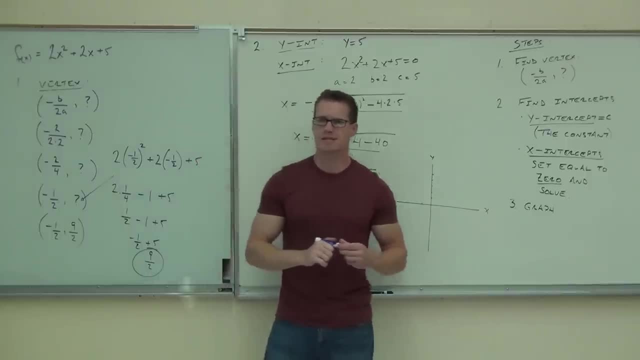 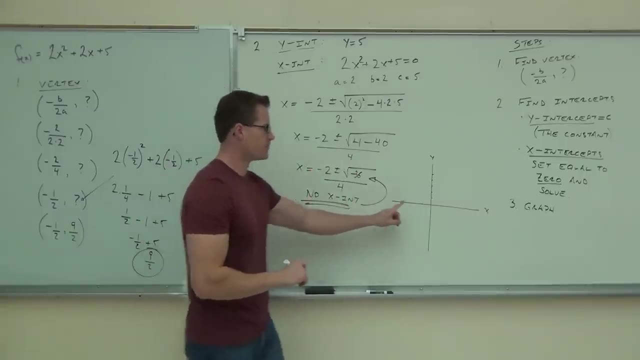 Only two. So the first thing we do is graph our vertex. Our vertex is at one-half, Sorry, negative one-half comma nine-halves. You tell me how to get to negative one-half. Where do I go? Left or right? 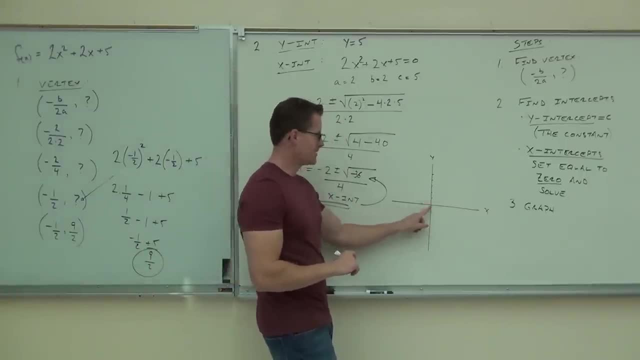 Stop me when I get there. Are you ready? No, just kidding. Stop it Right in the middle. That's negative one-half, Now nine-halves. How much is nine-halves? Translate that to a mixed number, if you'd like. nine halves is four and a half. 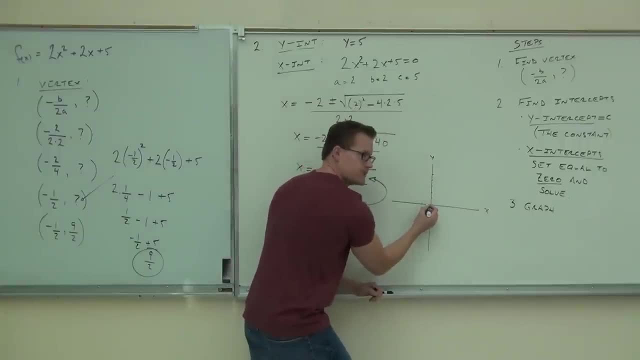 So here you go, watch on the board, we've got negative one half. we've got nine halves. That's one, two, three, four and a half, four and a little bit. Are you okay that? that right? there is my vertex. 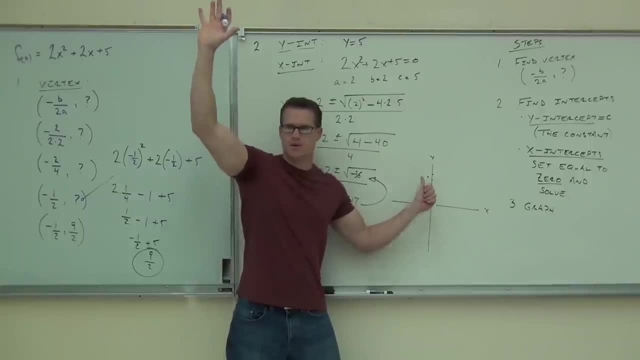 Raise your hand if you are, if you're all right with that. If you're not, raise your hand, I'm assuming you're not okay with it. let's check one more time. Are you okay that the vertex is right there? 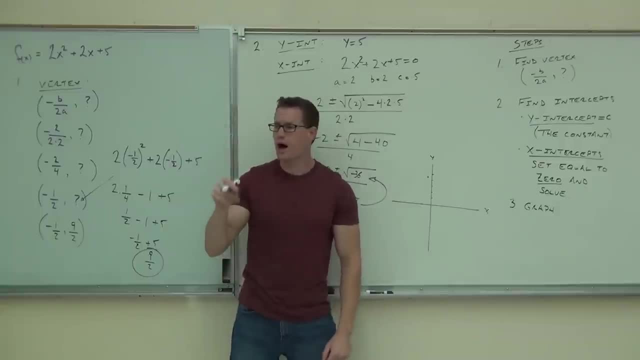 Good, okay, we can plot that thing. Now plot your y intercept. what's your y intercept? Where's five? Pretty darn close, right there, right You with me. That's it, that's all you got. Is this going to have any x intercepts? 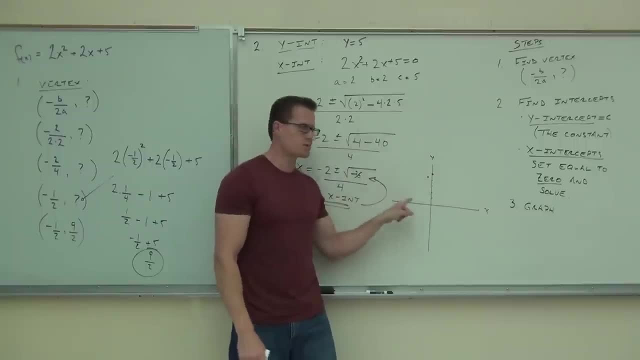 Look at it. this is the vertex and it's going upwards. can it possibly cross this axis? That's why you couldn't find anything here. that's why it didn't exist in real numbers. Okay, How do you graph this? 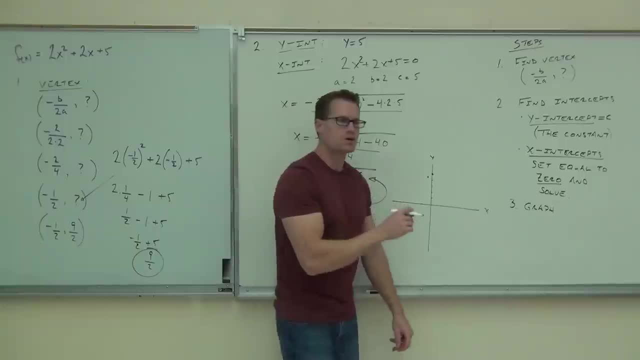 You graph the y side first and then you make it symmetrical, So this should be a more narrow graph. we can see that right here. it's pretty narrow. we're going to graph this up as best we can and then just make it symmetrical on the other. 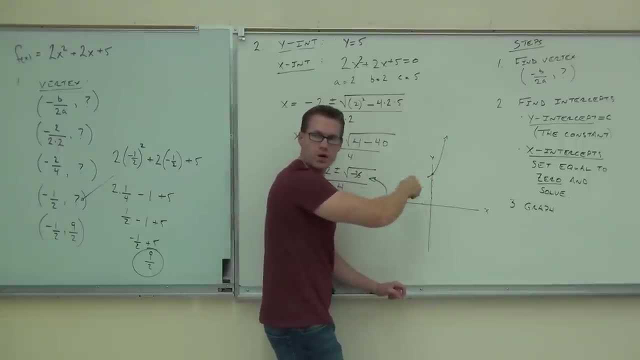 side. There's nothing over here to give us a reference point. that's why you have to use the y side first. So one, two f of x zero. Would you raise your hand if you're okay with that so far? 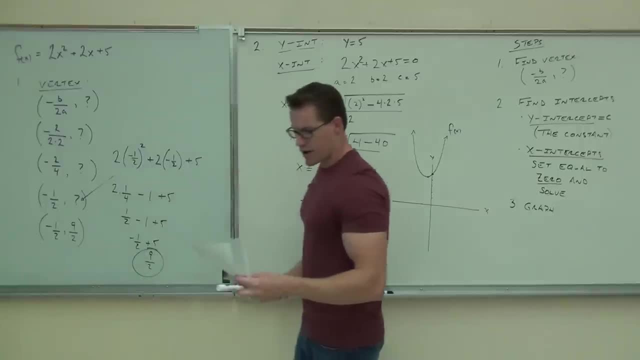 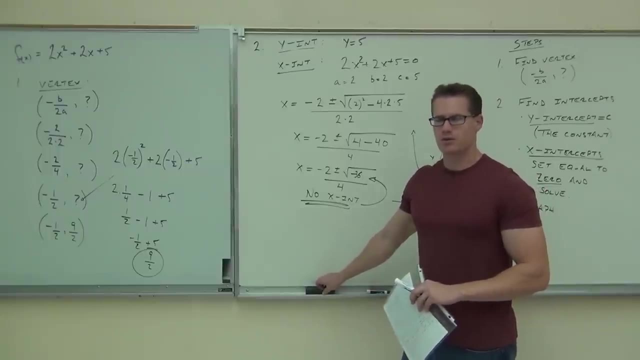 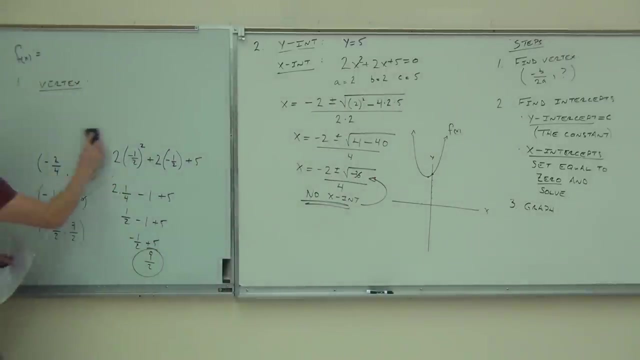 Okay, Good deal, We're going to try one more together, just one more example, and then I'll show you how to find the maximum height of a rocket, which is going to be kind of cool, and we'll be done, Yeah. 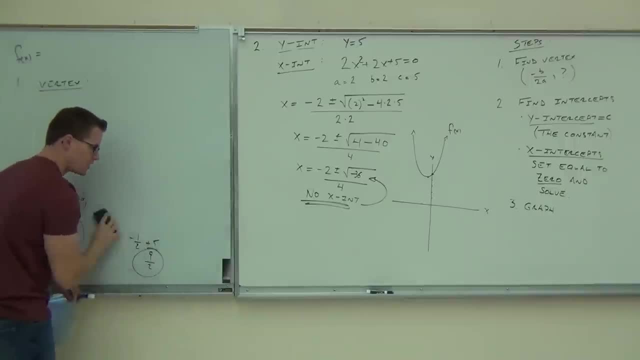 If the square root was positive, then we would be able to have an x-intercept. Absolutely, If the number inside the square root is positive, you're going to be adding and subtracting a real number. That will give you two intercepts. 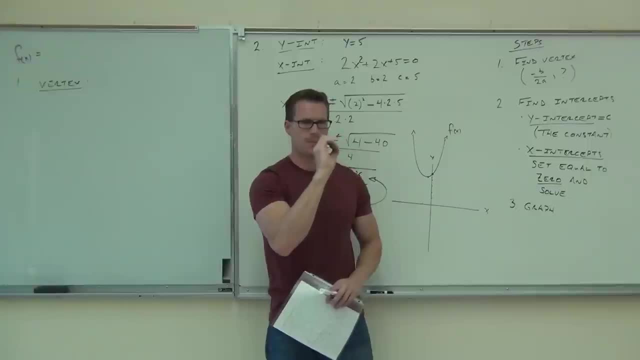 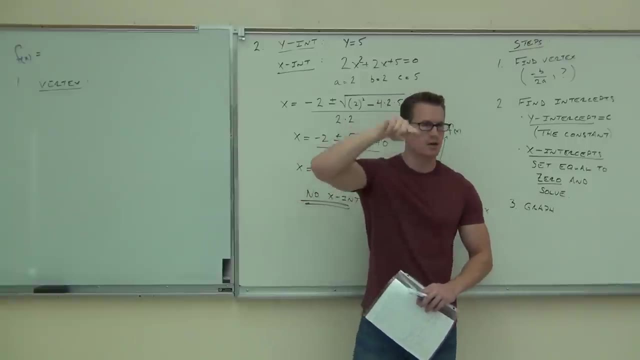 If the number inside the square root is zero, zero, Zero, Zero, Zero, Zero, You're adding and subtracting zero, right? That means you're only going to get one solution. that means you're going to be touching the x-axis. 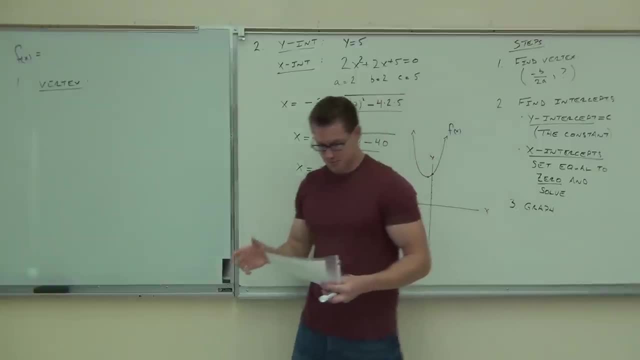 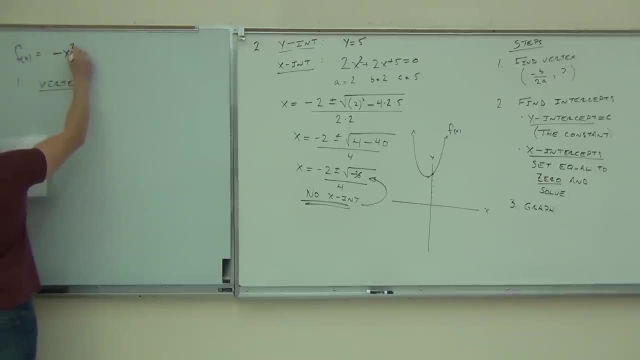 The vertex will be on the x-axis. If you're following me on that one, That's it. Okay, I'm going to have you do most of the work on that. So If you're following me on that one, I want you to find the vertex I'll give you about. 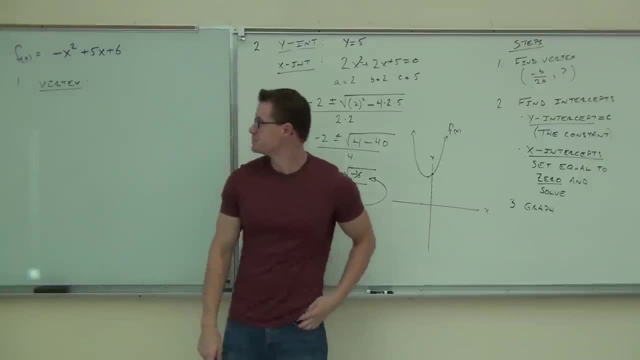 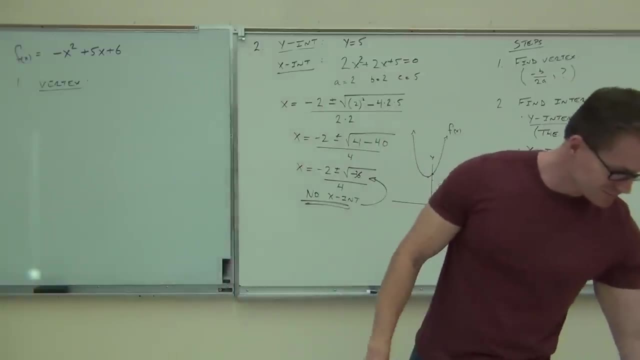 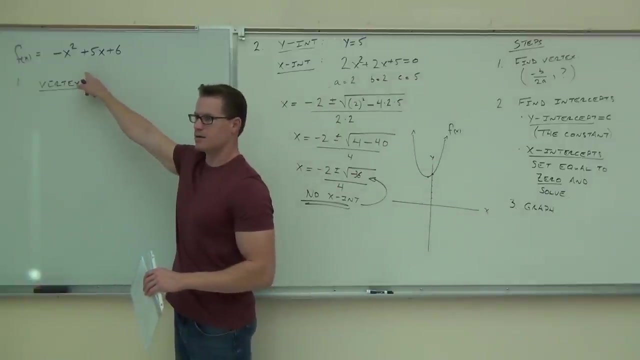 30 seconds. Go for it. This is easier than the last one. Oh wait, No, it's not. No, it's not, but it's good for you. It's harder when they're not even huh, It's harder when they're not even. 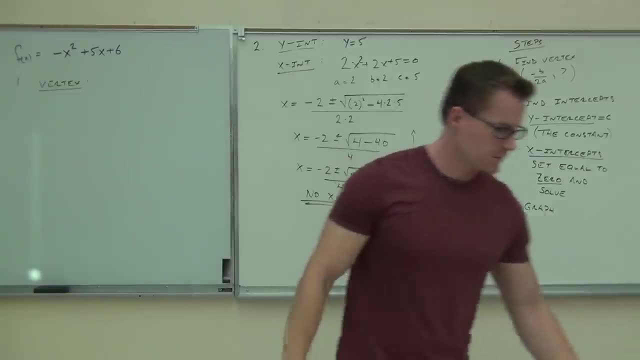 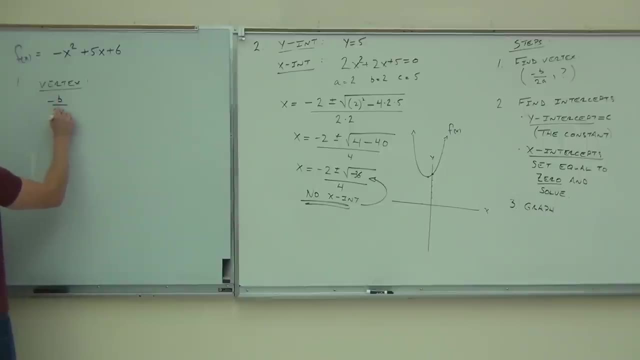 You're going to get a fraction. Okay, Thank you, Have a great day, Bye, Bye, Bye, Bye. Hey, by the way, what is your A here, negative? what's your B? what is your C? are you going? 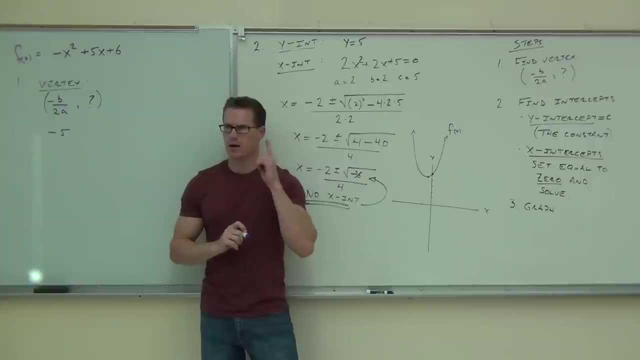 to get an upward or downward facing parabola. keep that in your mind. you're going to get a downward facing parabola. When we plug this into our vertex, you should have negative five over two times negative one. did you see that? did you get that? you get the negative one right comma. some question? 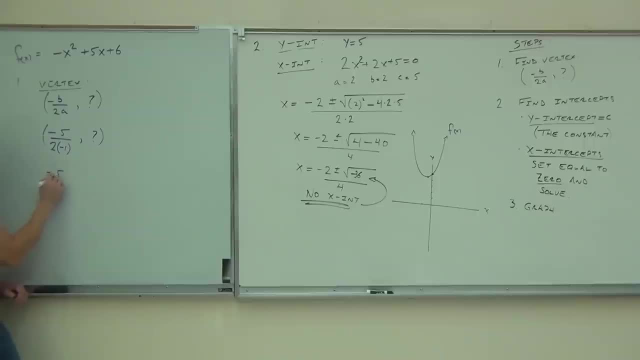 mark because we're not there yet. This is going to be negative five over negative two. how much is negative five over negative two, folks? how much is that positive? five halves, why? because we've got a negative over a negative, so you're going to get five halves. comma question mark. 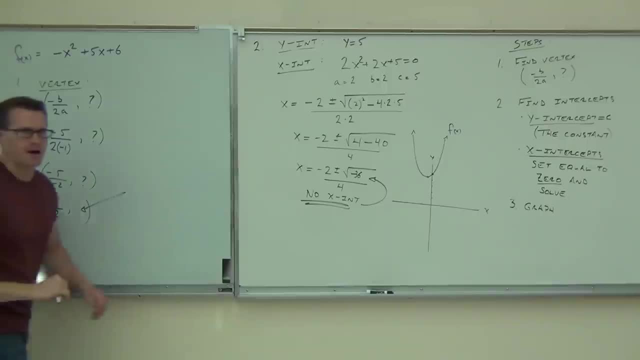 Now what goes in here is what happens when you plug this into our vertex. You plug in five halves. so you've got to be kind of good at plugging in those fractions. I'm going to do this kind of quickly, but do you know where this comes from? what do? 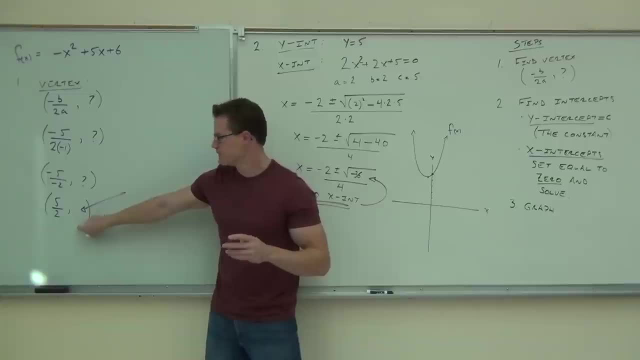 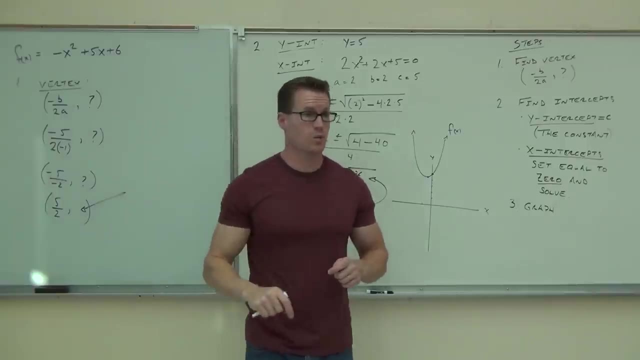 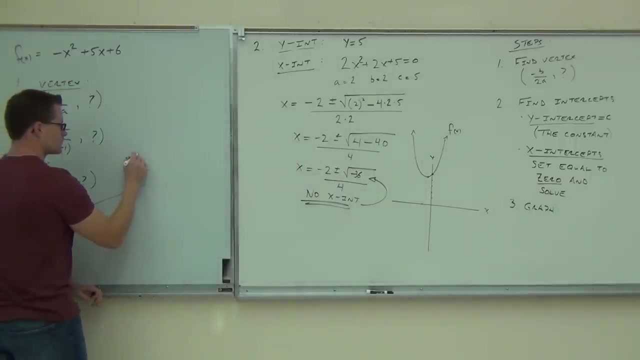 you. what do you? where do you get this again? This one? Yes, Where In the original? So do that now, show me on on your paper, just plug it in, then we're going to do the work together, okay, so take some time, plug that thing in there. 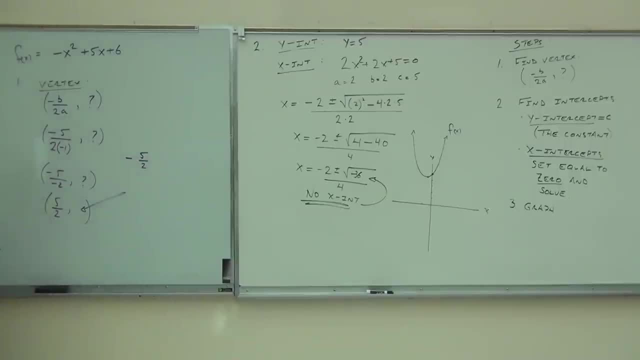 Just one little note here: When you're doing this one- I'm going to show you how to do this- please watch carefully on the board when you're plugging this in- That negative is not being applied to that square. So what happens is you're going to have negative like that, five halves squared. do you see? 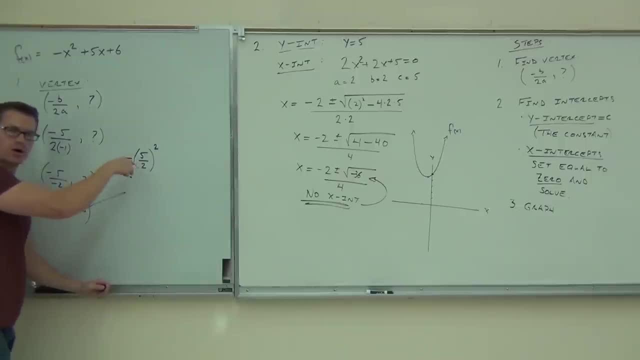 the difference. So this is going to be a negative number when you're done, not a positive, because you're not squaring the negative Plus five times five halves plus six. So we get negative 25 fourths, 25 fourths plus 25 halves plus six. 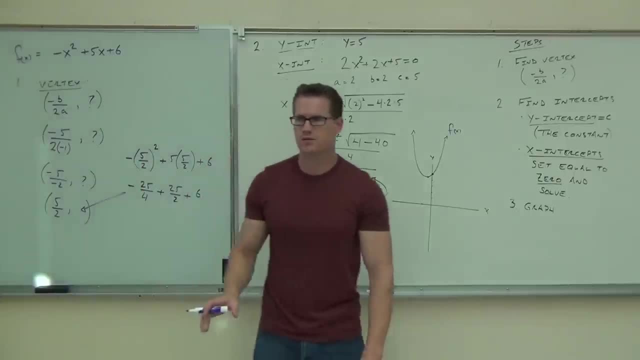 You still okay so far. I'm going quickly through the fractions here, but are you okay on where this comes from? This is the important part. This is it. You can plug this in the calculator and it will do it for you, okay. 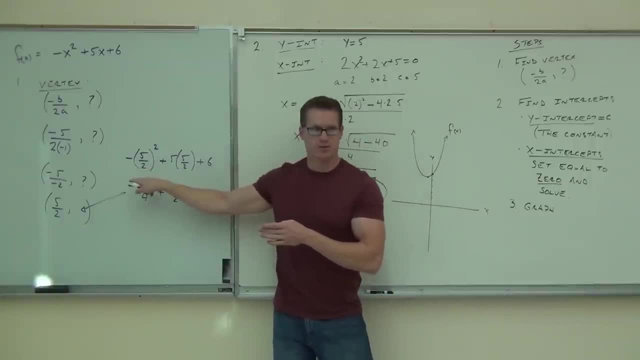 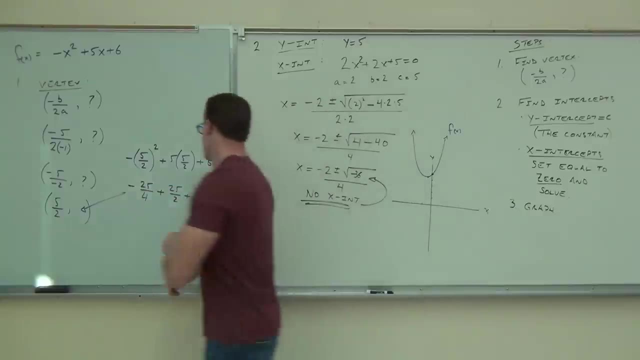 But are you okay on getting exactly this thing? Not sure. if you are, Are you okay that that negative is outside the parentheses? That's very important for you. That would change your whole problem. So, negative 25 fourths plus 25 halves this same thing as 50 fourths. so we're going to. 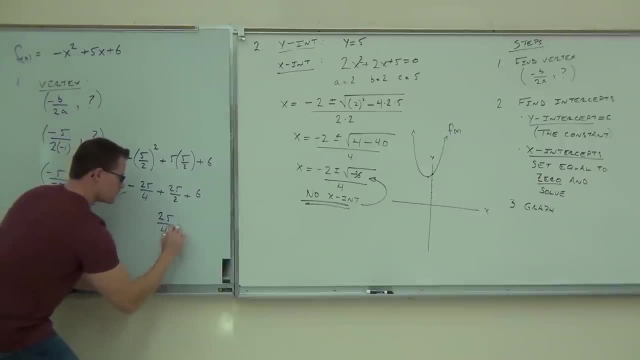 get 25 fourths out of this, plus 6, that's going to be 25 fourths. plus, let's see 24 fourths. that's going to be 49 fourths. That's nasty, So I'm going to double check the work, though I did that pretty quick. 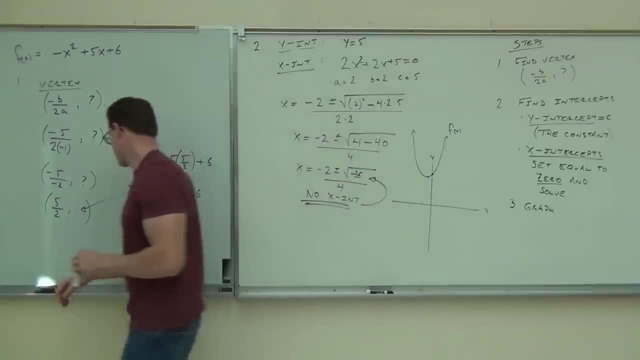 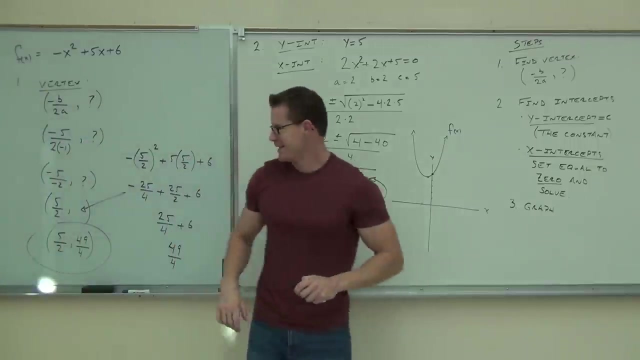 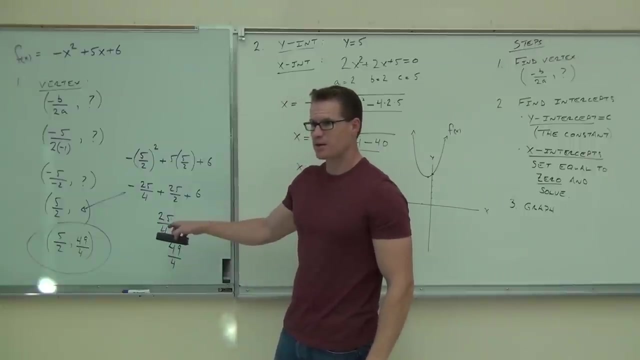 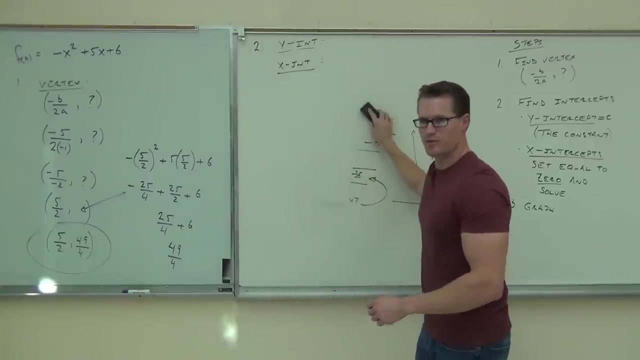 Yes, no, No, Okay. So that's that got a nasty looking vertex. Have you double checked that? did that come out right? Yeah, Good, Good. Have you started to notice that in this problem, the vertex is the hardest part? 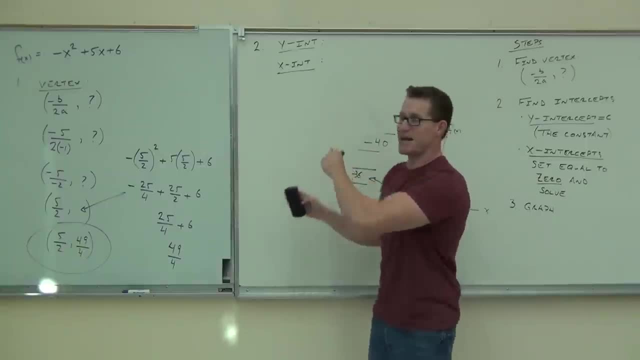 Have you noticed that It's the hardest part, The solvability, The y-intercept, that's the easiest part, that's so nice. The x-intercept's right in the middle. right You have factor and a quadratic, but you know how to do those very well. 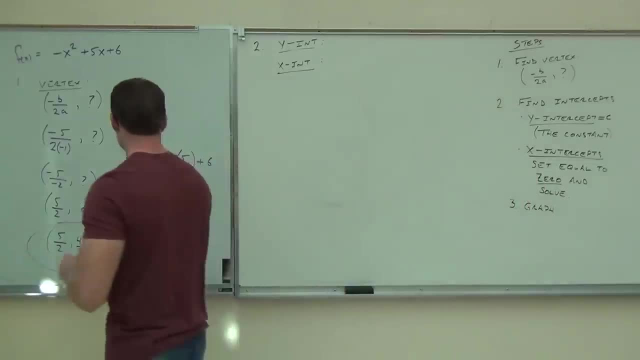 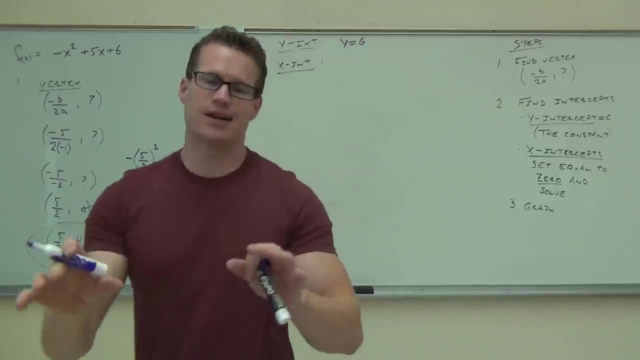 Okay, so that's your vertex. Go ahead and find your y-intercept for me real quick. What is your y-intercept, please? Y equals 6, great, Okay, x-intercept. Now here's the trick to the. not a trick, but here's what you can do with this problem. 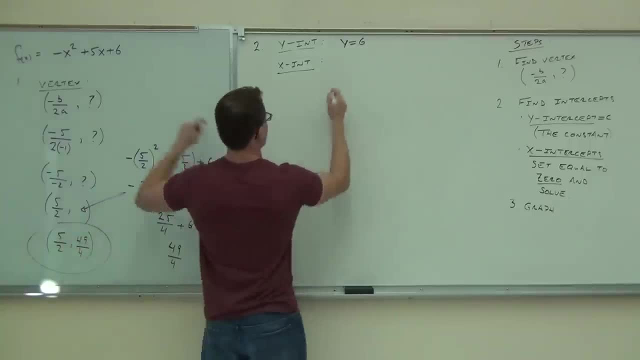 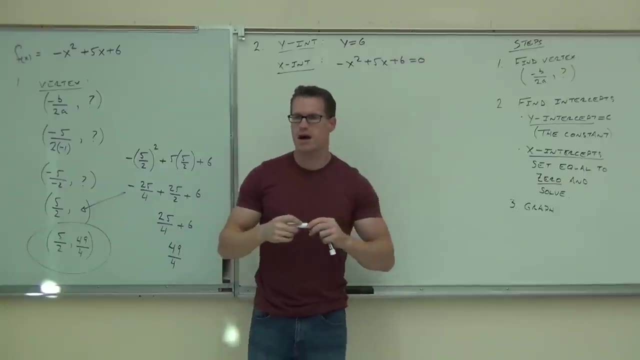 Check it out Please. everyone's eyes should be on the board right now. When you do this problem, you're going to have negative x squared plus 5x plus 6 equals zero. Yes, Now, a lot of you on the second test made a little mistake at this part. 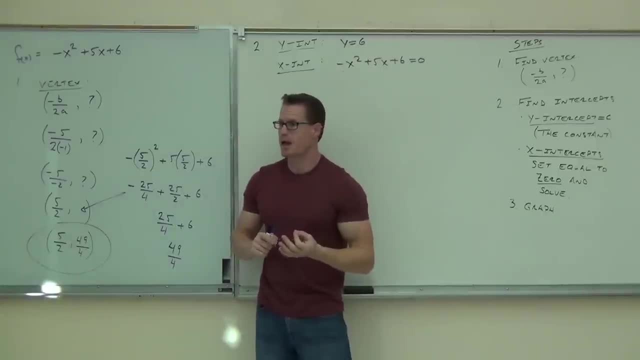 You left it negative and you still tried to factor it, and that's not going to happen. You can't do it. Okay, it's not going to work out correctly for you because you have a something times something. give you a negative, something squared. 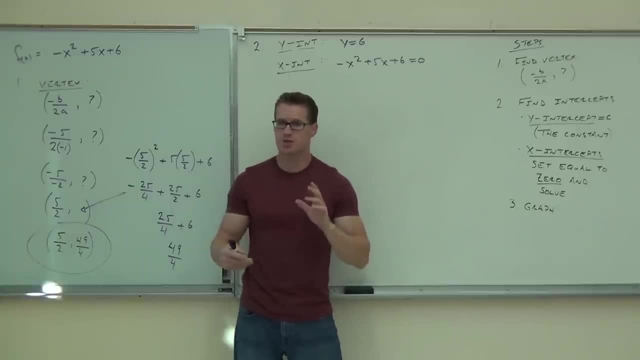 You're not going to be able to factor the way we learned how to factor. You can either choose quadratic formula or you can manipulate this just a little bit. I want you to watch. I want you to watch something here. You agree with me that it's legal to do whatever I want, as long as I do it to both sides of. 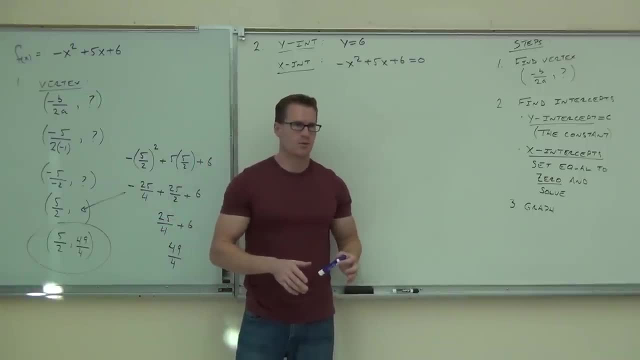 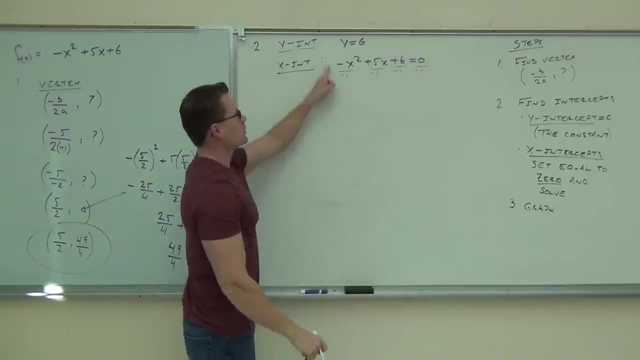 the equation. right Yeah, Divide everything by negative 1.. What that's going to do is change every single sign. Do you see what I'm talking about? Just do that. If I divide everything by negative 1, check it out: negative 1,, negative 1, negative 1.. 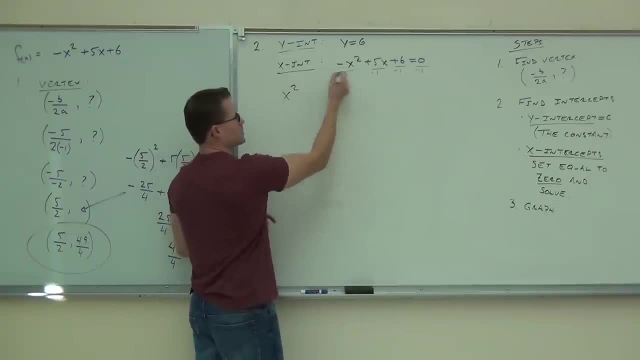 What's this first term going to become? Second term's going to be minus 5x, then minus 6, and I'm still going to have zero, aren't I Do you see it Now? here's why we do these steps in order. 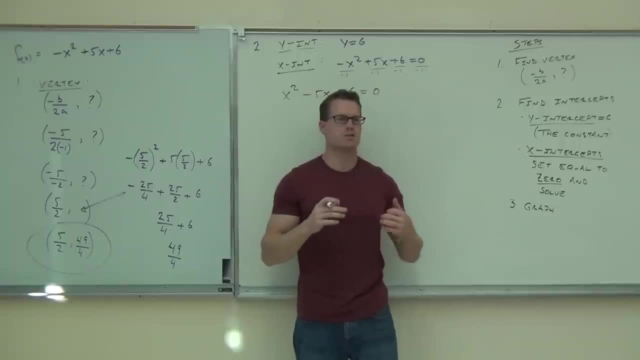 If you didn't believe me, you're like: ah, Mr Leonard's just full of smoke. I don't have to do this in order, Check it out. If you try to do this first and you try to find the vertex from this one, it will be. 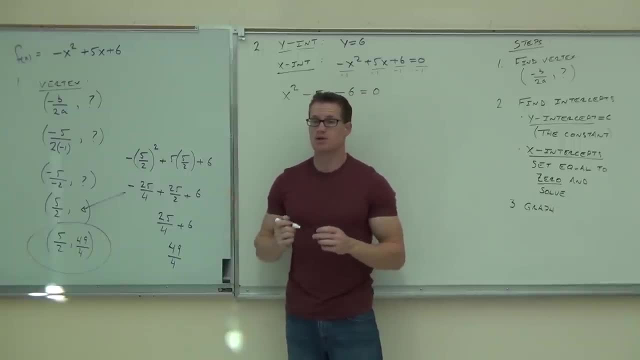 completely different than that. Okay, It's not going to be the same thing. That's why you have to find the vertex from your original, You have to find your y-intercept from the original. before you do this whole thing, before you start changing signs. 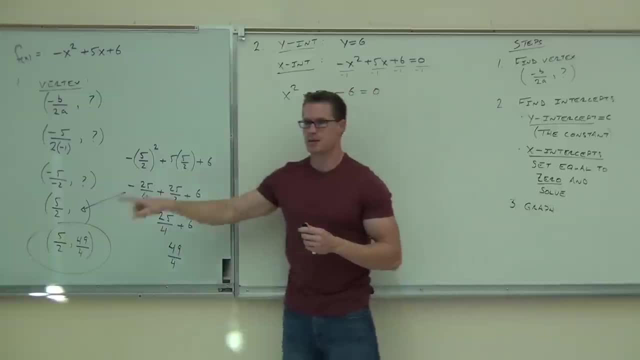 Do you get it now? You've got to do that Now. this is kind of a nice little trick. I'm going to show you how to do it. I'm going to show you how to do it. We can do x minus 6, x plus 1.. 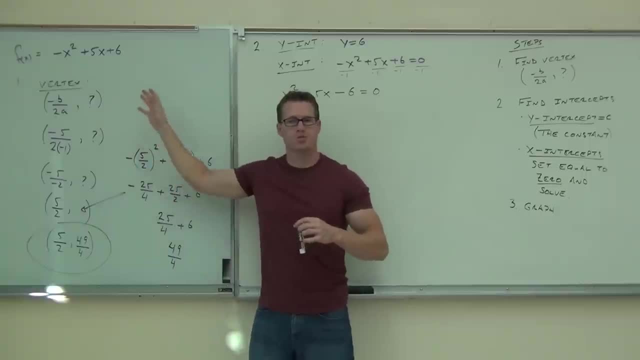 We can do: x minus 6 equals 0.. x plus 1 equals 0.. We can do x equals 6,. x plus 7 equals 0.. We can do 8,, we can do 6,, we can do 10.. 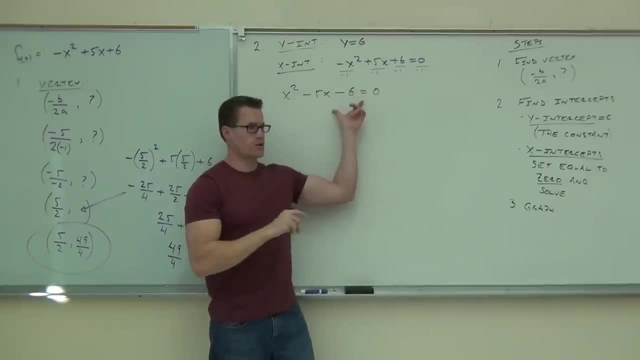 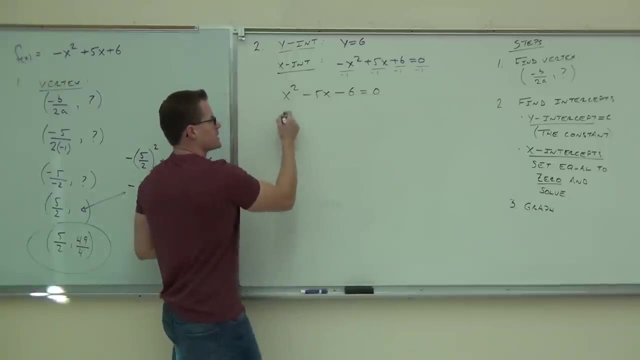 Now let's put these in order. You can do it in space, you can do it in size, You can do it in number, Let's do it in size. These go separate. Whatever you do is going to be exactly the same value. 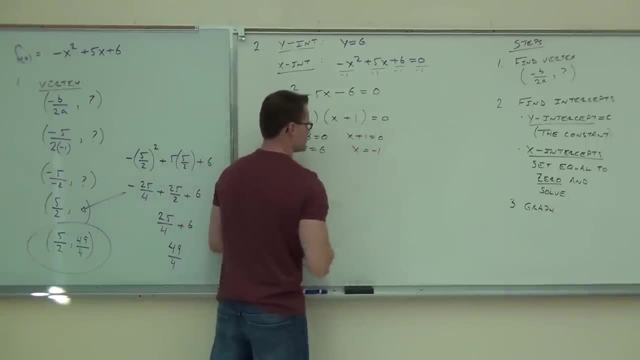 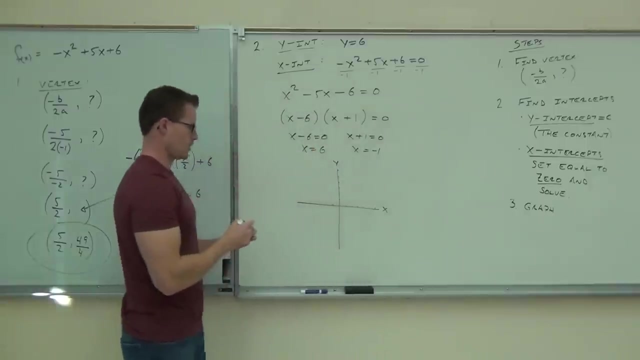 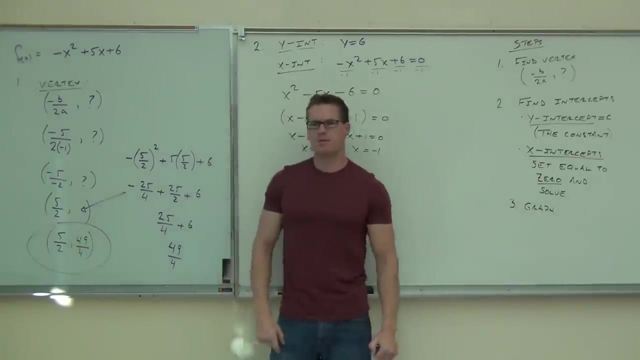 Little things we want to do is going to modify them. x and x equals negative one. Let's see. Oh my well, let's plot this thing. Can you tell me please, how much is five halves as a mixed number Two and a half? 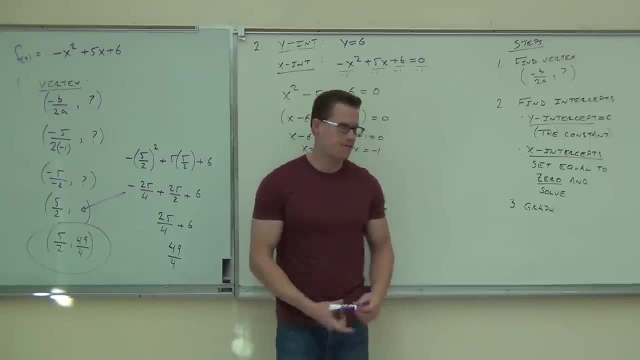 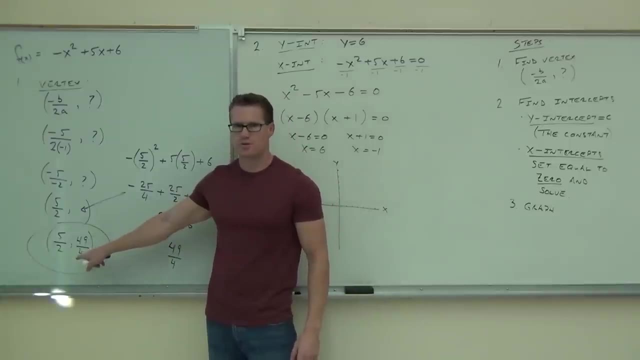 Two and a half. two and a half on the x, You with me Two and a half on the x, So we're two and a half. we're right there. How much is this as a mixed number? 12 and a quarter. 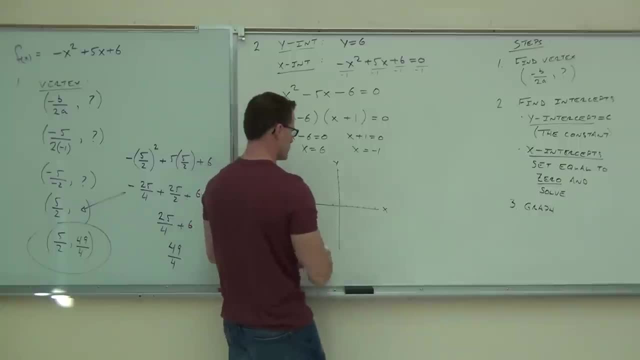 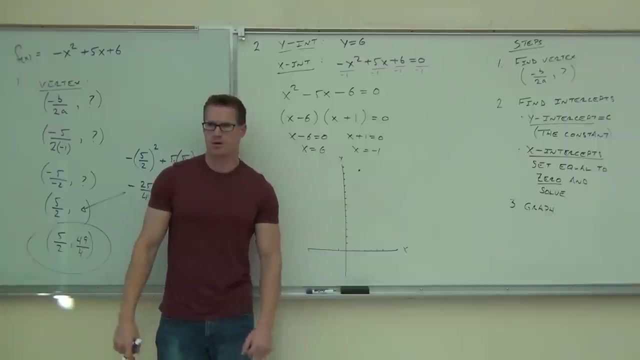 12 and a quarter, That's way up there. shoot Six. ah, I had to redraw my graph. Okay, Okay, So two and a half, 12 and a quarter, That's way up there. You okay with where the vertex is. 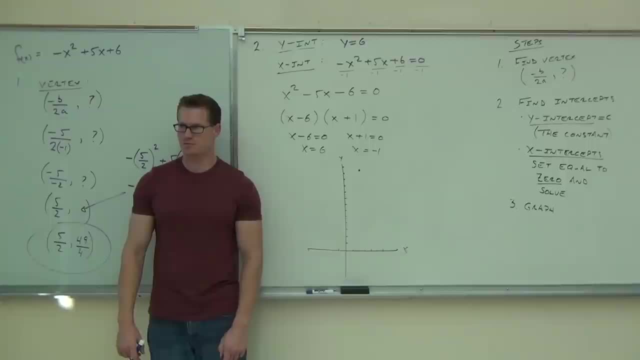 Yes, Pretty close. Two and a half, 12 and a quarter Mixed numbers. if you want, Do your y-intercept. now, where's your y-intercept? Negative six, Six, six is up here: One, two, three, four, five, six. 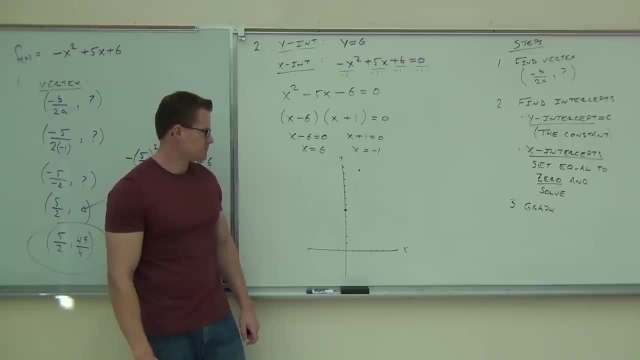 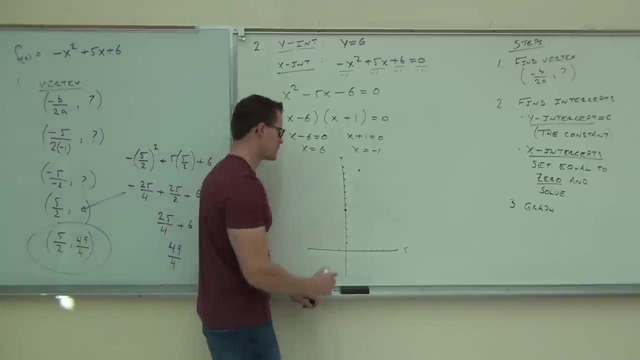 Where's your x-intercept at Negative one, negative six? Go ahead and plot them. now. My y-axis is a little curved, you noticed? Oops, Are you all right with these points, where these are coming from? I mean, yeah, you got some nasty fractions, but honestly, this is math C. You should be. 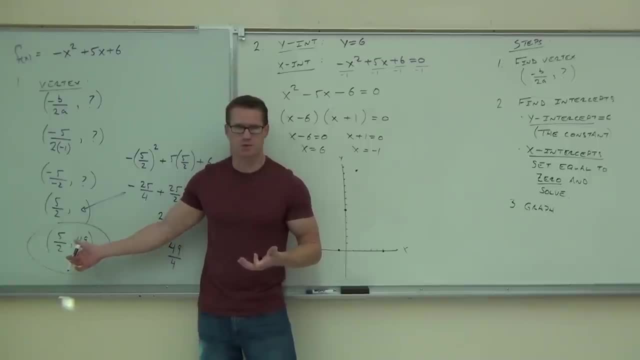 rock solid on fractions. This is a long time ago that you were doing this stuff. you should be rock solid on it. So if you're not, if you're going, where's he getting? five halves and 49 over four? Review your fractions. 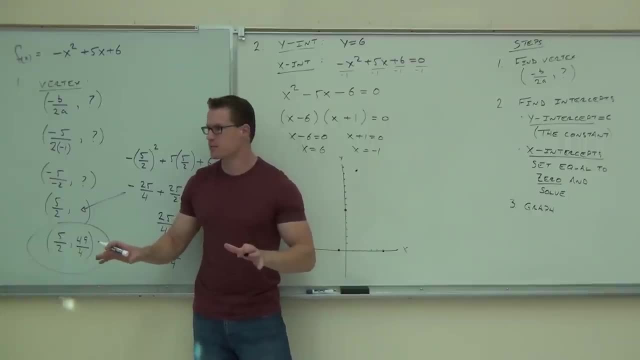 If you don't know how to graph it, review your fractions. That's important. You have to be there. There's no excuse for you to be missing problems because of fractions at this point in your math career. There's no excuse for that. 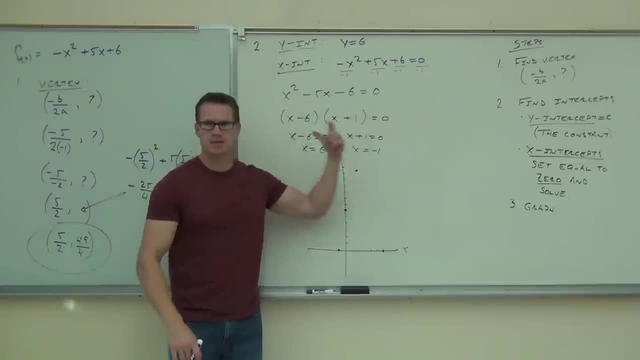 So be rock solid on your fractions Now. this stuff is easy. This is the easiest stuff we've done. We've done this since before chapter seven, So you need to be able to get the six. you need to be able to get these intercepts. 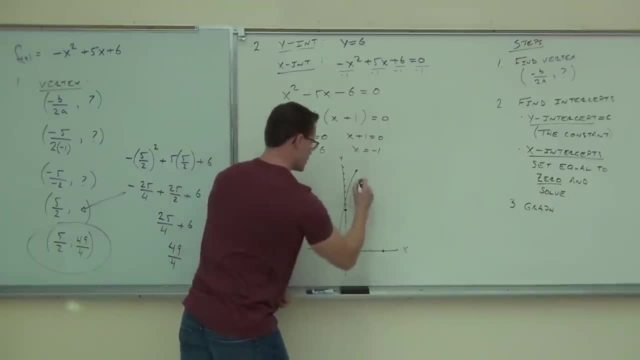 We plot the y-axis first. That's a little off. Plot the other side next. It's hard. They're big graphs. Let's leave one of those here. Hey, it's downward facing, like we thought it was supposed to be. 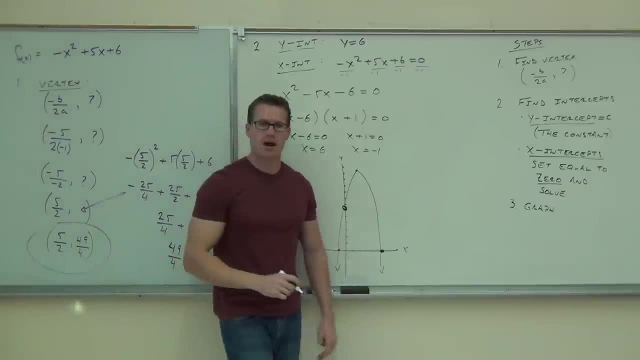 It's normal, shaped like we thought it was supposed to be. That's it. That's our graph. How many people feel okay with this? so far, Okay, good. So the two key points about this particular problem were: make sure you know how to deal. 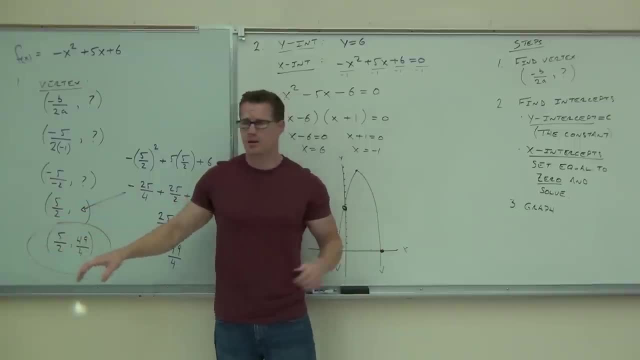 with fractions. You're going to get some fractions, Okay, Yeah, they're a little tough, They're a little tough, but also make sure that you're doing these in the correct order. Find your vertex first, then find your y intercept. 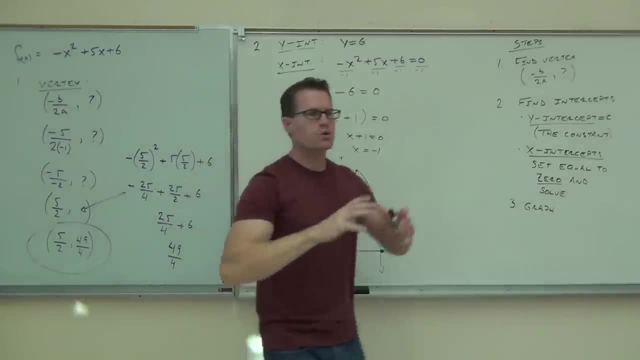 And if you have a negative? if you have a negative, go ahead and find your y intercept. Don't do anything until you switch signs right here. Don't factor it like this. That's ridiculous, You can't even do it. Don't use quadratic formula if you can factor it. 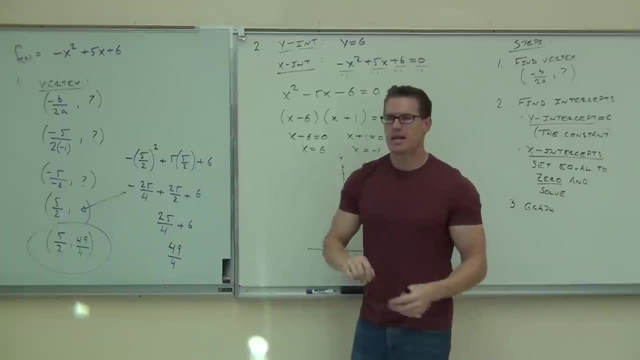 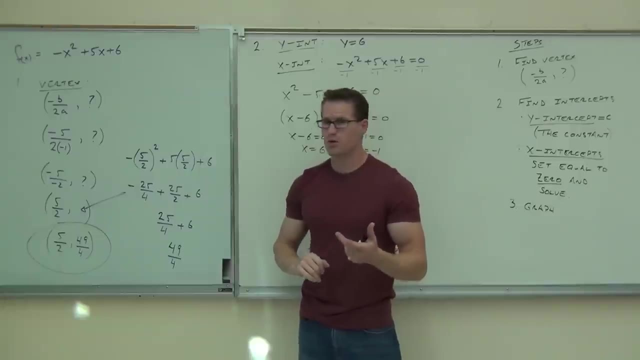 Try changing those signs first and then factor it. Even if you change the signs and you can't factor it, quadratic formula will still work out exactly the same. That's what's nice about it. Quadratic formula doesn't care which way you're going. 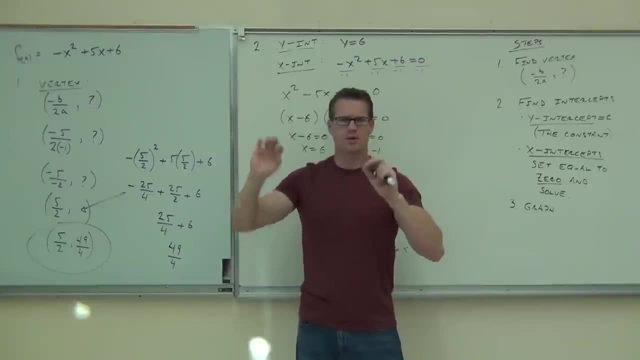 It'll still find you the same exact intercepts. How many people understood what we talked about so far? Good, Okay, Let's do a couple little pieces of information to help you out on some of your homework problems. Some of your homework problems have to do with, like, the height of a rocket. 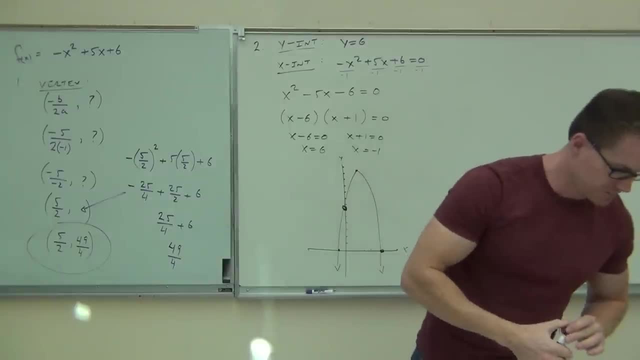 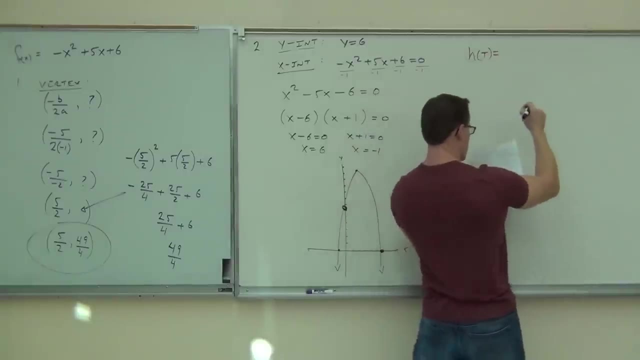 How can you find out the maximum height of a rocket? So, for instance, let's say that you have this: This is the height according to time, Height time, And it's based on seconds. So this right here. hey, what happens if t equals zero? 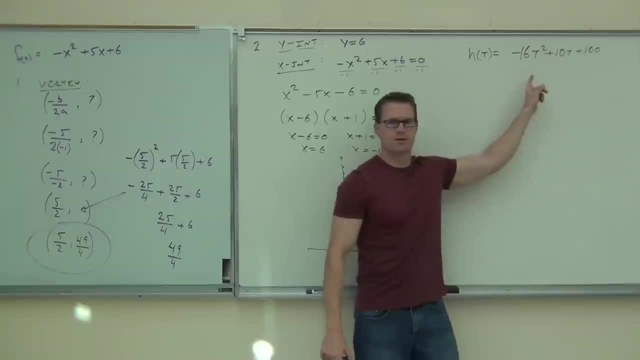 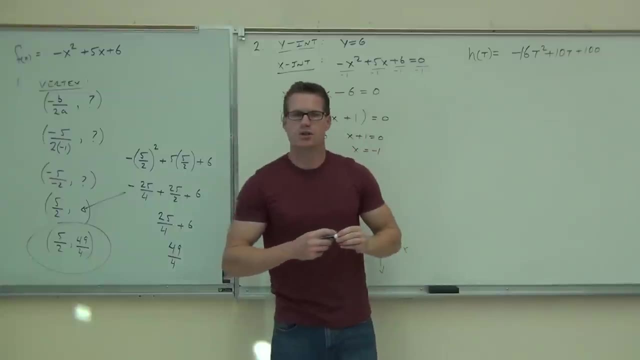 Can you tell me that? What happens if t equals zero? How high are we Zero? No, not zero, We're a hundred. Do you see that A hundred doesn't go away? This person launched a rocket off a cliff. 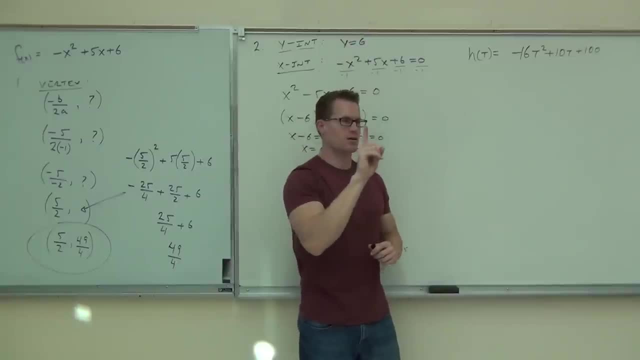 It's freaking awesome. So this guy launches a rocket straight up off a cliff and it's going to go up and it's going to come down right past the cliff. You get me, And the height is given by the time, in seconds. So at zero seconds it's at a hundred feet up on a cliff. 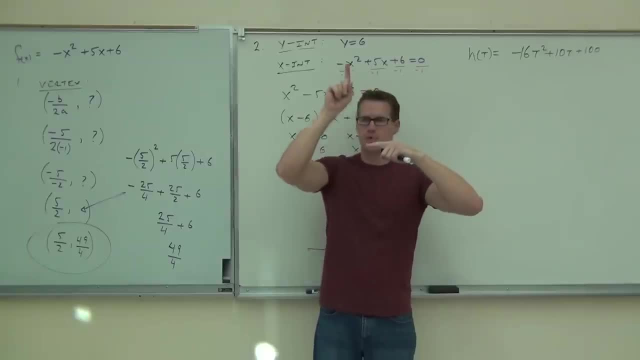 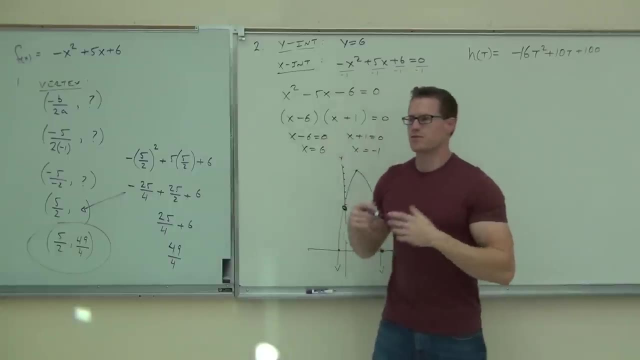 After one second it's going to be a little bit higher and then at some point it's going to max out right. At some point it's going to hit the ground. Here's how you figure all that out. Have you noticed that the vertex is the highest point of a parabola? 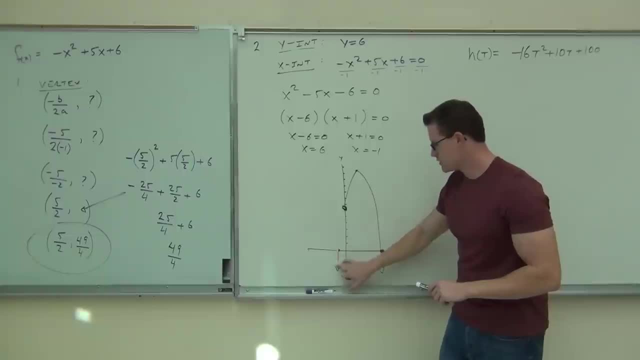 Here's pretty much what this graph looks like. The guy starts at a hundred feet, So he's starting up here. There's no left side, There's no negative time. Guy starts up here, he goes and he hits somebody. whatever, it is right. 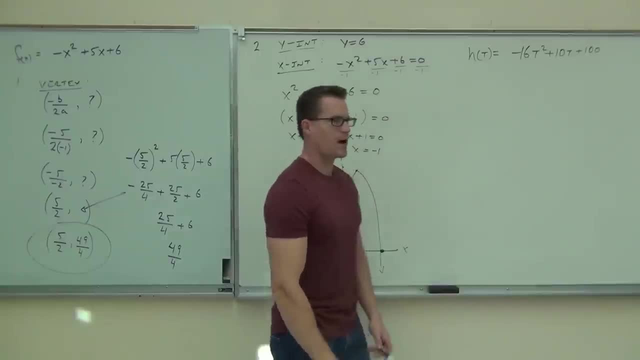 That's like military science or whatever. So he's going to hit somebody. So the height of the rocket initially is given by a hundred feet, Whatever the constant is. that tells you how high you started. Secondly, the maximum height is given by your vertex. 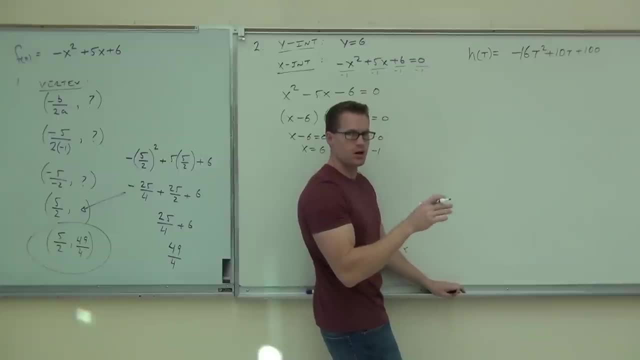 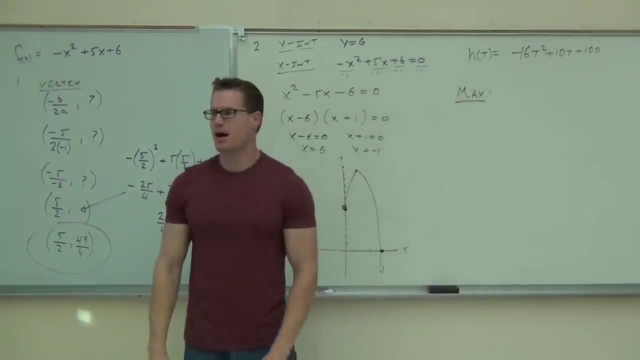 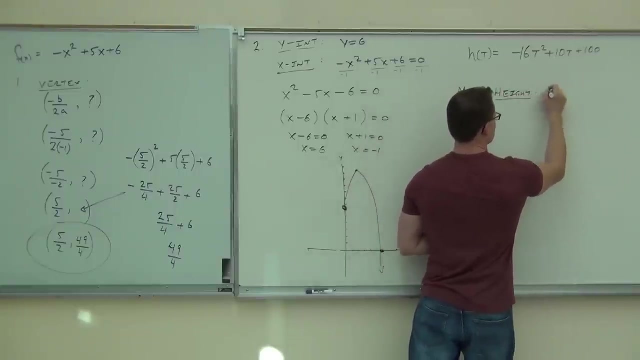 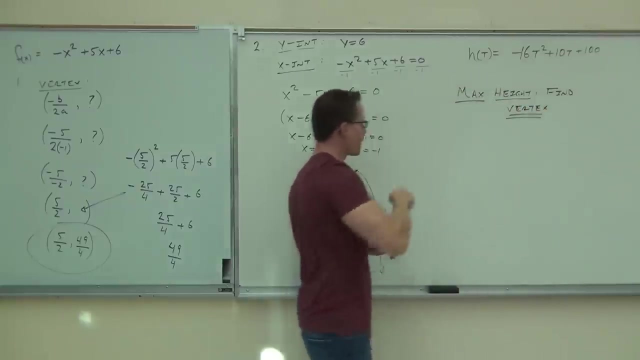 So they ask you: at what point will this rocket attain maximum height? Maximum height in any instance for a parabola is given by the vertex. So for maximum height, find the vertex. I'm not going to go through that with you. the negative b over 2a, you can find the vertex. 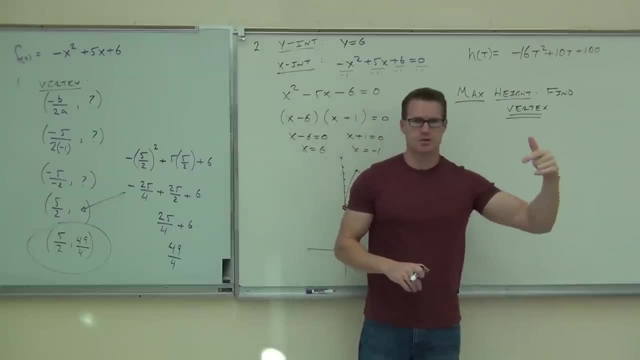 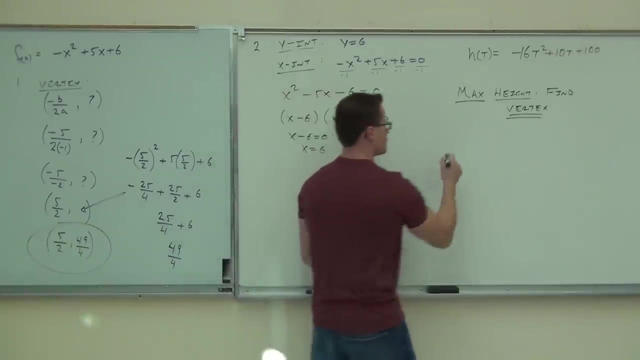 yourself. The x will be the time, the y will be the height. So you're going to get some time comma, some height. Did you follow me on that? Now, if they ask you when will it hit the ground, The answer is gonna be the time and the height. 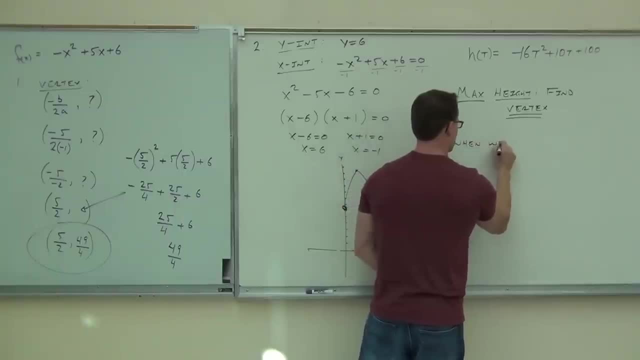 So you're going to have some time. comma, some height. Did you follow me on that? Okay. Now if they ask you when will it hit the ground? Well, the answer would be when the rocket hits the ground And you can find the vertex on the top. 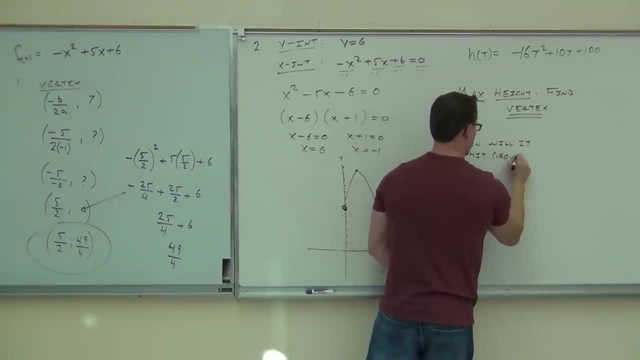 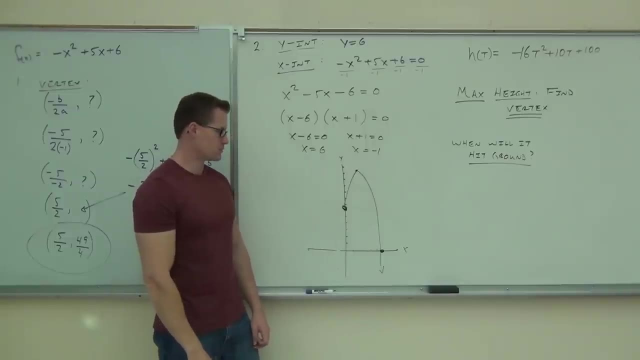 That's right, Or when will it land? Let's look at that. When does the rocket hit the ground? Whenever it hits the x-axis. Whenever it hits the x-axis- right, That's the ground. Now, is it going to hit the ground this way? 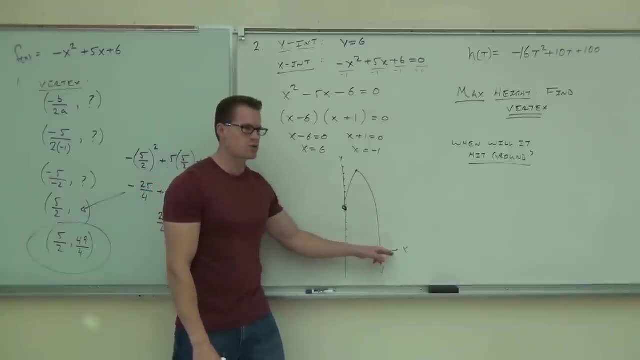 No, that's negative time. So, on your parabola, sure you're going to come up with two, two- I'm sorry- intercepts. One of them very well could be zero, in which case it would be starting on the ground level. 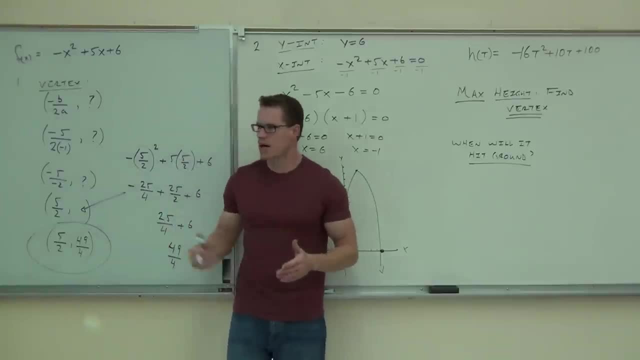 If it's not, if it's negative, of course you're not going to take that, because you can't go backwards in time, but you can go forward. So you're going to look for your positive x-intercept. That's going to be the time at which you hit the ground.